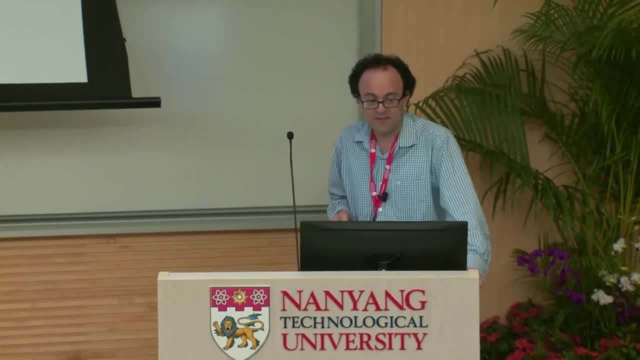 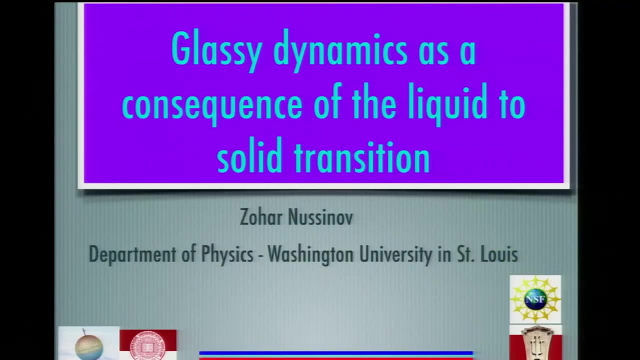 which is very, very different from conventional melting, in which you have topological defects which actually can, of course, induce melting. to actually try to relate it to, basically to say that the glass transition or more precisely, the onset of glass dynamics might 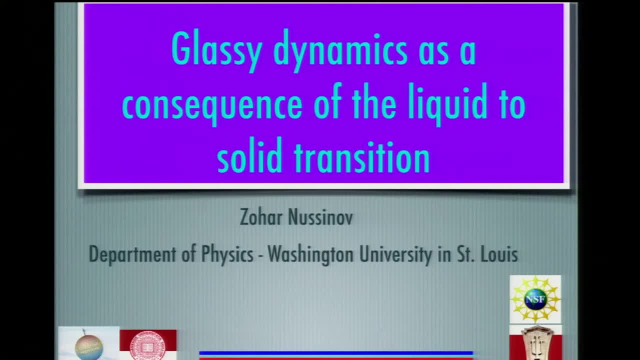 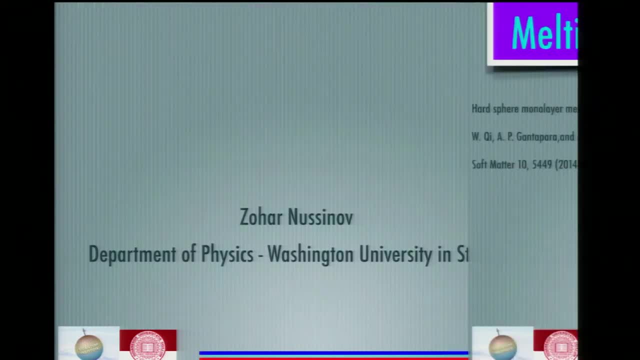 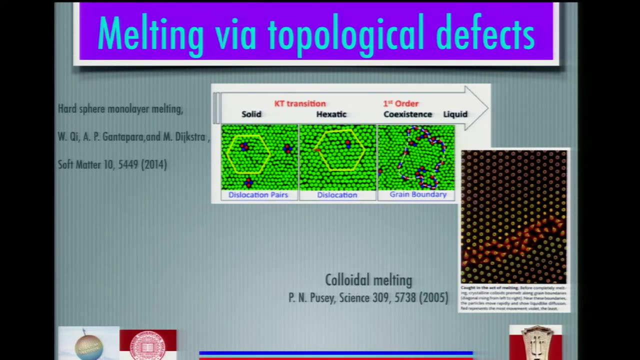 be in disguise, a melting transition in which topological defects appear and so on, but not in an obvious way. So this is, of course, what I just alluded to, that you have, as of course you know, and some of you of course, worked on it, that you can actually relate. 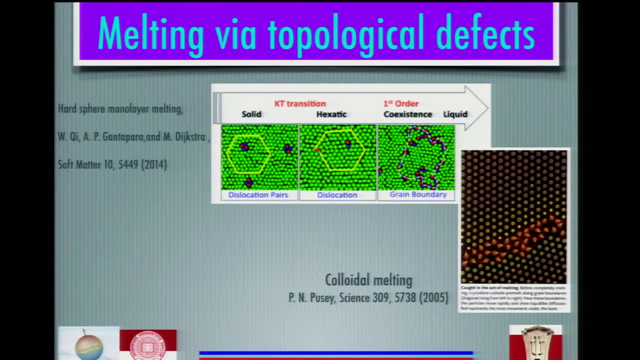 glass. You have transitions in which you have proliferation of topological defects, whether it be vortices, dislocations, discriminations, grain boundaries and so on, which can induce melting. Okay, so this of course, I guess you all, of course know. And let me tell. 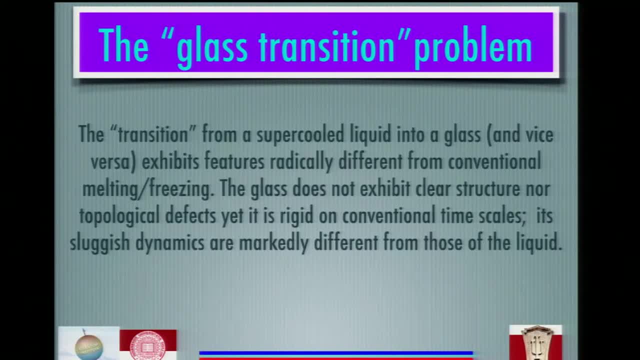 you about what the problem is. What is a glass transition problem? This is a very, very old problem And, of course, if there are any questions, please stop me and ask questions. So this is a very, very old problem and the problem really is the following: You take 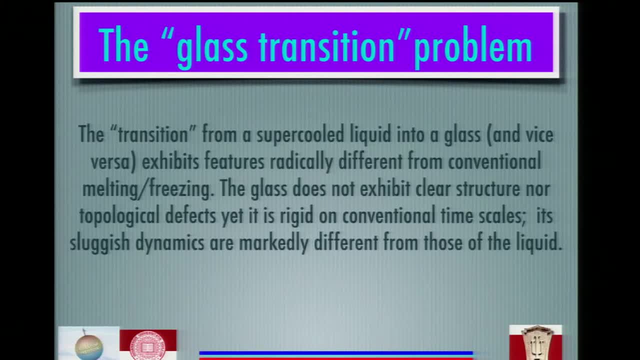 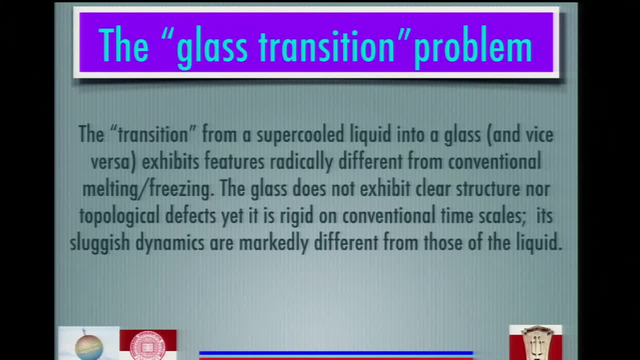 And if you cool it down slowly under ambient pressure, it becomes a solid. On the other hand, if you cool it down fast enough- and of course what enough stands for depends from material to material, But if you cool it down fast enough, it does not crystallize. 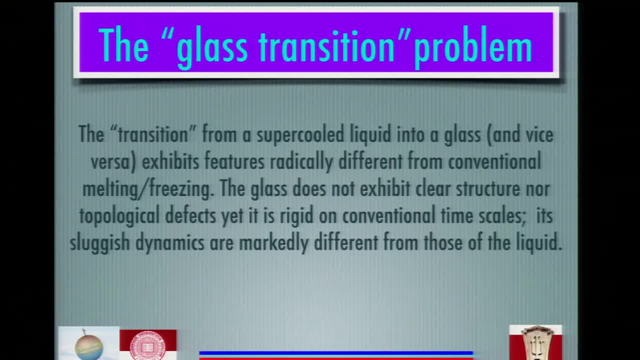 And some. It has a higher and higher viscosity. It's a so-called supercooled fluid. It's supercooled below its melting temperature And at some stage the viscosity becomes so high that it's called the glass, When viscosity exceeds the threshold value. 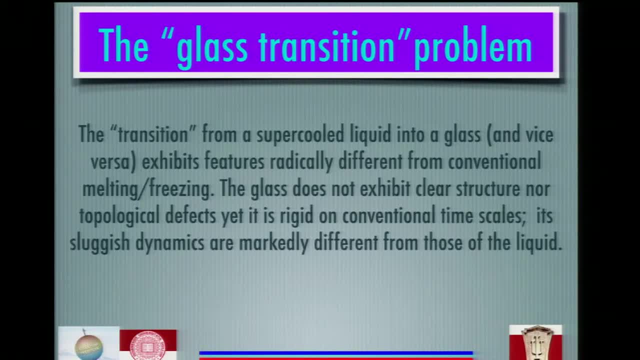 which is a bit arbitrary: 10 to the 12 Pascal seconds. people just call it the glass. Now, the problem really is that, even though we get to this material, this phase in which viscosity is tremendous and it seems to be solid, and all for many practical purposes, 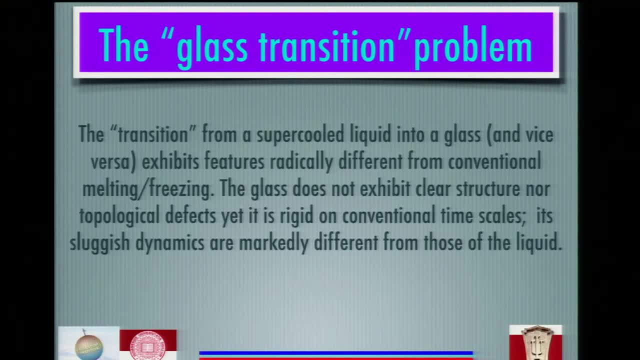 nothing really happens dynamically. So if you look at heat capacity measurements and so on, there's nothing really there. You might see a small blip here and there and so on, But the changes that you actually see are not profound. By contrast, if you look at the dynamics, 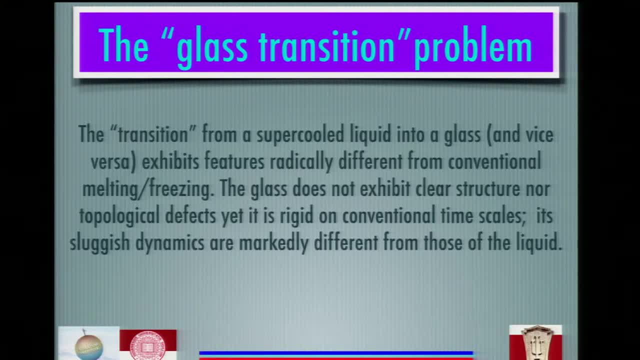 the dynamics change dramatically, The viscosity ultimately shoots up by orders of magnitude. It's not uncommon to actually have just a viscosity and time scales by totality. It's not uncommon to have a viscosity of 12 order magnitude or 15 order magnitude over a relatively narrow temperature. 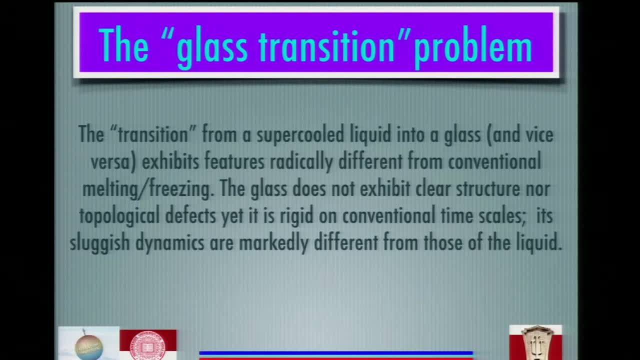 range. So dynamics increases precipitously, But on the other hand ferrodynamics doesn't change that much And of course, as I guess you all know, the structure of these materials is pretty amorphous. You can actually find short-range orders and so on. 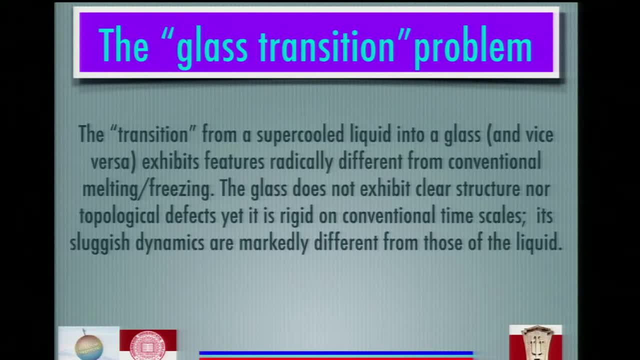 but it's nothing like a crystal. of course, This is very much unlike conventional transitions, in which dynamics and ferrodynamics go hand in hand. You want to think there's a tremendous change, but ferrodynamically nothing, really nothing profound- as profound really happens. 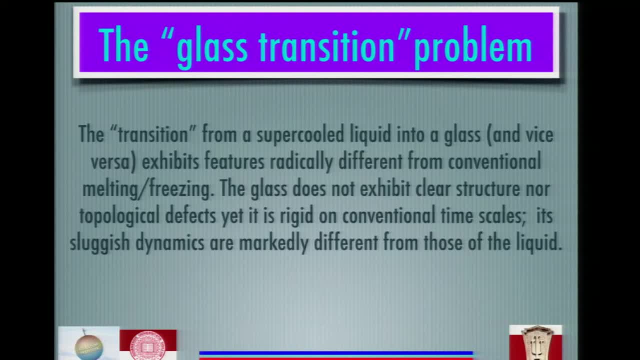 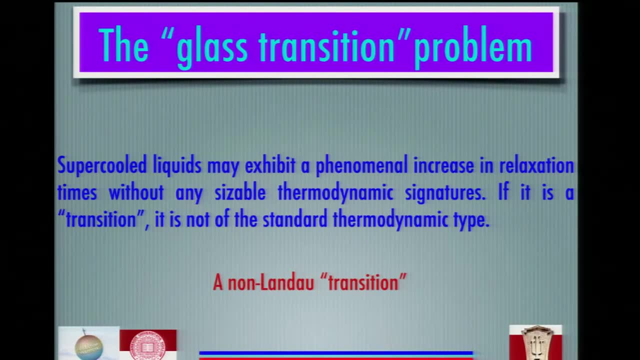 And that's a problem. How can this be? What's going on here? So, basically, as I just alluded to, and so on, so you can have a huge change in relaxation times, but there's nothing really profound dynamically. So if it's a transition of any type, 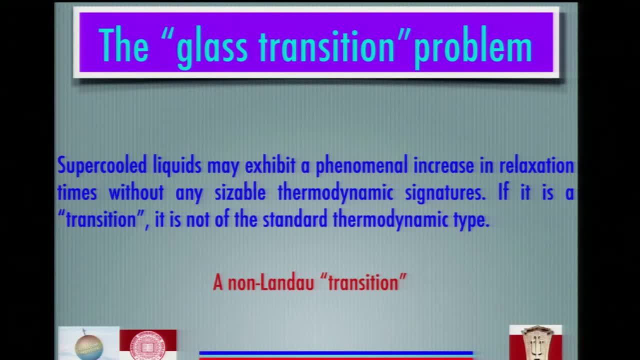 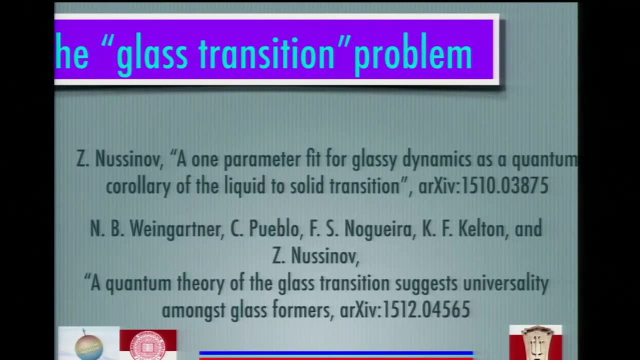 and people do call it quite often a transition. it's certainly not of a Landau type. That's the conventional wisdom. So we did some works When we worked on this. I'll just mention my former student, I apologize. I apologize. 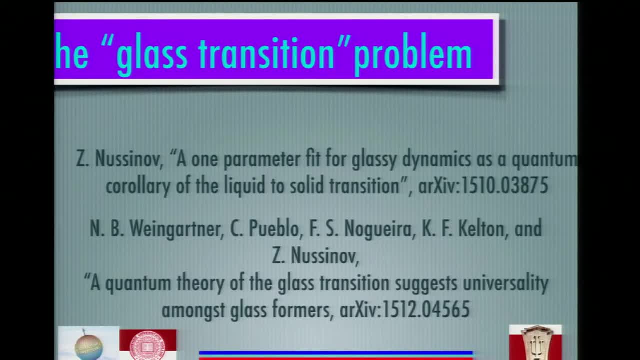 So Nick Weingartner- he was my former student. He just graduated. This was work done with Flavio Nogueres. He's a little field theorist. Ken Kelton is an experimentalist in our department And these are my principal collaborators on this. 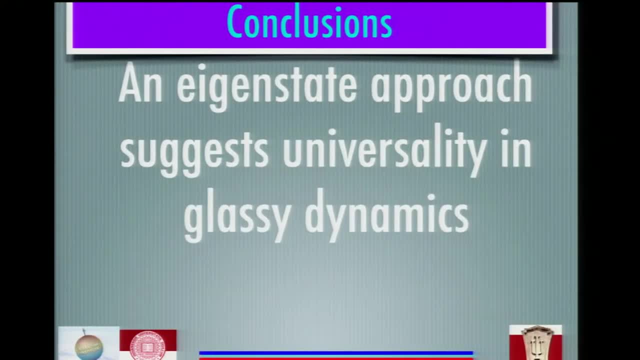 OK, so before I run out of time- and I will run out of time pretty soon- let me tell you what conclusions really are. So, conclusions sort of are, but if you think about this problem, which seems to be classical- and of course you might say it's sort of silly- 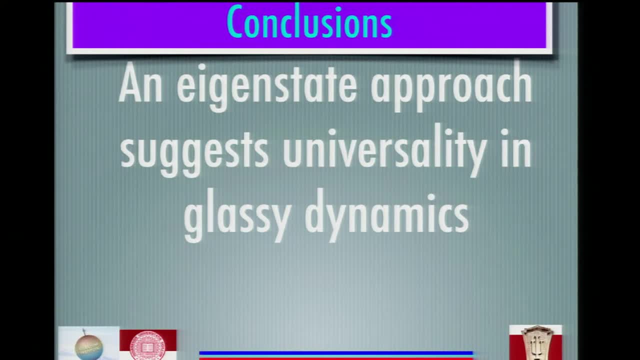 to think about this problem quantum mechanically. Nonetheless, if you think about this problem quantum mechanically- OK, Think about the terms of eigenstates and so on In a very, very simple setting that I described to you- then that approach suggests that there 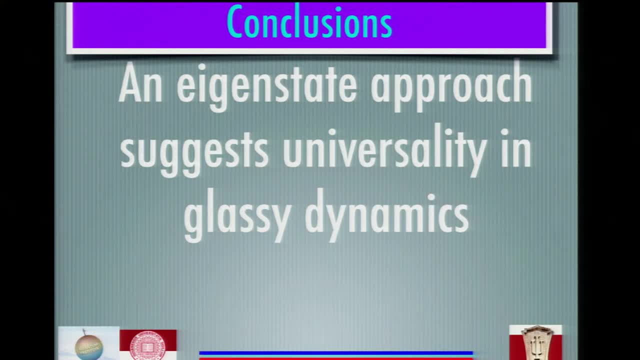 might be an underlying universality in which the only important energy scale in the problem is vanadon, equilibrium transitions in which you have topological defects, the usual type of melting. OK, That's basically the conclusions from this theory, which of course has consequences, if it's, of course, correct. 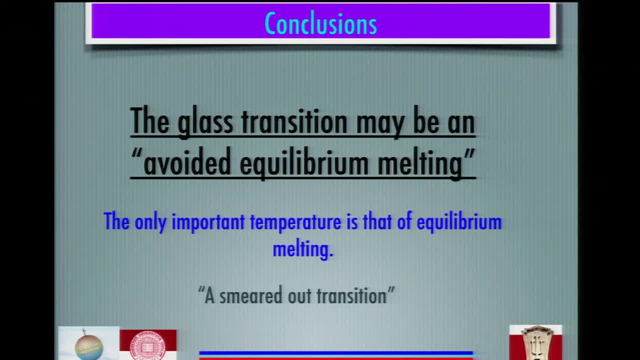 So, as I just alluded to, basically the idea is is that you have a melting of some type, But it's not obviously usual melting, otherwise of course you would have all the usual hallmarks of conventional melting transitions, But it's sort of a rounded off melting transition. 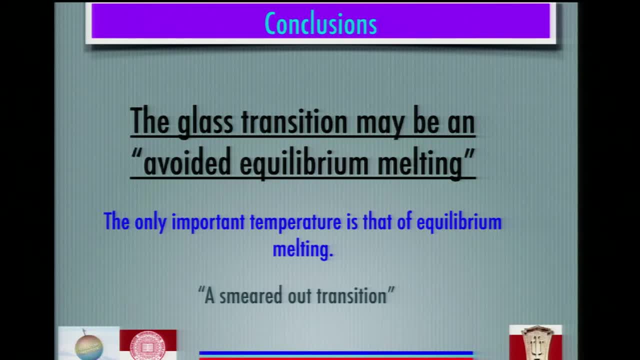 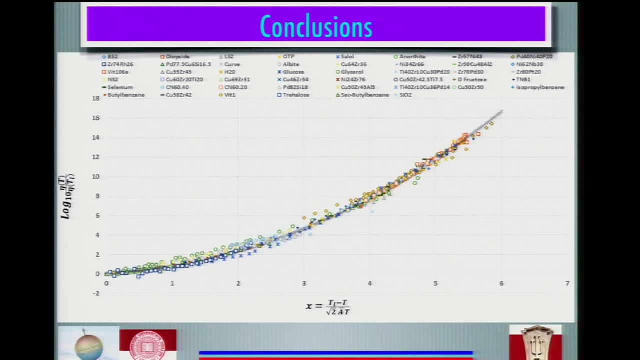 OK, And nonetheless, the only important temperature scale in the problem is vanadon equilibrium melting. So here's a prediction of a theory. So according to this theory, as I just alluded, by now, four times the only important temperature scale. 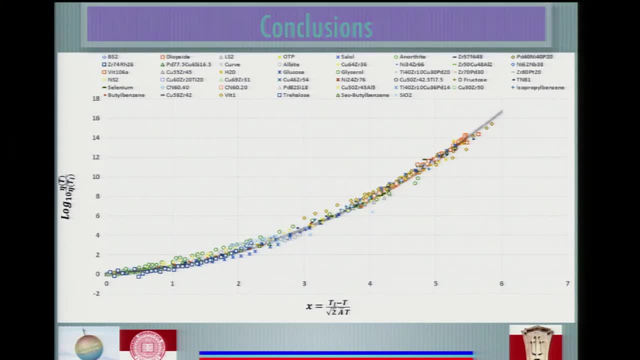 is vanadon of melting, or, as people called, the liquidus temperature for when you have supercooled fluids. I apologize, I'm going too fast here. So that means that you could actually- if it's indeed true, you can actually scale viscosity data, which is drawn here. 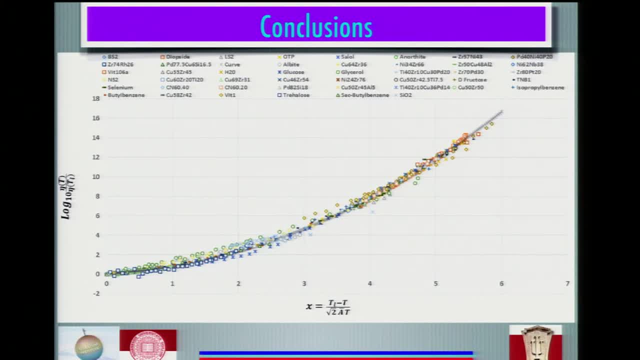 on the horizontal, on the vertical axis. So the viscosity that you measure for supercooled fluid at a temperature of T, you divide that by the viscosity measured at the melting transition. it's going to be melting same supercooled fluid. 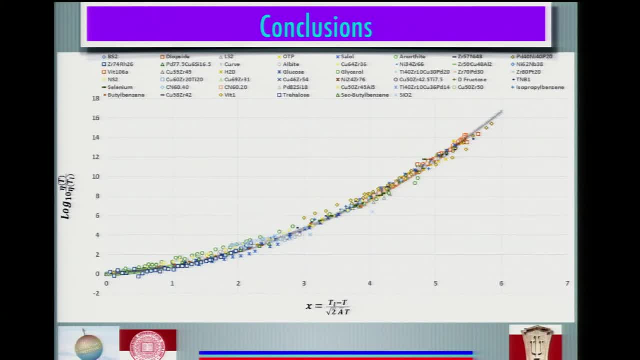 And you plot this, And this is a function of a dimensionless quantity, which is how far below you are relative to global melting. OK, There's only one dimensionless parameter here, which is a bar which varies from fluid to fluid. 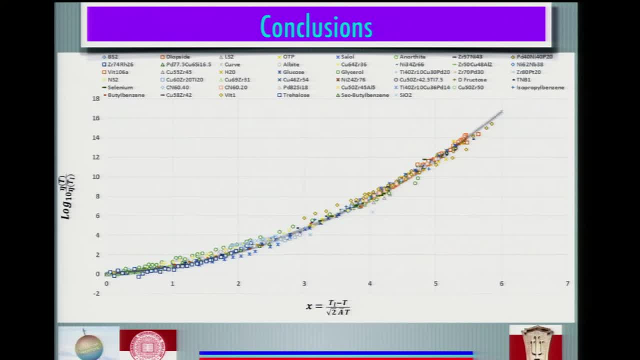 but doesn't vary that much. It's an order typically of 0.07 numerically And as you can sort of see here, regardless of a figure I'm going to try to describe to you, a figure might be wrong, it might be right. 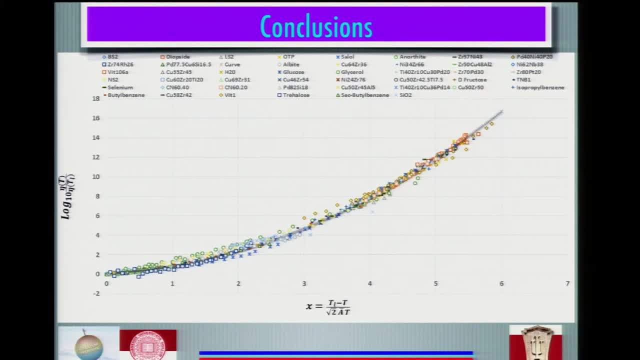 But regardless, it's sort of a fact of nature. But all of these different fluids that actually are plotted here, they collapse into one universal curve. So that strongly suggests that, whatever the mechanism really is, the important temperature in the scaling problem is really that of global melting. 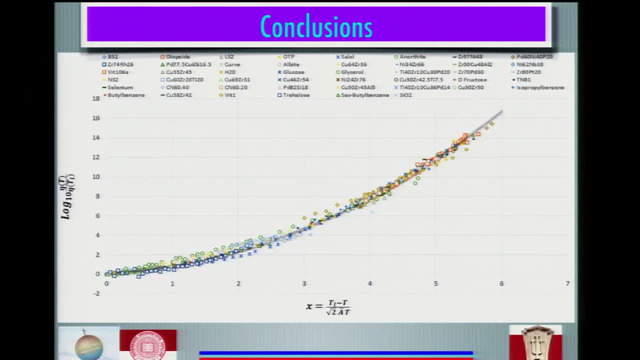 Otherwise why would 45 different fluids collapse here on one universal curve? And as I show you momentarily, you actually have even more fluids that can collapse. So here, for instance, we have 66 different fluids that can actually collapse on the one universal curve. 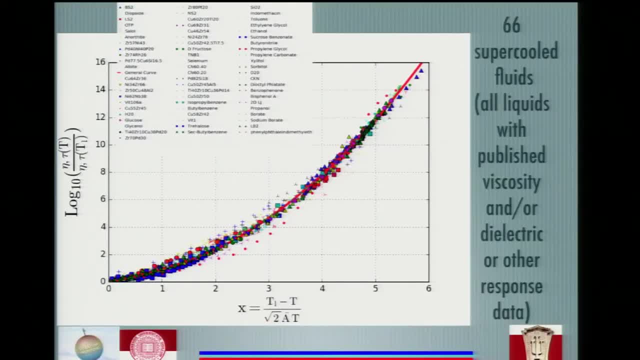 So here's another rendition of the same thing here: 66 different fluids, OK, On the same curve, And here we have both the viscosity data and also other measurements of relaxation data, like what you have from that response and other quantities. So sort of. you see that there are some outliers, of course. 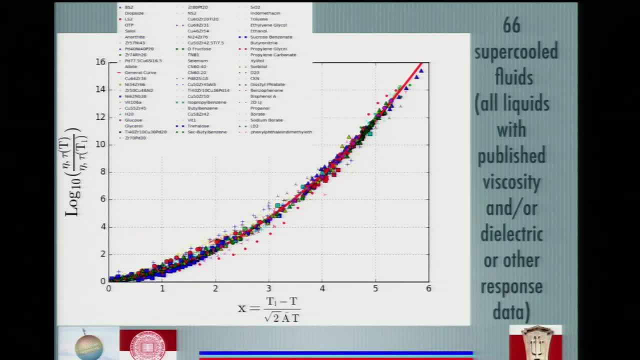 as you see here and so on, But by and large, all these different fluids- 66 different fluids that we can actually could find data on in the literature, they all collapse into one universal curve With only temperature scale, which is really important. 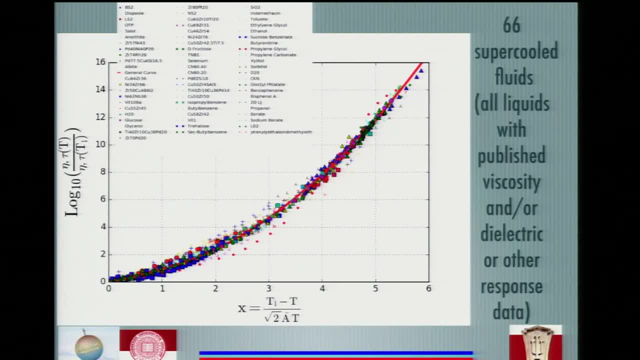 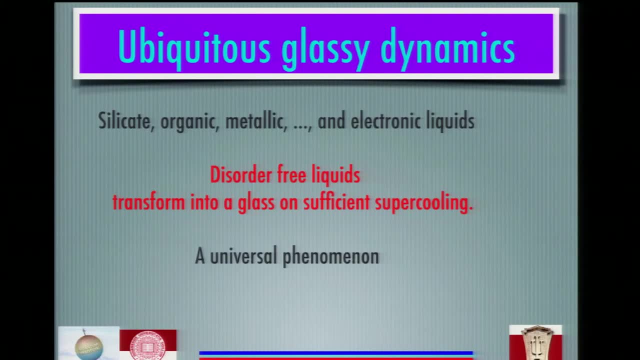 as I now say, and time being very, very important, And that's the point being that of a melting transition. So, as I alluded to earlier, glasses are ubiquitous, So you can, of course, have them in ordinary window glasses. 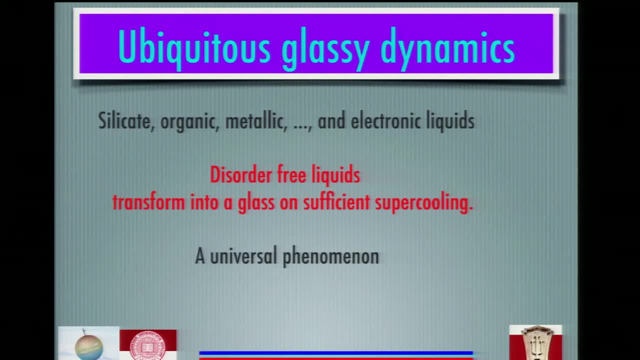 Yeah, I'll tell you a moment later on. Yeah, The global filter has more parameters. Here it was actually, and it doesn't assume melting, You have only temperature scale. It was actually that of melting. So any fluid, as far as we know at least. 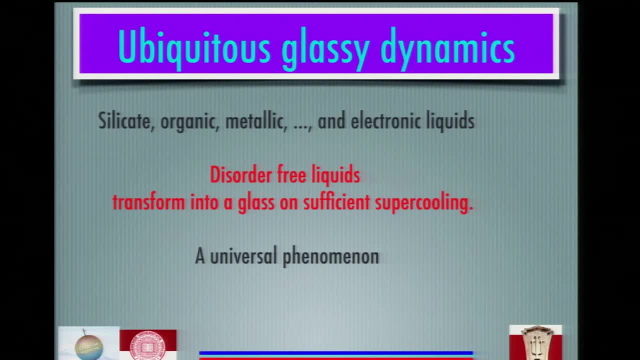 can be made into a glass under the right conditions. So basically, you just have to quench it in an appropriate way, So by any fluid, as I mentioned earlier, you can think about window glasses, so look at glasses, which, of course. 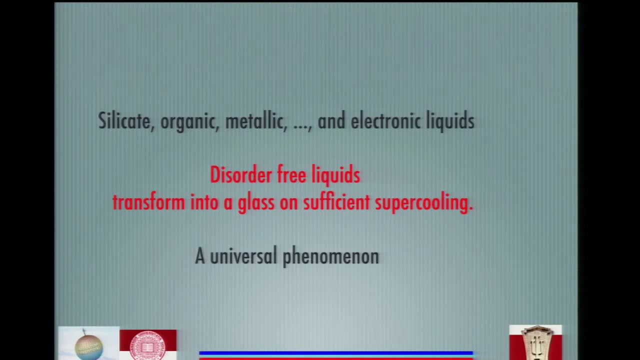 have been known for millennia. If I think about all sorts of many organic fluids, you can think about metallic fluids- So metallic glasses are actually quite hot, and so on. Also, you can think about the electronic fluids that are actually Exhibits of the hallmarks of very, very slow dynamics. 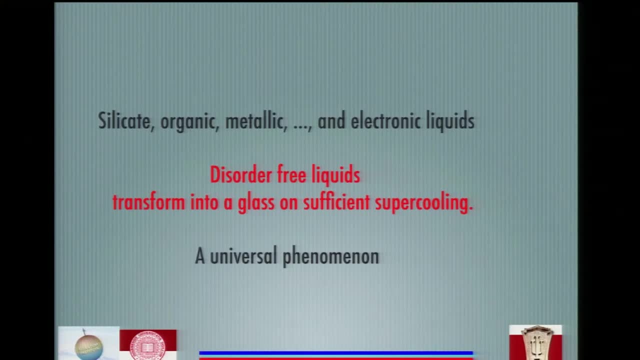 as you have the NMR wipeout and other signatures and so on. So, basically, the key point is that any, as far as we know, any disorder-free fluid, if you cool it down fast enough, it can become into a glass. 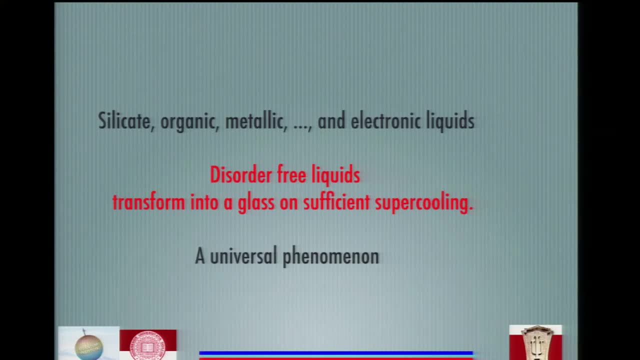 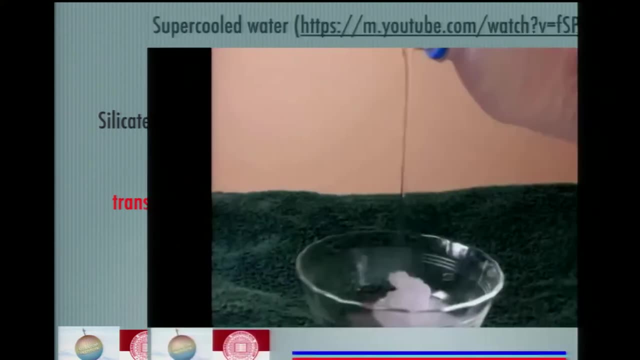 OK, as I told you earlier, how fast you have to do it depends on the material, But in principle, any fluid can become glassy, So it's a universal phenomenon. And here is an example of this universality in your kitchen. 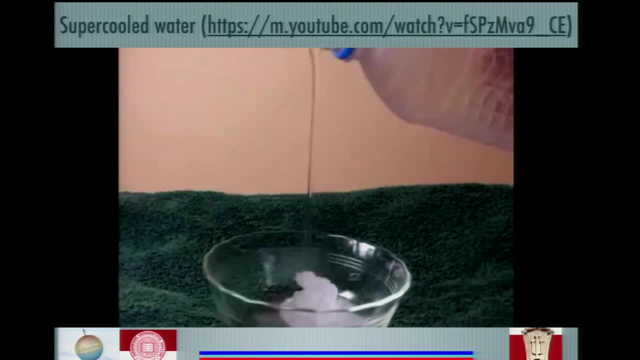 So you can take basically a plastic bottle and fill it up with water. But water really has to be pure water. The norm: purity is there, Otherwise it would crystallize. So fill it up with water, Take that bottle, put it in the freezer. 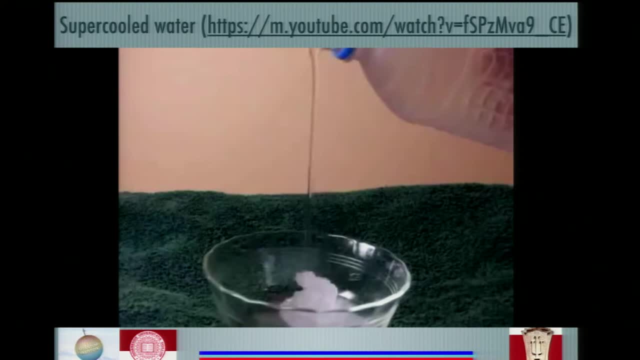 and wait for about an hour And after an hour open the freezer and take it out very, very gently out of the freezer. So don't perturb it in any particular way. Take it out very, very gently and pour it into a glass. 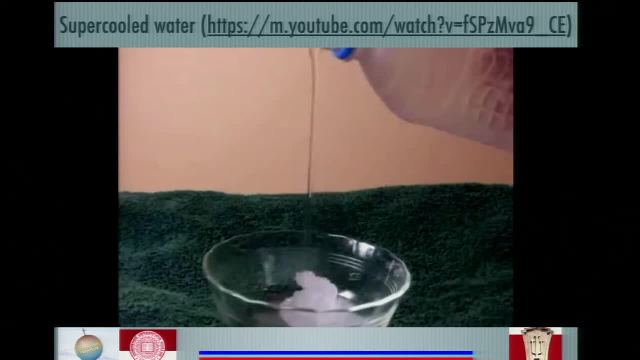 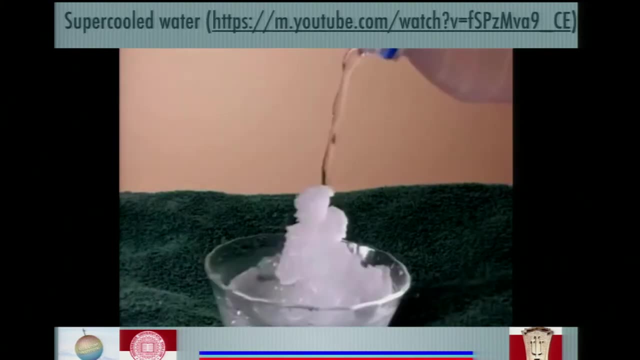 or container, And as you pour it down and the water strikes the surface, it will start to crystallize. As you pour it down more and more, you'll have this column of ice that develops. So what happens here is you have water which is super cooled. 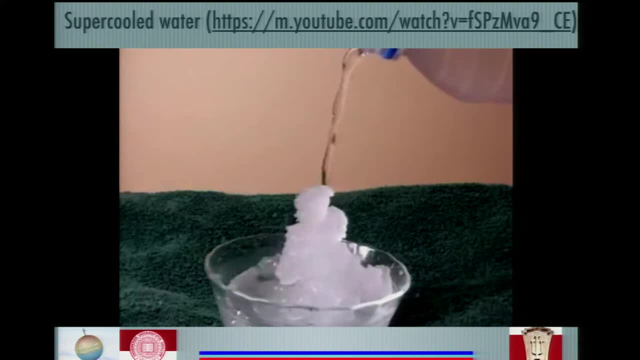 And actually it crystallizes because upon striking in the container surface actually there's enough energy that it actually has to trigger and start the nucleation process which proceeds. If you perturb it a little bit, you can actually crystallize. 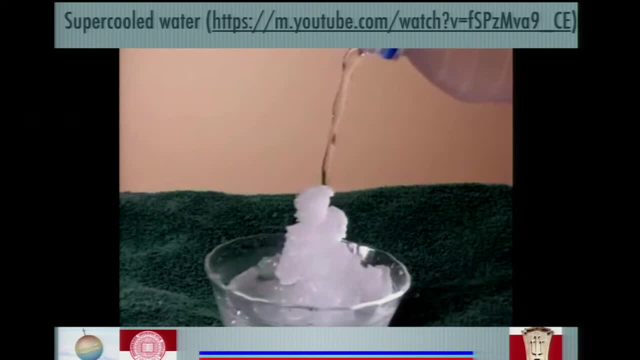 Actually, you can see in videos that we send YouTube, people try it over and over again. It's not easy to actually do it because usually there's some perturbations that you actually have, But if you do it in the proper way, 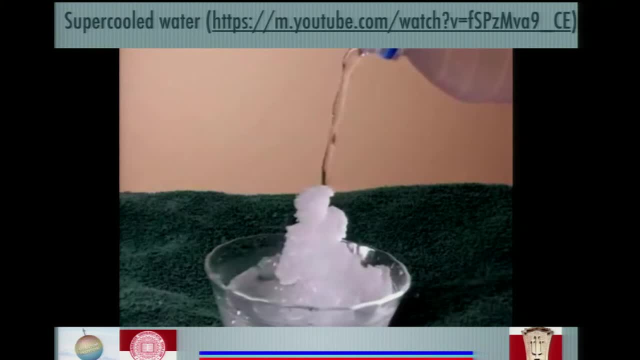 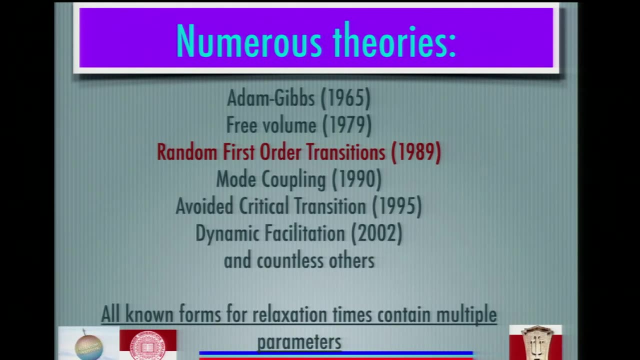 this is actually what will happen, And then not only water, any material in principle can be super cooled, Because this is a universal phenomena. of course, many, many theories try to explain this universal phenomena, which is substituted, sort of alluded to here. 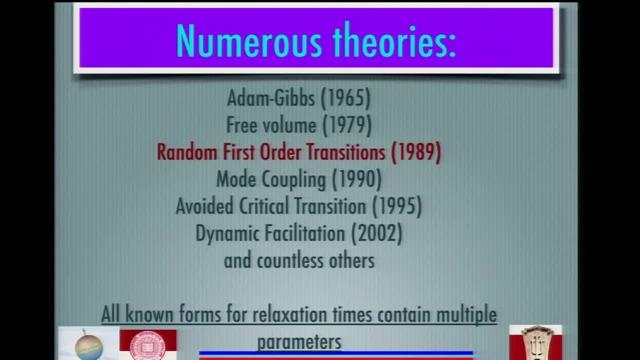 So these are many of the, and currently even one that's sort of most in fashion. is this random for those who are in theory? But many of these theories have very natural ideas, For instance, if you think about so-called dynamic facilitation. 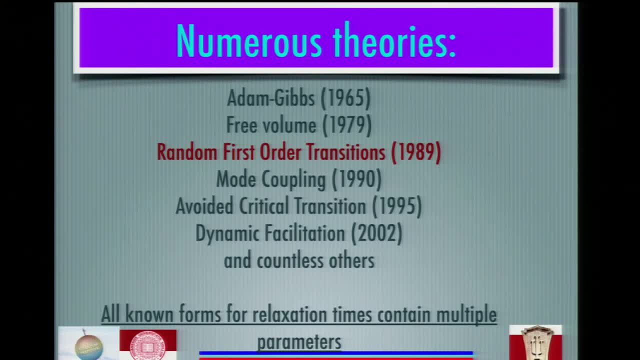 the idea there is that you think about a subway, but you want to get out of the subway. In order to actually be able to move, other people have to get out of your path, So you have to have some correlated motion And of course, that motion can become inhibited. 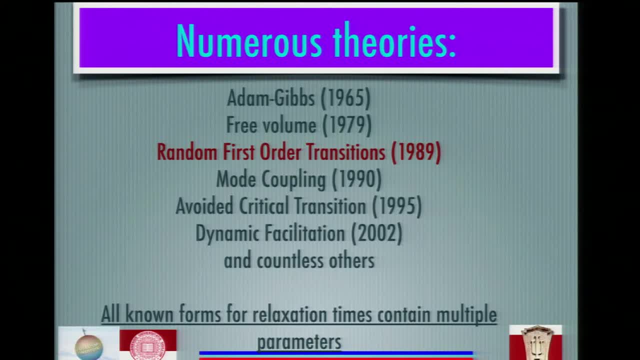 when there's not much way to move. So you can have very visual dynamics, but it was also governing laws of how we can actually move. So what is your role in all of the theory that it's very pure water and you have this thing for? 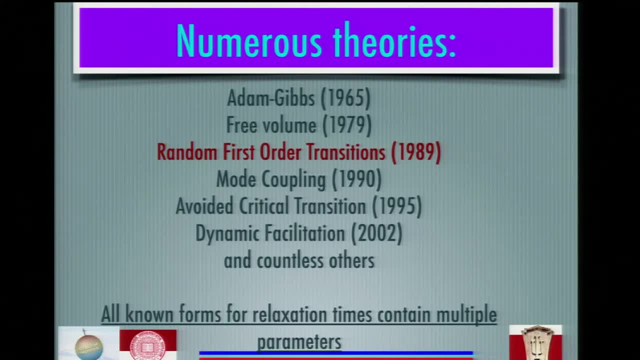 So it would just strike the nucleation site. So within that one hour then the fridge is going to It will be just ice. You'll take it out, just ice. If you stay longer, typically it will just be also a bottle of ice. 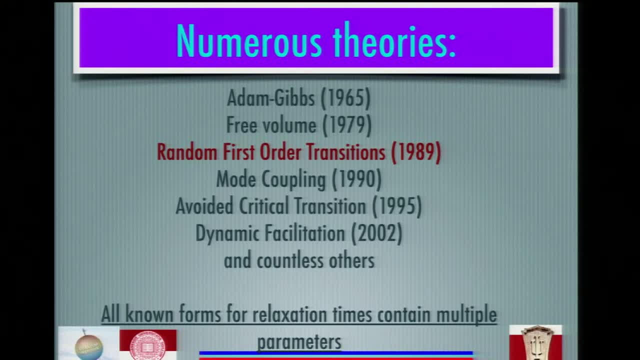 But yeah, if it's pure water and you do it right and no perturbate, it will do just that. And, of course, many other theories. OK, And all of these different theories. they contain multiple parameters And, in particular, as far as what I want to emphasize here, 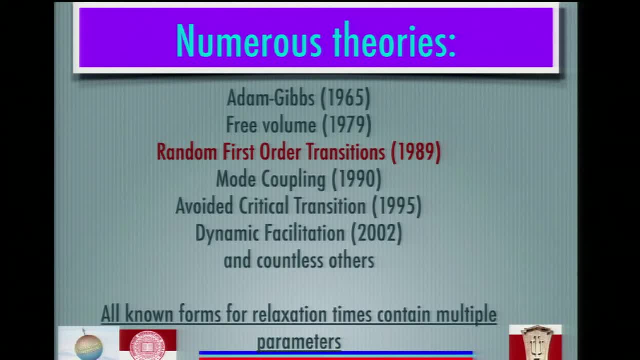 these parameters are different from that of conventional melting, So it's always assumed to be that whatever it is that underlies this phenomenon is radically different from usual melting. But, as I showed you earlier, for whatever reason it actually is, it seems to be that you can actually collapse the data. 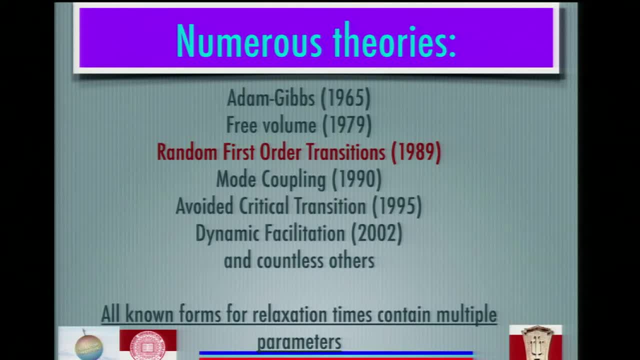 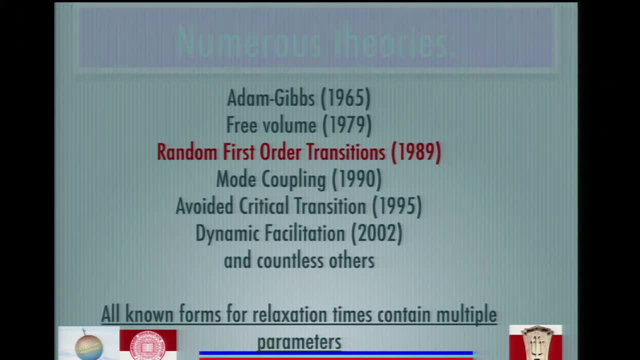 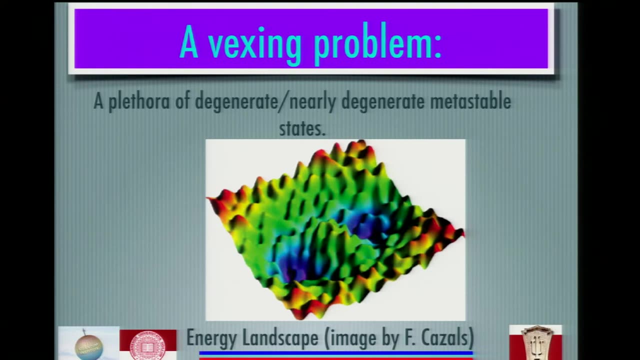 of the viscosity And of relaxation data, but you can actually find the literature on two universal curves, OK, So it seems to be that actually the two things are related. So the conventional picture people have, literally and figuratively, is that of an energy landscape. 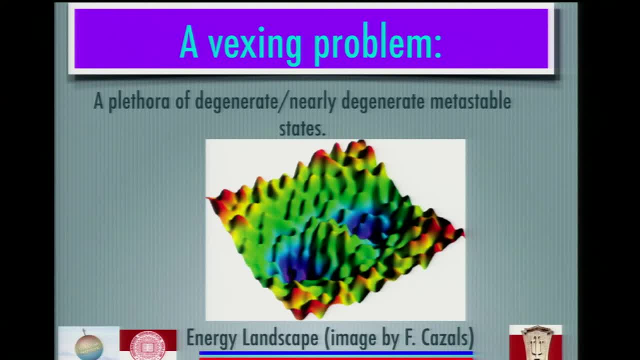 So you think about high dimensional space in which you have many, many different degrees of freedom And you can think about starting in some particular place And you want to make your way slowly- or not so slowly, ideally- into the true OK. 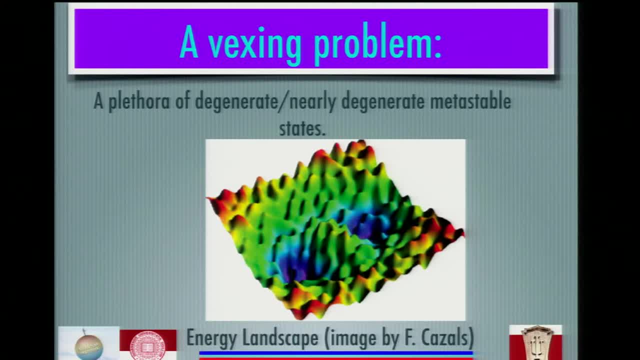 Ideally, you have a low energy state, But of course you have problems because you have to surmount barriers in order to go from one place to the other, And that's the origin, as people discuss for a very long time, in very different contexts, of course also. 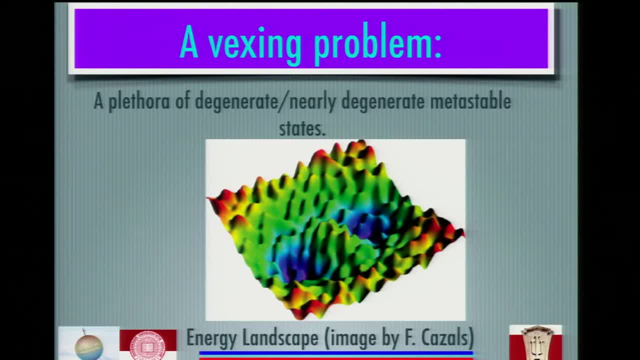 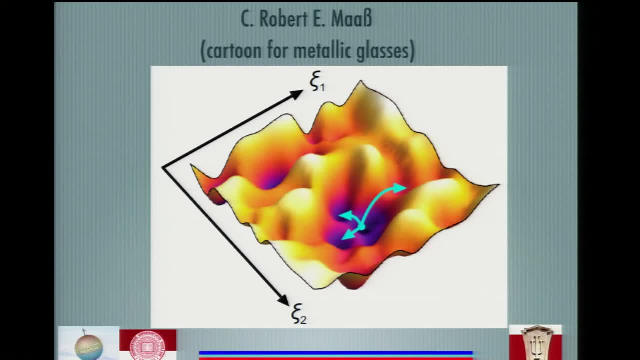 person folding and so on, of why a lot of dynamics actually onsets. OK, This is never a cartoon of the same thing. So you want to go from one basin to another basin, But of course that's not trivial because you have to do it many, many times. 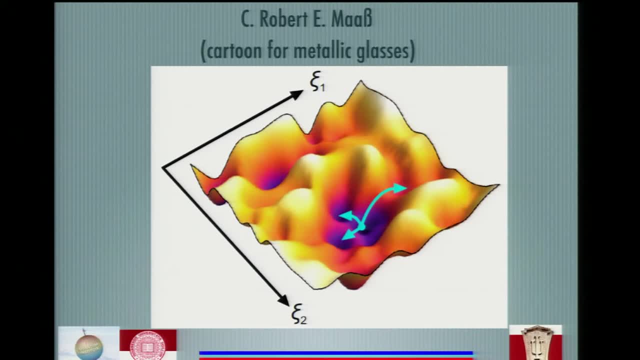 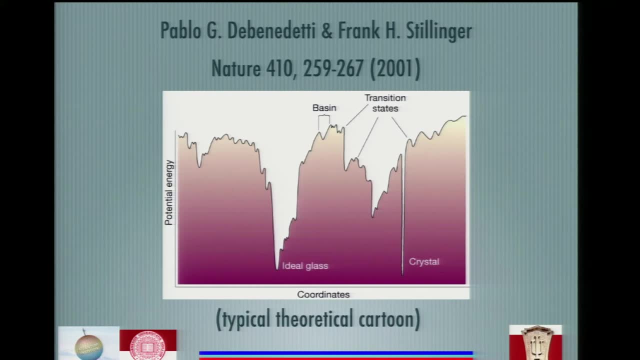 And you have to overcome barriers and so on. Hence the dynamics is slow. This is never a common cartoon you will find in many papers And this cartoon, as you can see here, on the vertical axis, I apologize. And the vertical axis is energy itself. OK, 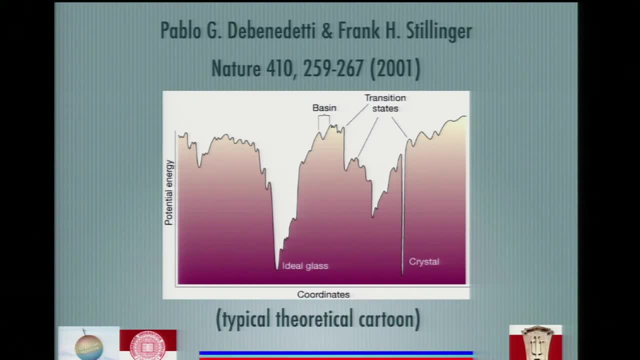 On the horizontal axis is some generalized hypothetical coordinate that you think about, And of course this is a high dimensional cartoon, but here we only draw a small cross-section of it. OK, And you can actually think about achieving the ideal crystalline state which appears here. 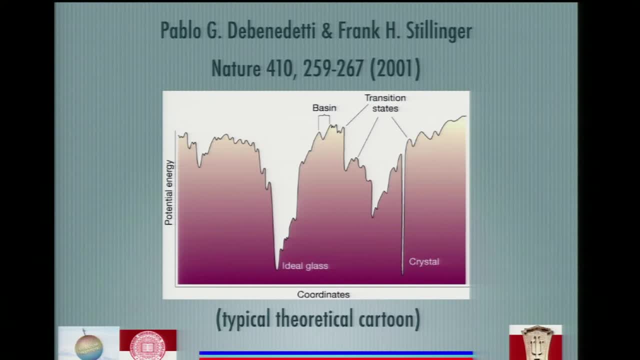 OK, But you can also very rarely get stuck in these small basins that are everywhere here, And at low enough temperatures you can actually go into this so-called ideal glass state. That's the conventional wisdom In most. this is not by everybody. 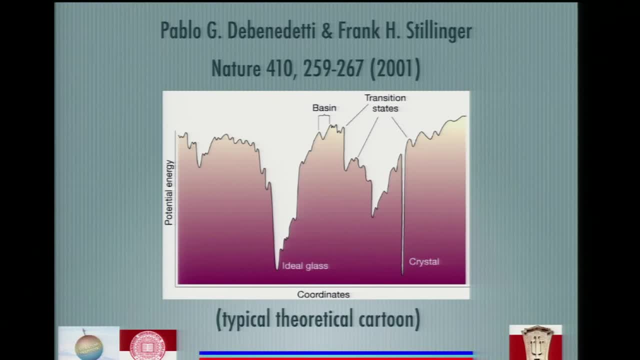 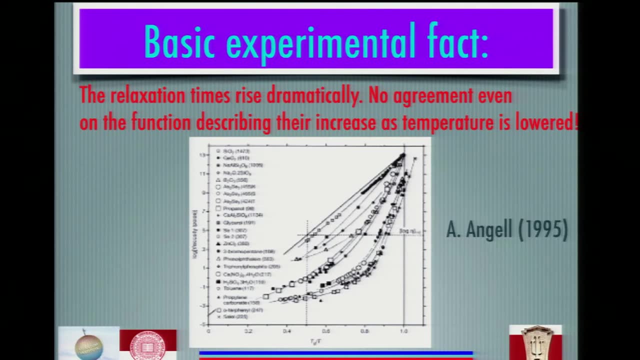 but that's what most people actually believe occurs Now. I mean, you asked earlier about global culture And earlier also also the fragility, Yesterday very, very briefly talking about global culture and so on. So this is a copy of it- from a very, very famous paper. 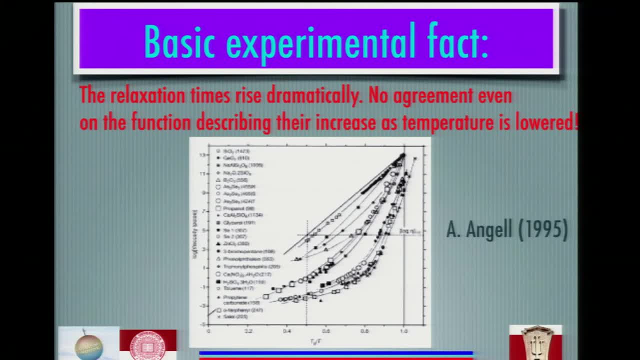 influential paper from 22 years ago by Austin Angel in which you cannot read it, nor can I. But here are very disparate fluids And what's plotted here is the log of the viscosity divided by viscosity. at the glass temperature, The viscosity becomes 10 to the 12 Pascal seconds. 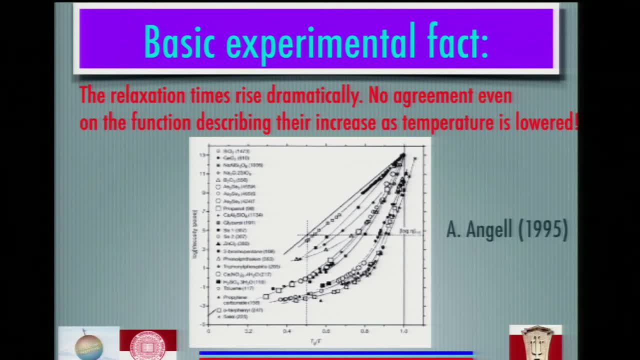 As a function of this reduced temperature, which is Tg, the temperature at which the system becomes, the glass divided by the temperature itself. OK, As you can see, of course some fluids don't deviate a lot from a straight line. 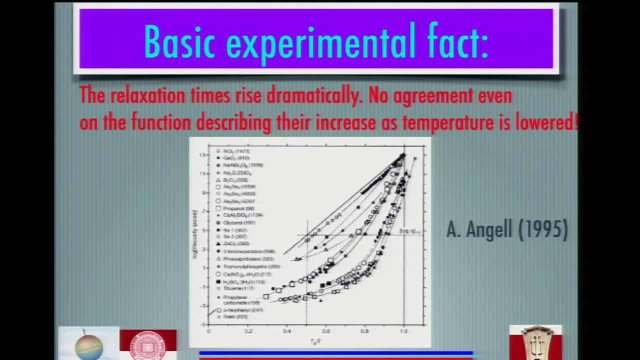 A straight line here on a log scale means activated behavior. It's a behavior. It means that the temperature scale, the viscosity, goes, like e to the power of some energy scale divided by temperature. OK, So we want just one of our temperatures. 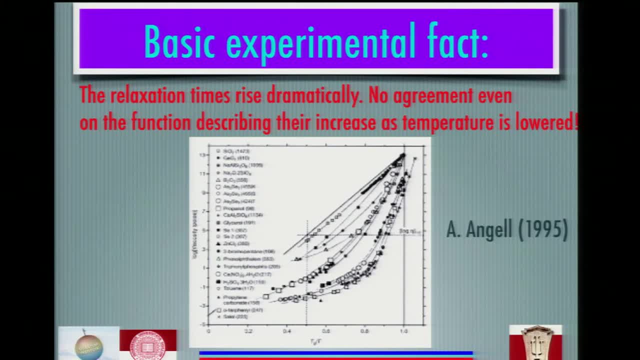 One of our temperatures, which is, of course, what appears here in the log. That's not surprising. Some fluids, like the silicates, don't deviate from a straight line by a large margin, And they're called strong because it's. 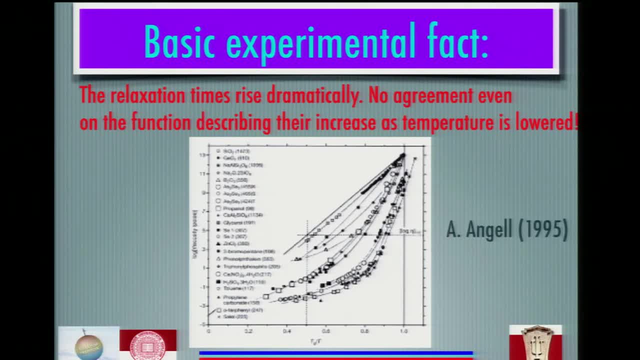 assumed to be structural, that they actually doesn't change that much, And that's why the energy barriers are sort of constant And that's why nothing really changed dramatically. On the other hand, some fluids, like this one ultrafennel- you can sort of see here that I have five minutes- 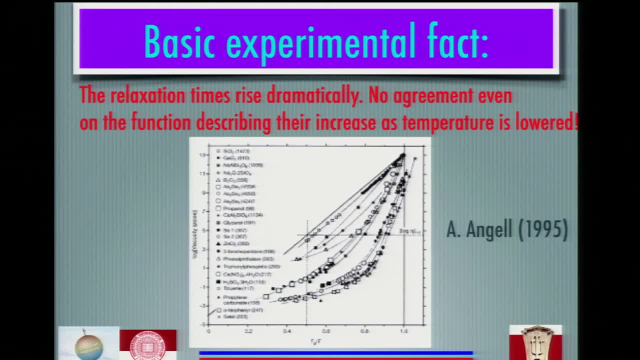 left. OK, sorry, You can sort of see here that the viscosity shoots up by magnitude. so by magnitude, and going from this point here all the way up to the top scale over a narrow temperature range. These are called fragile fluids. OK, 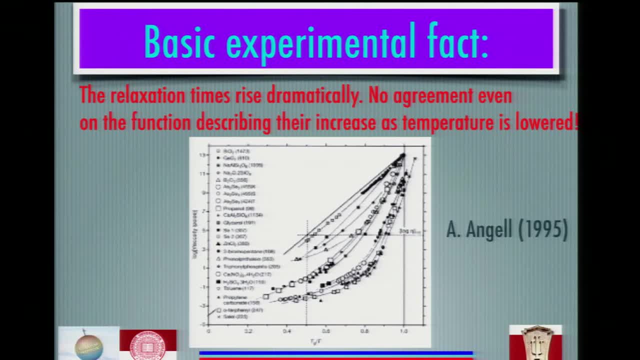 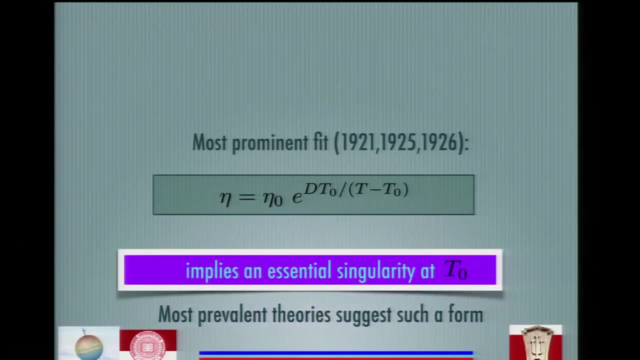 They're not strong, hence they're called fragile. And the most common fit people have for this, as you can see here, As I asked earlier, is the so-called Vogel-Focher law. This law was introduced empirically with no theory. 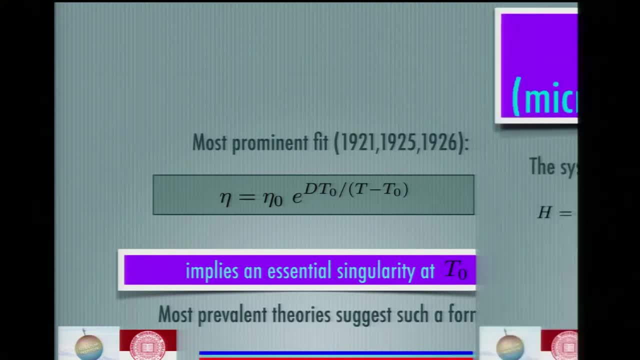 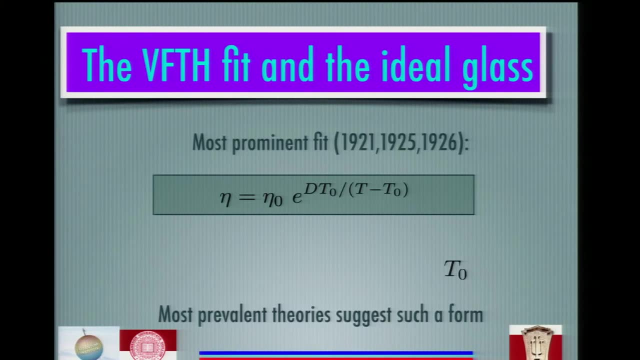 95 years ago, as you can sort of see in these papers, I apologize- And as you can sort of see here, if you believe this form. so basically, what this says is that the increase in the viscosity is faster than the radius. 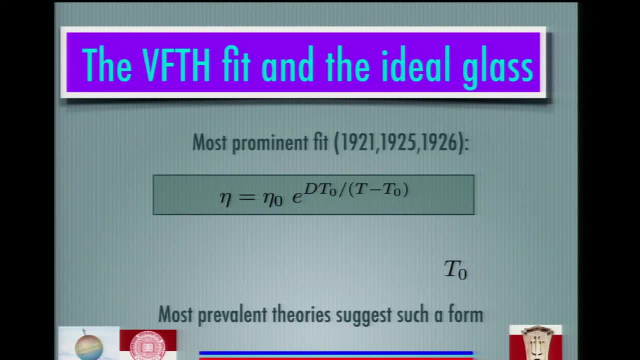 It's not either the power of some constant divided by temperature, but either power of a constant divided by a temperature minus another temperature, T0, OK, So it increases more rapidly than it would have been if it was simple activated behavior And of course this implies, if you believe this form: 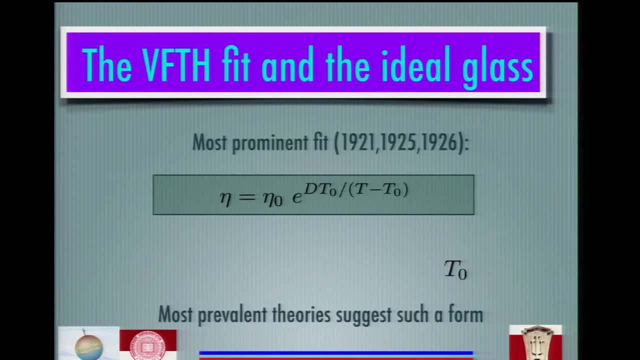 that there's some essential singularity that occurs as temperature: T is equal to T0, T is equal to T0. And that's presumed to be this ideal transition to the glass, what I showed you in this cartoon: that you have this ideal glass that people actually 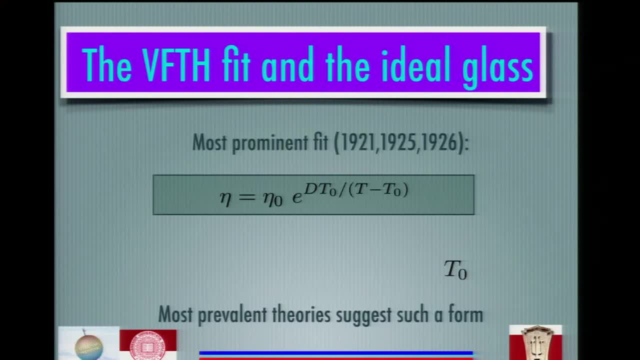 believe is associated with that And most theories try to derive this form. And in this form you can sort of see that you have three or at best two parameters. You have this pre-factor here, this A0.. You have this constant D, You have this temperature T0,. 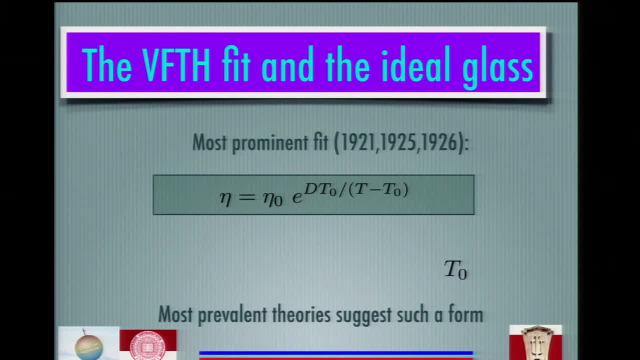 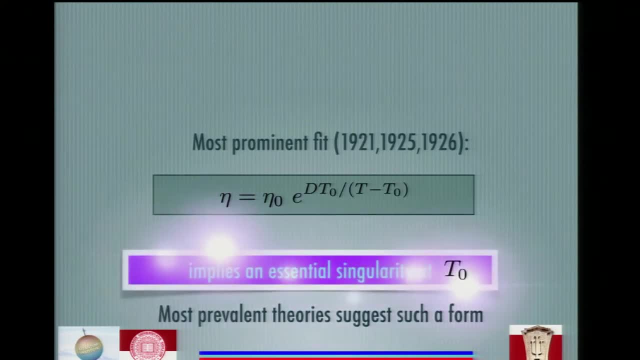 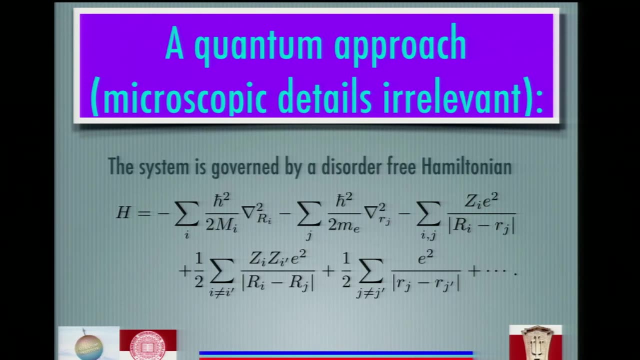 at which divergence occur. And nowhere here in this form is there any relation to could be melting. It's assumed to be completely different. Now, my approach is quite different And you might say naive and sort of silly and so on. 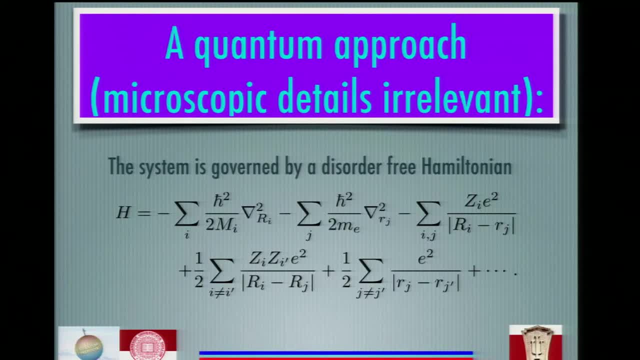 But we'll try to solve it as a homework problem And quantum mechanics, And so we'll try to write down the many-body Hamiltonian which of course we can all write down But none of us, of course, can solve it. 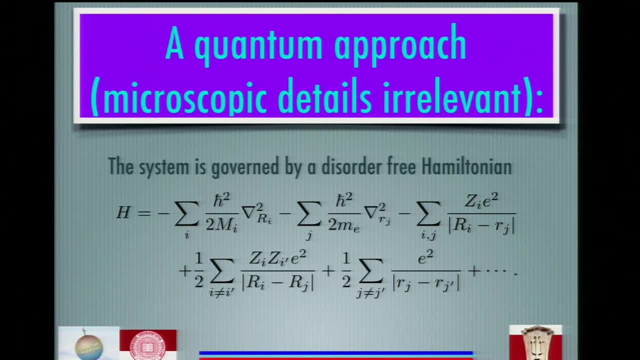 But let's write it down nonetheless. Let's imagine we write down the Hamiltonian for many-body system, including nuclei, electrons and so on, reactions, if you want to add in, and so on, And of course this is a theory of everything for us. 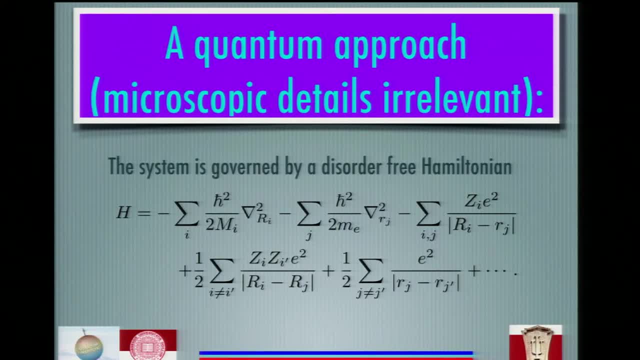 in some sense, But of course you might say it's because we cannot solve it, And you'd be absolutely correct. It would be typically, of course, useless to do, But it's not as useless as you might believe to be. 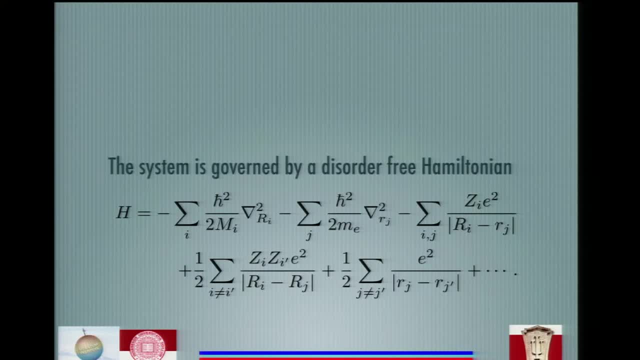 And the important thing here I should emphasize, and this is sort of a French rendition- This is a true glass, a real glass in the sense that the coupling constants in Hamiltonian that you see here, the real Hamiltonian there's. 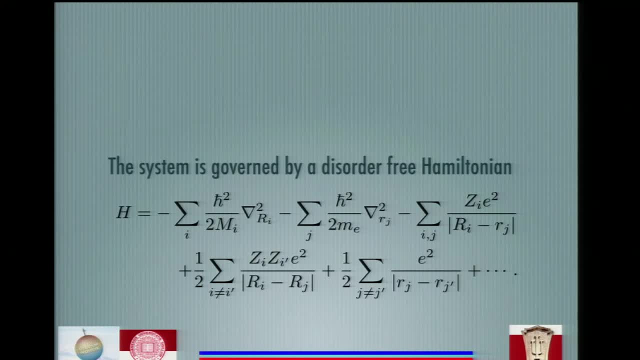 no disorder. The masses are just what they are. The interactions are what they are. There are no coupling constants here, which are random. It's not a spring glass. Even though glasses look distorted, the underlying Hamiltonian that describes the systems is uniform. 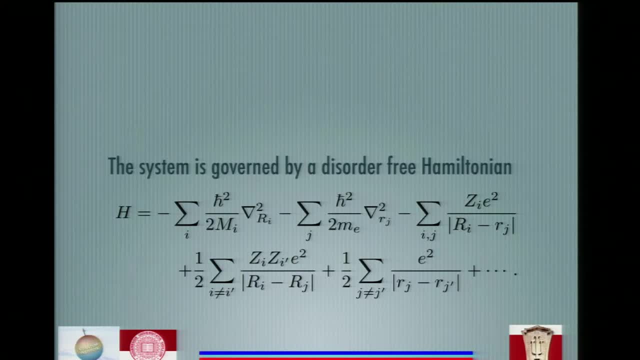 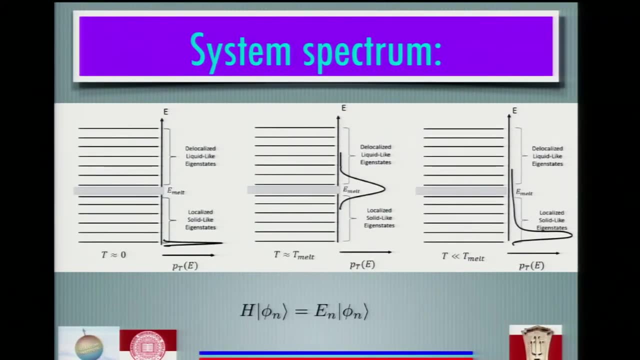 There's no imposed point of disorder. So in principle, of course, we cannot do this, but in principle there exists a completion of eigenstates. So let's imagine we label these eigenstates- I apologize, These eigenstates by here phi n. 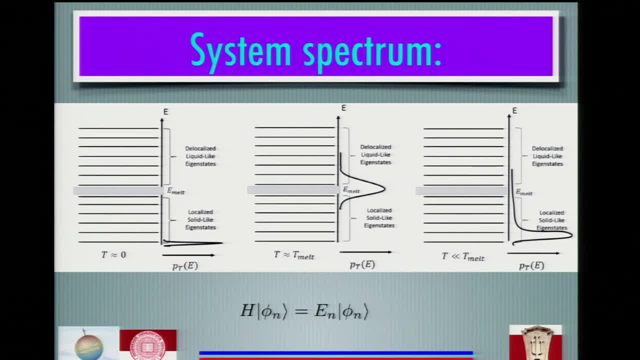 And we can write down, We can sort of plot the spectrum. Of course the spectrum is not the unit Ideally, like in harmonic, also like here. it's not equal to space, of course, As you go to higher energies, of course. 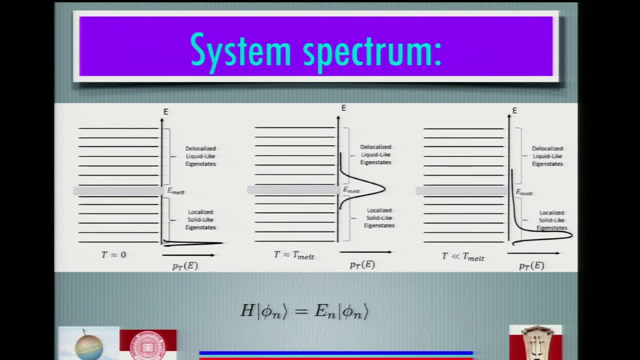 it becomes more and more dense, Entropy goes up, But nonetheless you have some spectrum, of course, to prove this problem And the solution to that. you of course have these eigenfunctions by here. Now, here is when I come. I'm sort of claiming: 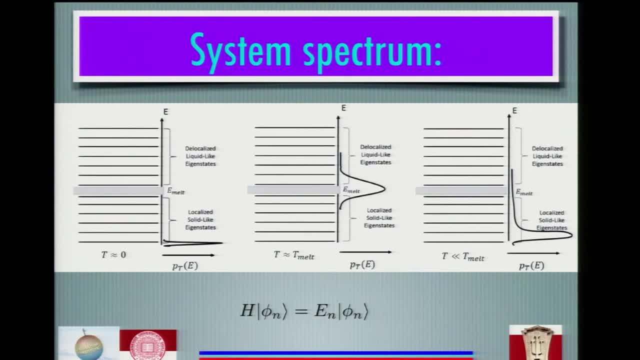 that all of these energy states here, these eigenstates here, at high enough energy densities. they correspond to eigenstates that have a fluid type. Even if I cannot solve this problem, I cannot die because I'm a Hamiltonian. I can sort of assert that at high enough energies. 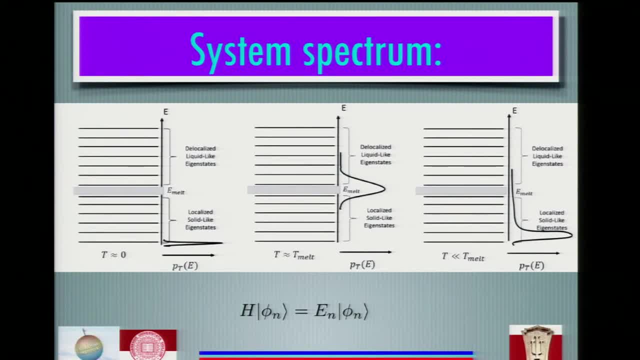 all of these eigenstates have fluid type characteristics At low enough energy densities. all of these eigenstates have solid type characteristics, And there's some intermediate range in energy densities in which eigenstates have mixed properties of both the solid and the fluid. Now why do I say that? 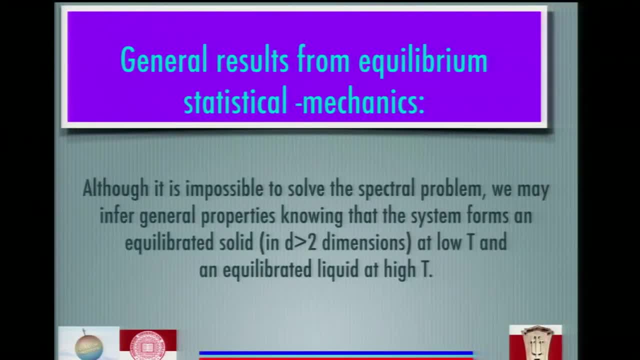 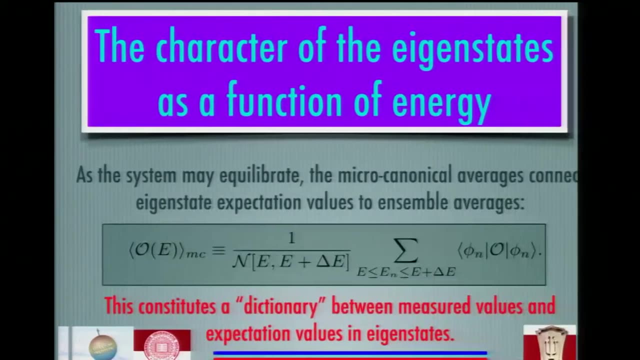 I can say that Why? Because we can use. we know that- typically in more than two dimensions for conventional systems. at high temperatures we have a fluid, At low temperatures we have a solid, And if we actually use any ensemble, 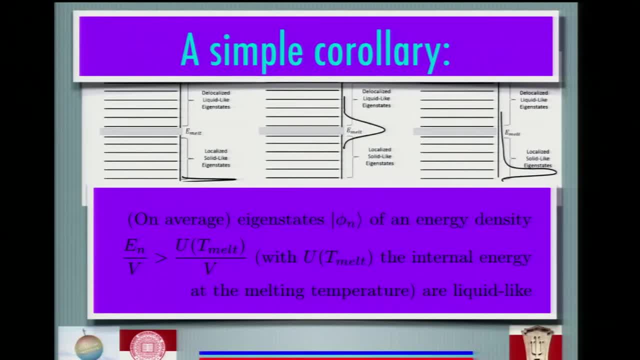 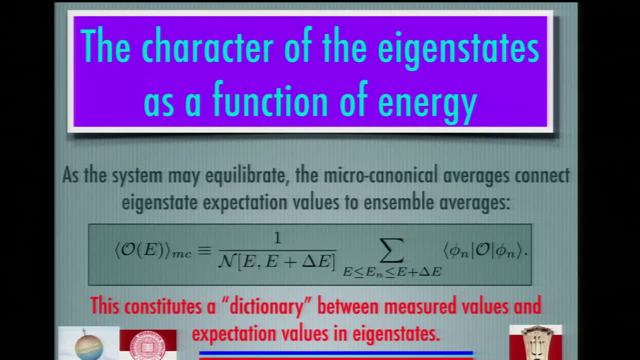 like, for instance, a mechatronical ensemble, any observable O. we can write down the coefficient value of O at an energy E in this ensemble. It has the average value that you have of addition of value of O over all eigenstates, phi n. 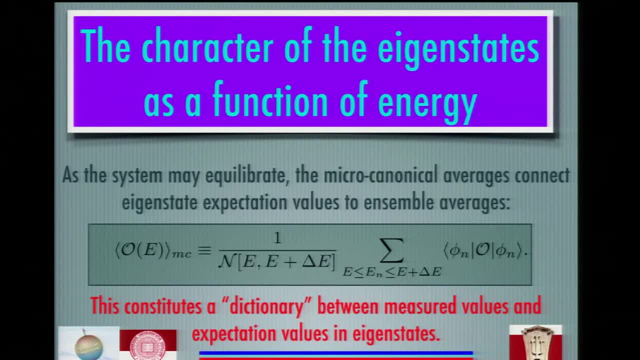 that line, some energy window of arbitrary width, delta E. The important thing about delta is it doesn't scale system size. It can be as large or as small as you want, but it doesn't scale system size. And in fact recently, in the last 10 years or so, 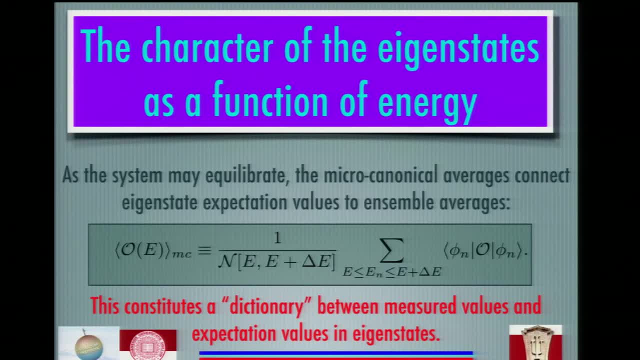 people have been asking themselves what happens if you take delta E to be equal to zero. regarding this so-called eigenstates hypothesis, We don't do this here, but basically this is, of course, what describes, as you all know, mechatronical ensemble. 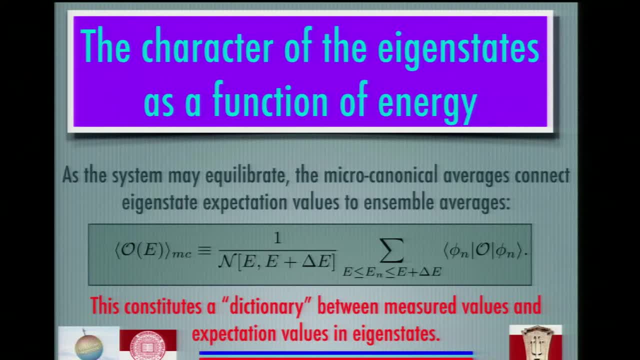 Any system in equilibrium- if it's not of too long range and so on- not pathological. what you actually measure in equilibrium will be equal to what you actually calculate here using this sum. Now, typically what we do is we evaluate the sum. 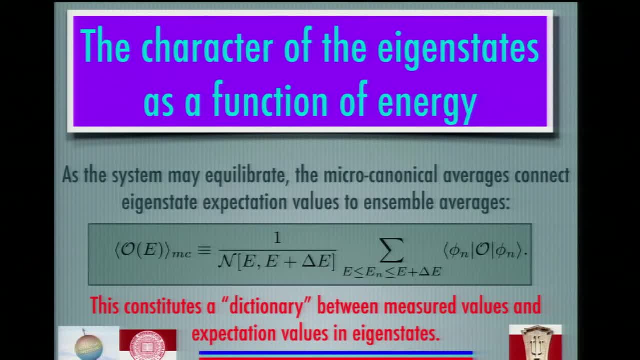 For some system we can actually solve like an ideal gas, harmonic ushers and so on. We get an answer Here. of course we cannot do that because we don't know what the eigenstates really are. We cannot write them down. 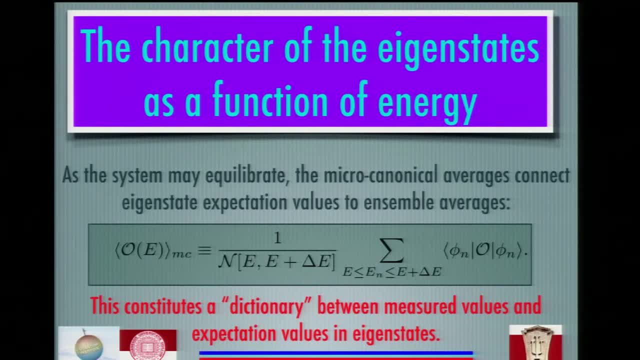 It's useless In some sense. But here we can actually use empirics. So empirically we know for this, Hamilton, I just wrote down for you earlier the sphere of everything. Empirically we know that all of these systems 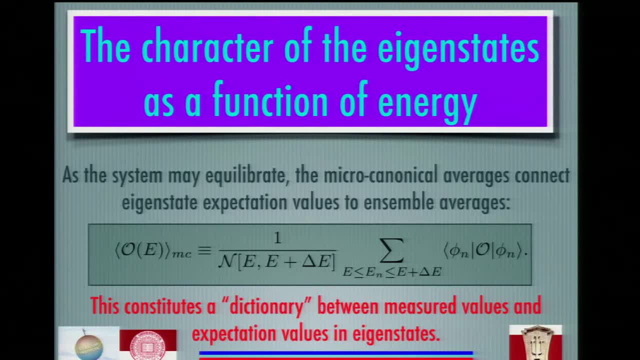 can be equilibrated if we don't actually quench them, By which I mean that if you actually measure them in equilibrium, what you actually measure for any quantity O you want to think about will correspond to this average. So this gives us sort of a dictionary. 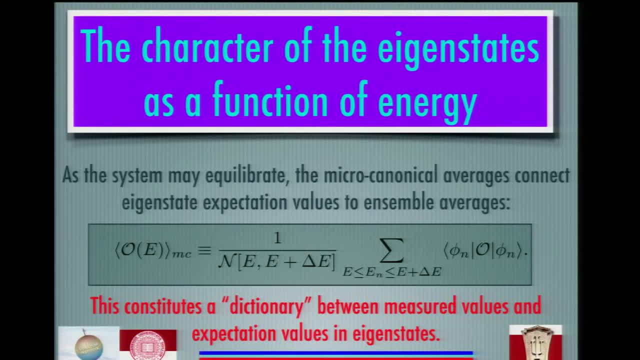 but looking at what happens to eigenstates, we cannot actually calculate relative to what we have from empirical observations. OK, Now we know, with high enough energy densities, when we're in a fluid phase empirically, but we measure a corresponding to a fluid phase. 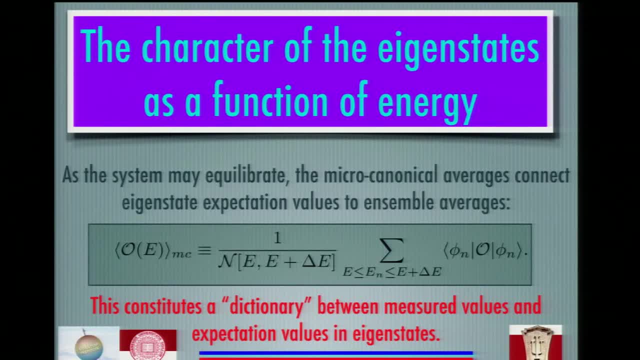 meaning that the eigenstates here, at these energy densities which are high enough, they give it features on average, because this is an average that I have here, on average corresponding to a fluid, And similarly, if I go to low enough energy densities, 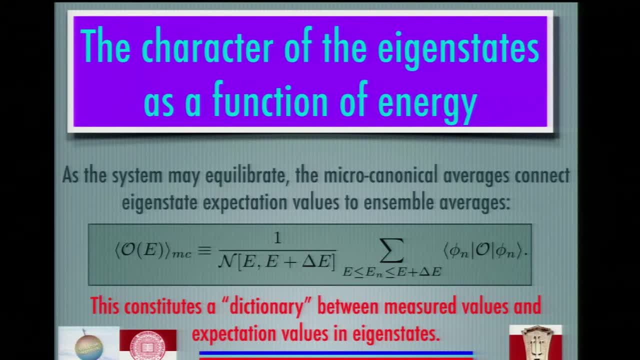 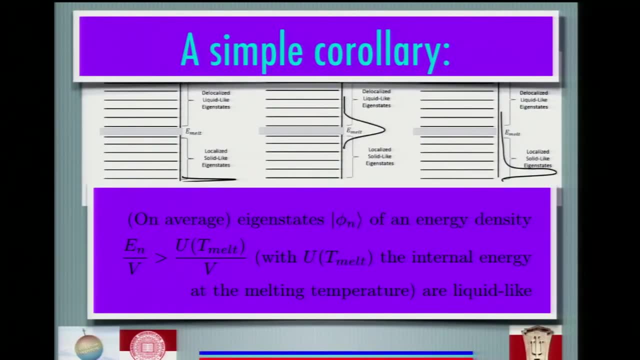 what I actually measure will be vat of the solid. Is this clear? This is with cartoon. So if I go into high enough energy densities up here I will have eigenstates that on average correspond to the fluid. If I go to low energy densities here, 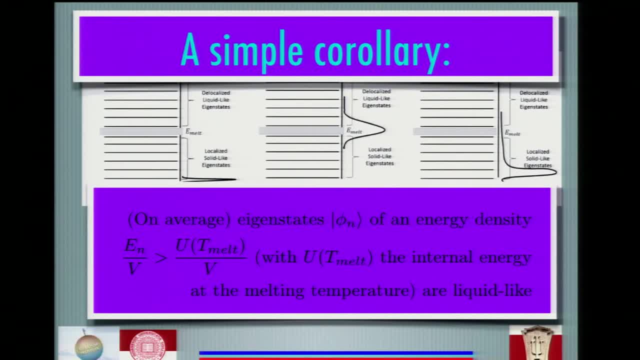 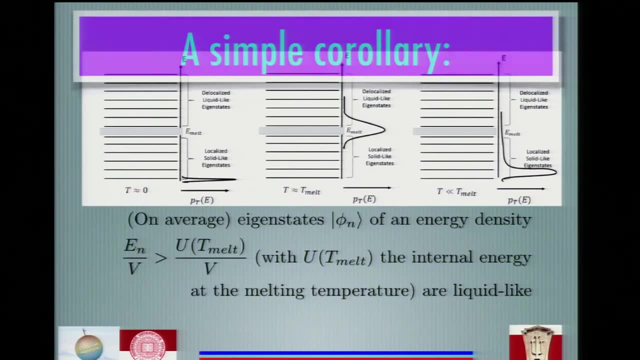 I'll have eigenstates that on average correspond to vat of the solid, And if I have latent heat, I will have eigenstates in that interval which will have mixed properties of both the fluid and the solid. OK, OK, and I should of course mention 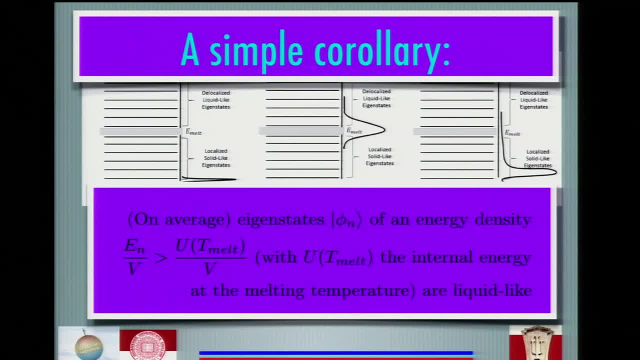 that, whatever you want to think about phonons, topological defects and so on- dislocations is an example, of course, All of these things that actually you can think about associating the solid type eigenstates, they all appear here OK. 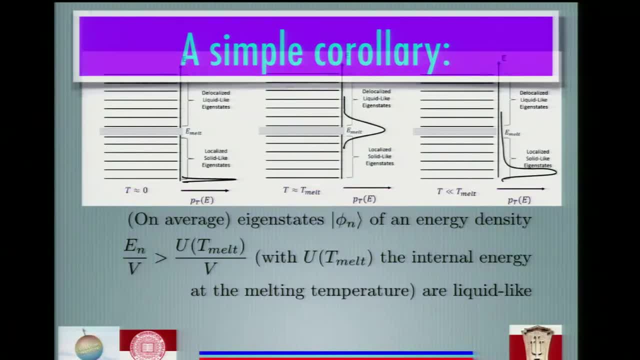 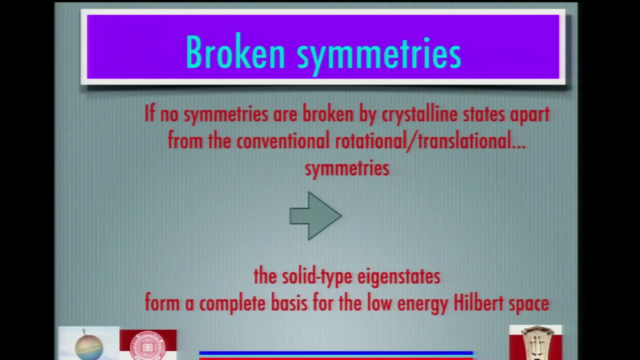 OK, OK, OK, OK. So if we believe, as we typically do believe, that crystals don't break any symmetries apart from the conventional ones like translations, rotations and so on, then that means that at low energy densities, 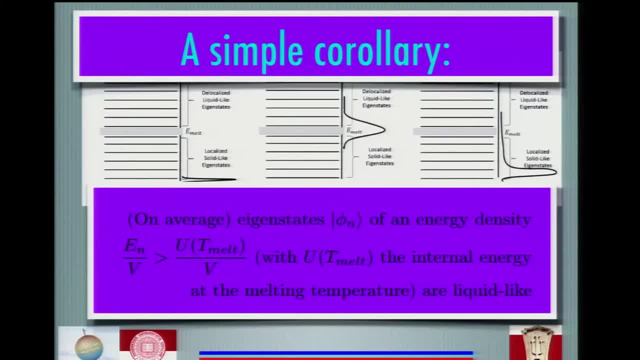 the full spectrum that we actually have, the one that I have here, all of these eigenstates that I have here at low energy densities, if I look at all possible, they all correspond to crystalline eigenstates. OK, Nothing else can appear because I 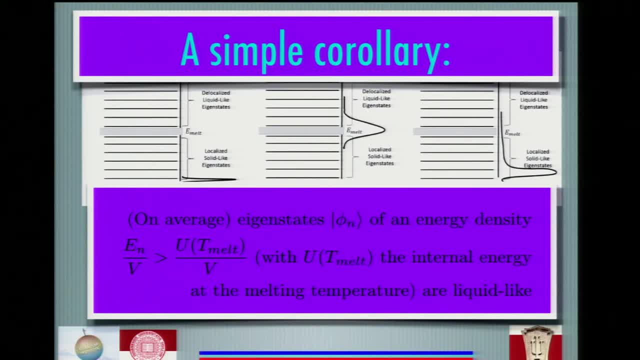 would have other eigenstates with a different character. I would have additional symmetries. I would actually have to break additional symmetries to actually get the crystal OK. so that means I can actually crystalline eigenstates. they span completely the space. 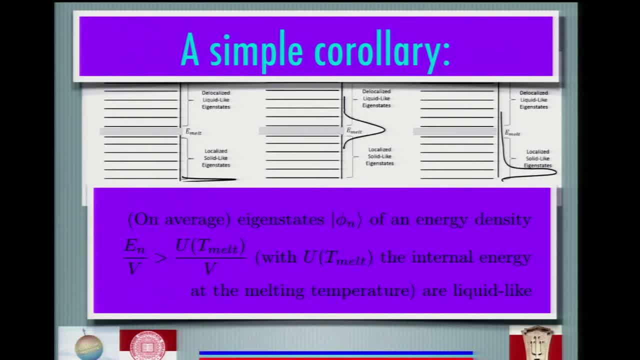 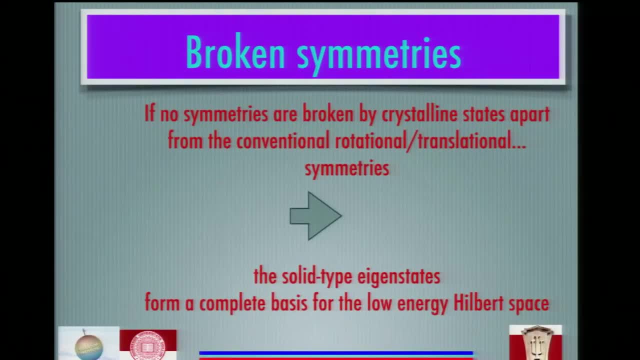 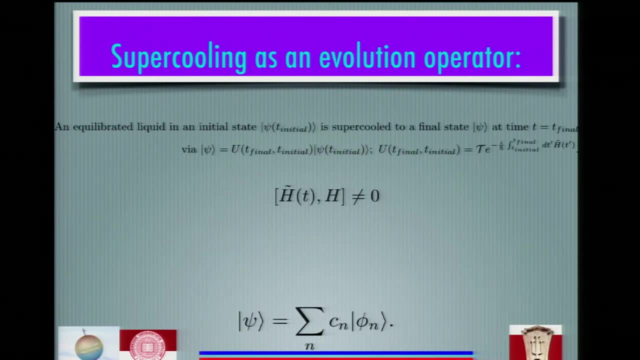 that I have at low energy. So now let's do a phi experiment. Suppose I start now at high temperatures and I cool the system down very, very quickly. OK, So I start off with some initial state. So this is psi initial. 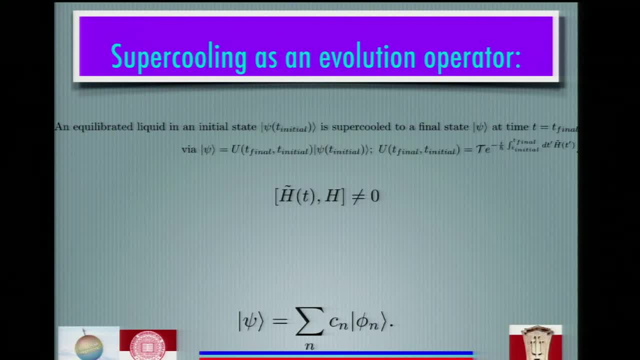 Psi initial corresponds to something which is close to an eigenstate, because if it were not close to an eigenstate I would have a mixture of different energy densities and I would actually get what I would compute in various ensembles And then I cool it down. 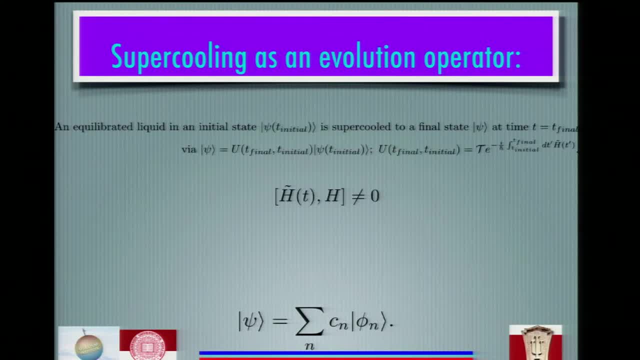 So I cool it down, I change my Hamiltonian in some particular way, It doesn't matter how I do it. So I have a mixture of different energy densities and I would actually get what I would compute in various ensembles. So I do it. 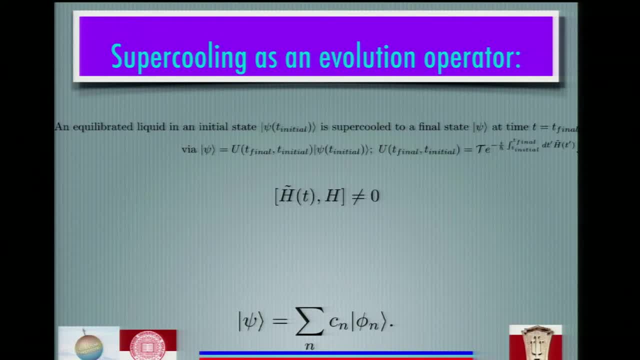 Energy goes down because whatever I do to it does not compute for Hamiltonian And the phi. energy density is actually now lower from what I had initially. Now, regardless of what I actually do, at the end of the day I have a new state psi. 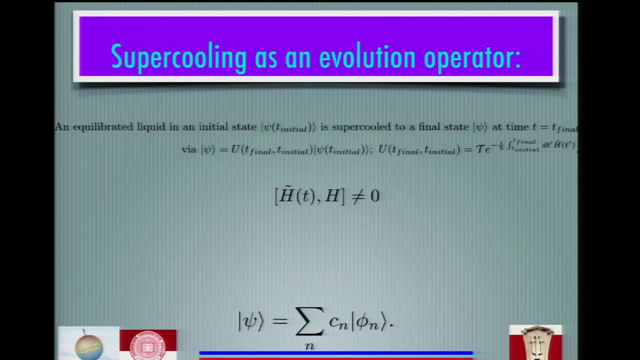 which I can actually expand on a complete eigenbasis of my Hamiltonian. OK Now, as I told you earlier, we obviously cannot calculate what these eigenstates really are, But we do know, as I just described to you in the last few minutes, that 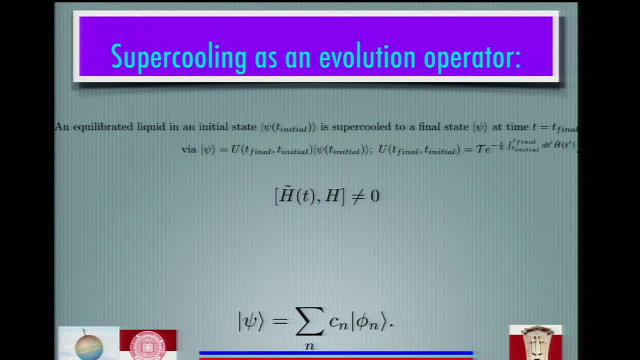 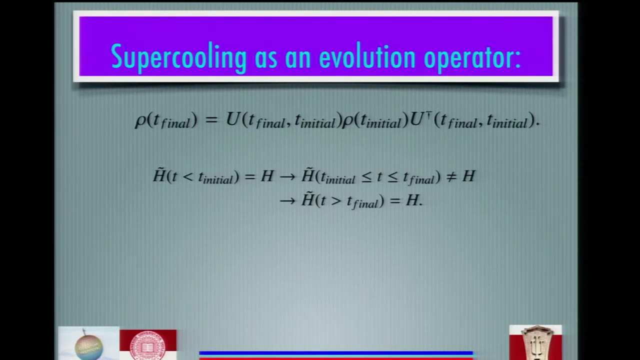 these states phi n. if I go to an energy density which are high enough, they correspond to the fluid. If I go to an energy density which are low enough, they correspond to the vat of the solid. OK, So now I can do the same thing if I have an open system. 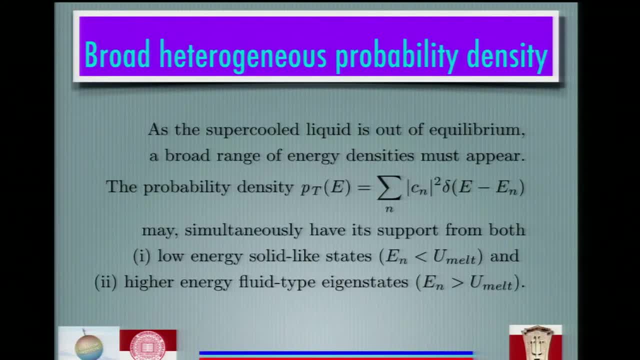 and so on. So I can do this anyway. This is sort of a general feature. So now, if I want to calculate the probability of having different energy densities that corresponds to this sum here. This is a probability If I have a temperature T, final temperature T. 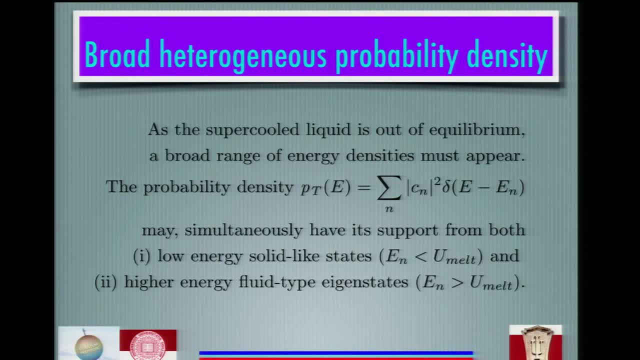 I have an energy E, So it's basically, of course, the sum of a moduli squared that I have of all states that have an energy E. Yeah, So yeah, I was going to say: why do you think you need to make the unitary operator? 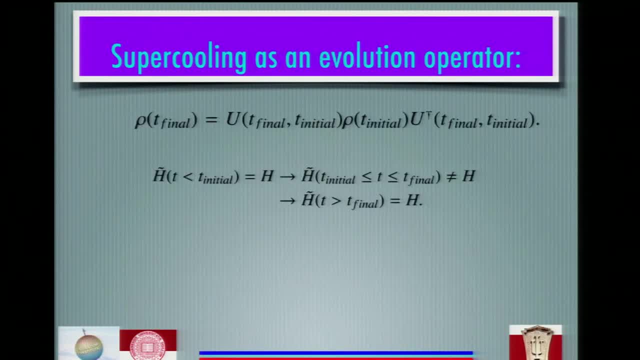 Yeah, so you can do it in a variety of ways. So you can think about also the unitary operator in some ways. But the unitary operator obviously does not commute to the Hamiltonian, Because if it were to commute to Hamiltonian, of course, 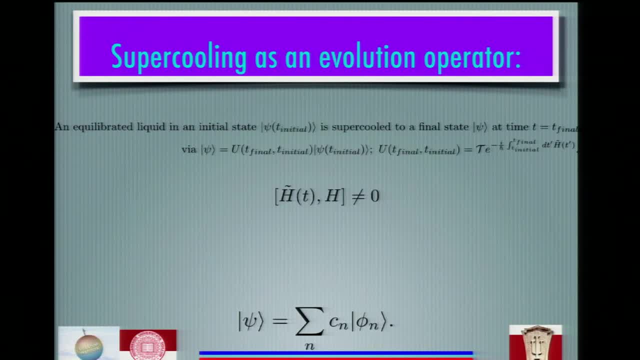 energy would not change. So whatever I have here, this h twiddle doesn't commute to h, So the energy goes down. Energy is measured by the Hamiltonian itself. h goes down because this h twiddle doesn't commute to h itself. 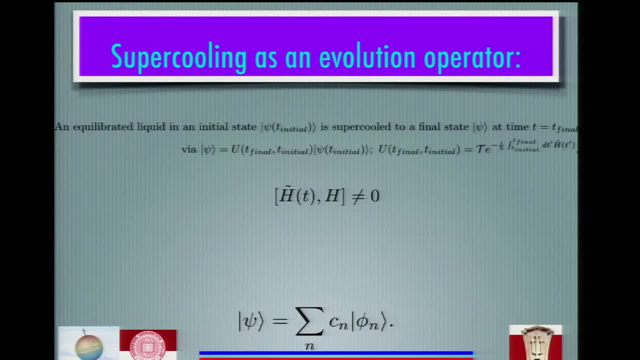 So I can think about the system plus its environment as one big system and which is the closed system, And I can write it this way. But it doesn't really matter. Whatever I actually do with my system, I can write down my full state in the eigenbasis. 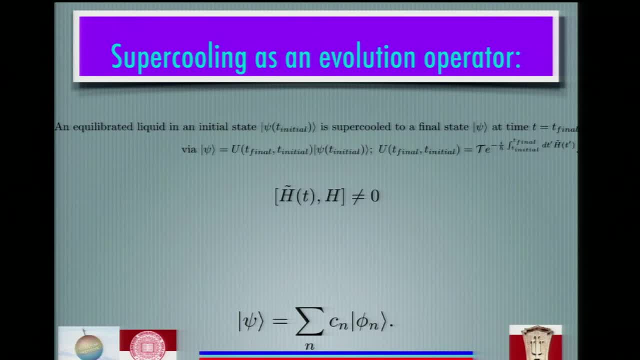 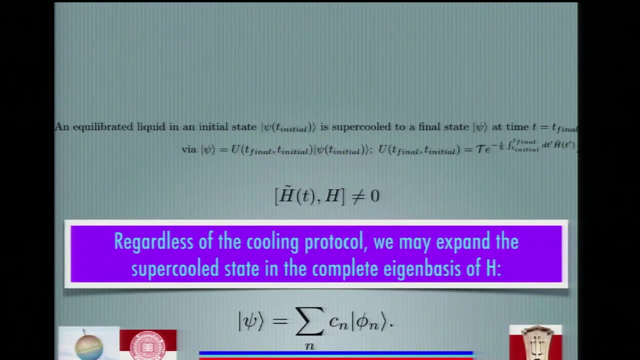 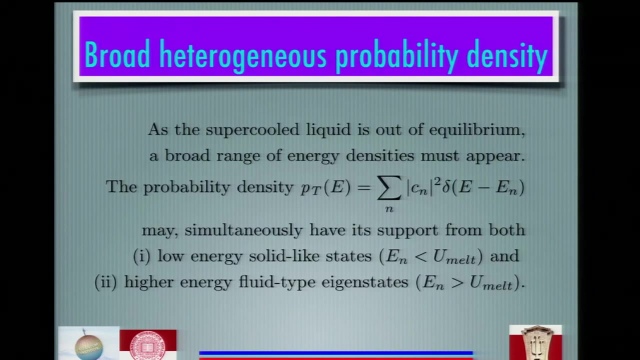 span by all these eigenstates that I have in the Hamiltonian, Because they're a complete set of states, OK, OK, So, as I just mentioned in this sum here, in this probability that I have here of finding different states of various energies, 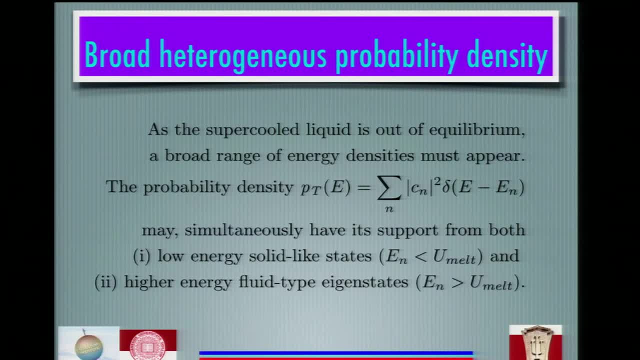 some energies will correspond to that. Some states will correspond to that of a solid- If energy is lower than that of a system, it's melting- And some will correspond by the fluid. So here in general I have a mixture. So when I write down, when I decompose my state, 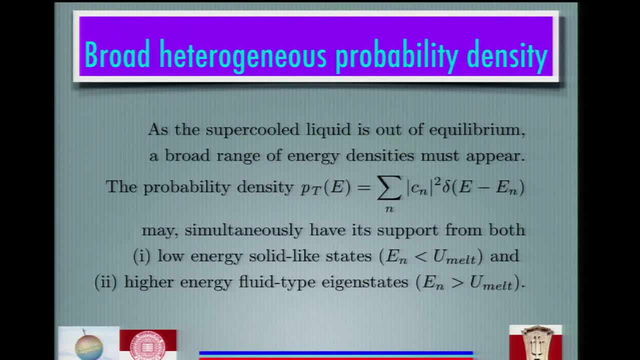 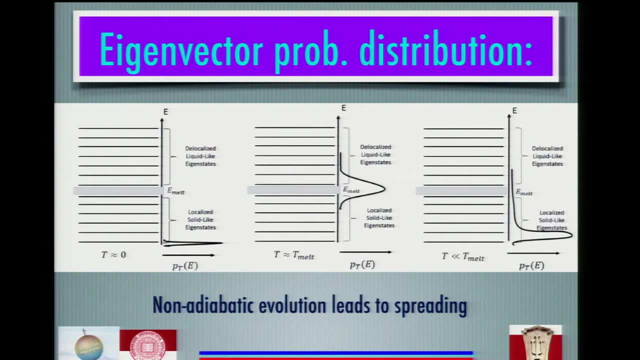 in the eigenbasis of Hamilton I have a mixture of states which are partially fluid and partially solid, So here is a cartoon of what actually happens. So imagine I start off initially at high temperatures somewhere up here, somewhere in these eigenstates right here. 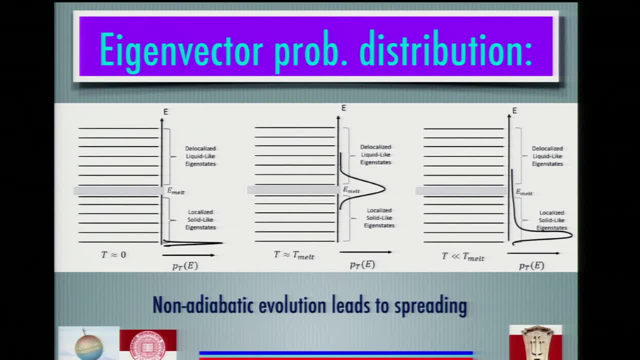 I cool down very, very quickly Because I do it Not adiabatically, I do it very, very quickly. I don't stay close to any eigenstates And in general I will have some spreading. So as I cool down I will have the distribution. 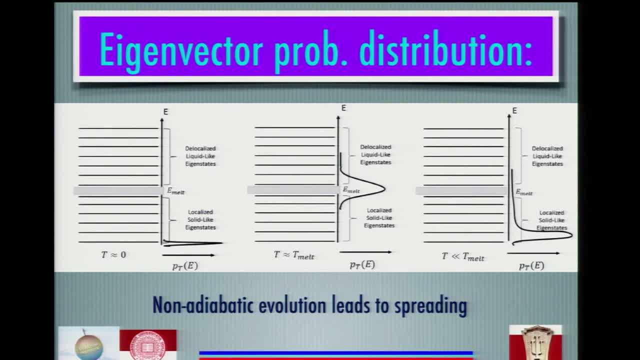 I just alluded to, of a probability of finding different energies. E will look something like this: So we'll span both states' high energies and states' low energies, So we'll have both components which should behave like a fluid and the components which behave like a solid. 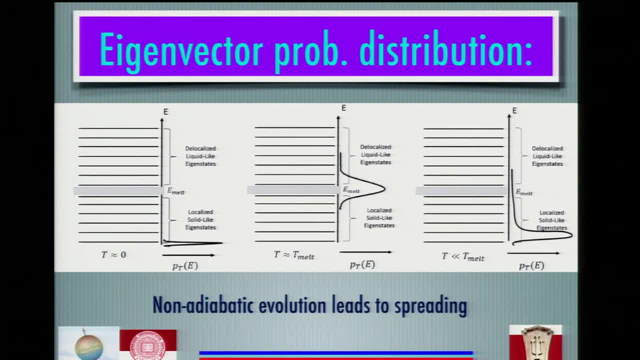 As I cool down more and more and more the center of mass of this distribution, so to speak, goes down. So overall the average energy density goes down, But in general there will always be some fine probability of having arbitrary high energy. 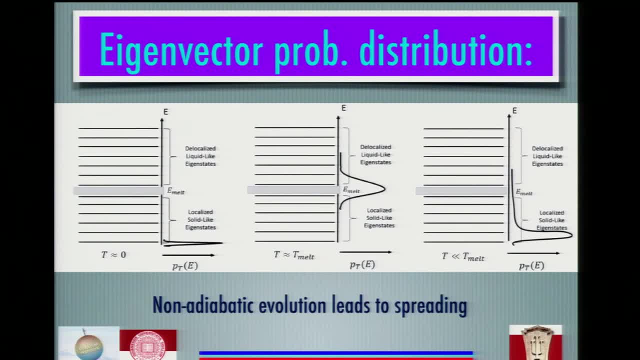 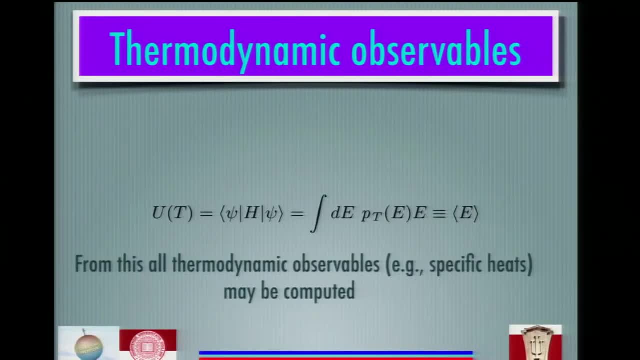 there. Now, of course, you can calculate whatever you want to measure, So you can calculate the energy itself. That's of course easy to do And you can: Sorry, Sorry, And from that you can, of course. 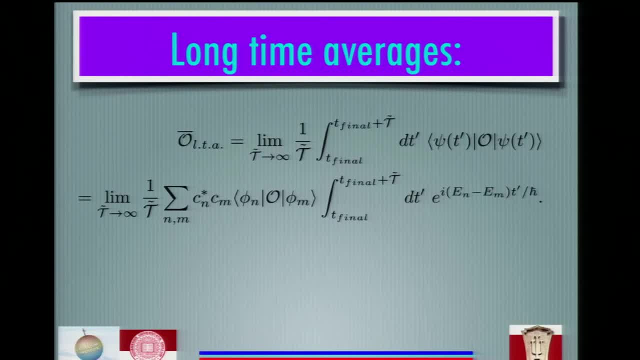 calculate any quantity, of heat capacity and so on, And you can also calculate slightly more involved quantities, like, for instance, viscosity, in a very, very simple way. So if you consider any quantity, you only want to think about and look at its long-time average. 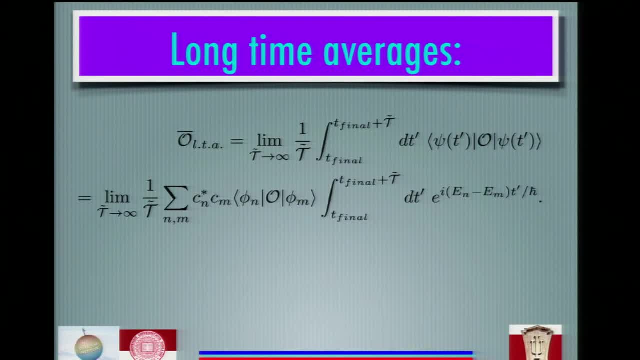 So LTA here stands for the long-time average of any observable O. What does it correspond to? By definition, it corresponds to the value of O that you have at time, t prime. So it's the value of time from initial time to the final time. 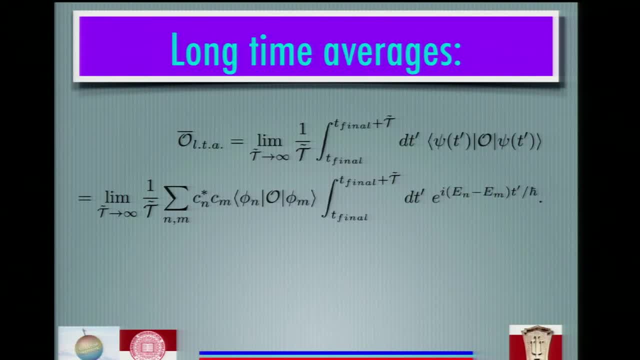 And you make this window of times arbitrary or large and you average over it. Now again, you can write down these states that I have here, this psi of t's. You can write down them in the complete eigenbasis of the Hamiltonian. 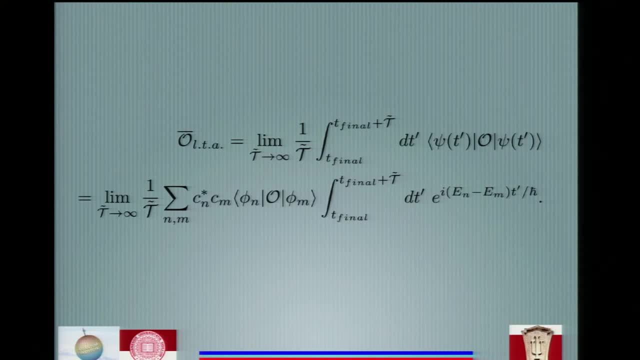 So you have these amplitudes here, And so what you have ultimately, as you can sort of see- and this is of course the conventional calculations- very, very simple- is just the metric element you have observed between different eigenstates of the Hamiltonian. 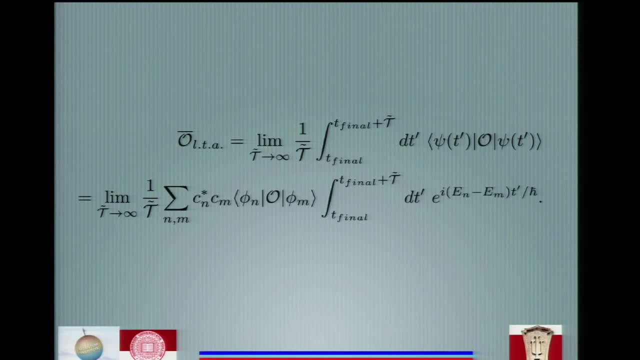 Multiplied by these amplitudes of being in these different states, Multiplied crucially by this integral that I have over time of eta pi i: the energy that I have at state n minus energy that I have at state m, times t prime over h. 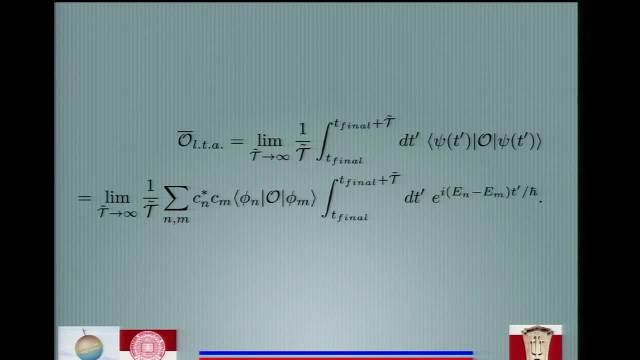 bar. Now, as I look at long-time average, when I take this time here to be infinite, this integral will become the delta function. So basically it enforces that En is equal to Em. so ultimately what I have are just diagonal elements. 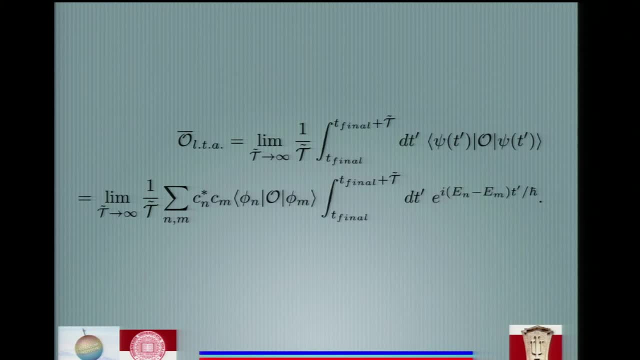 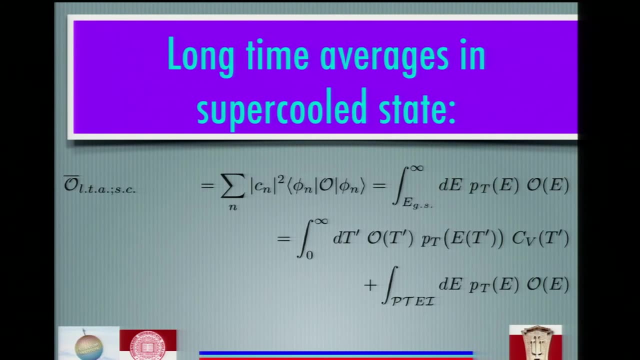 So the long-time average I have with any quantity ultimately just corresponds to a sum of diagonal elements. So I can write this down as the sum of diagonal elements. So basically it just corresponds to probability being in different states times, what actually I will measure in those states. 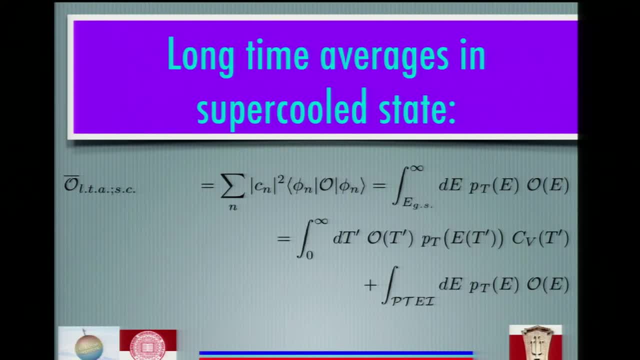 Now I can convert this, of course, into this integral over these energies I told you about. It was probability distribution. I had told you earlier Of having this pt of e, the probability of being at state e, the temperature of t at the end. 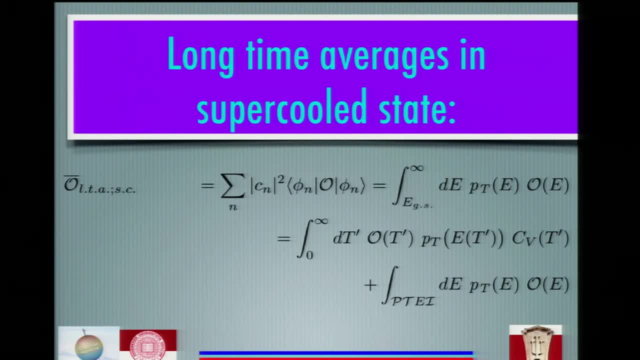 This is just basically just writing down what these are in a continuum Multiplied by the average value of o in equilibrium, Because, remember, the average value of o over eigenstates, over a narrow energy window, just is not nothing else but the equilibrium average value. 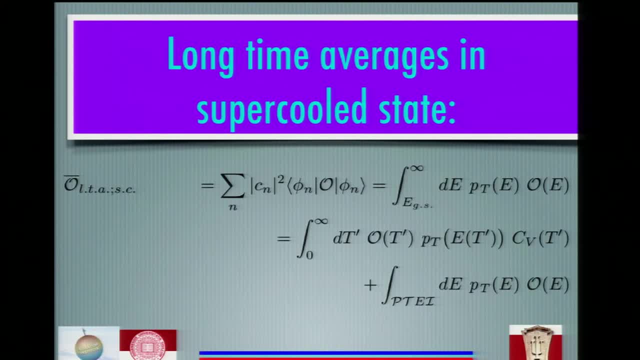 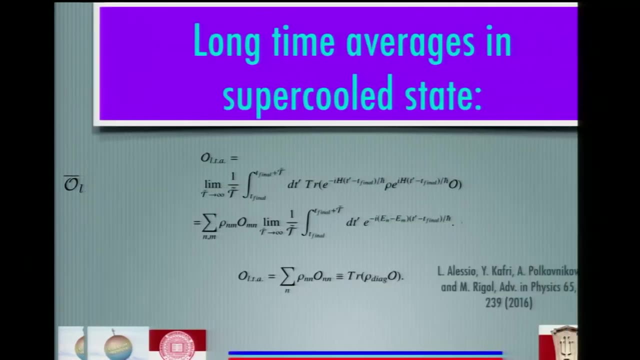 that you have of o at an energy itself. So you can write down a long-time average of any quantity you want to think about As what you have in the equilibrium, weighted by some probability distribution, And you can do this also more and more involved. 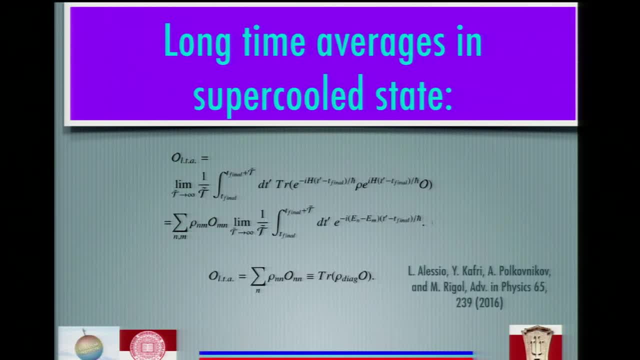 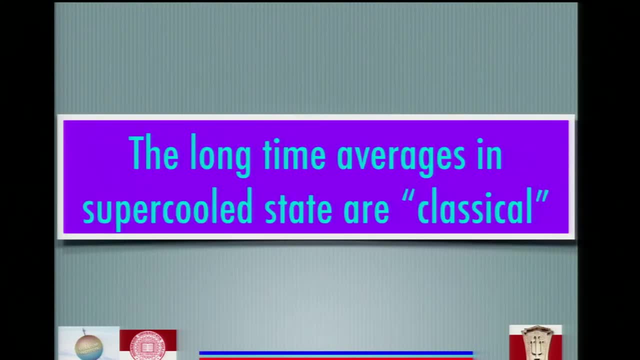 if you have a density matrix and so on. So the same idea, of course, will apply there. So now you can actually mention, of course, that all these averages that we alluded to earlier, all these that I have here and if I have additional quantum, 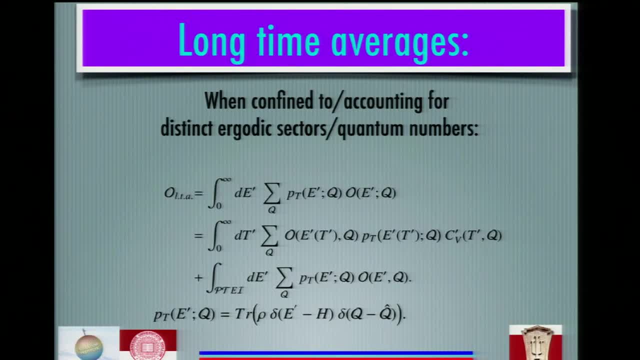 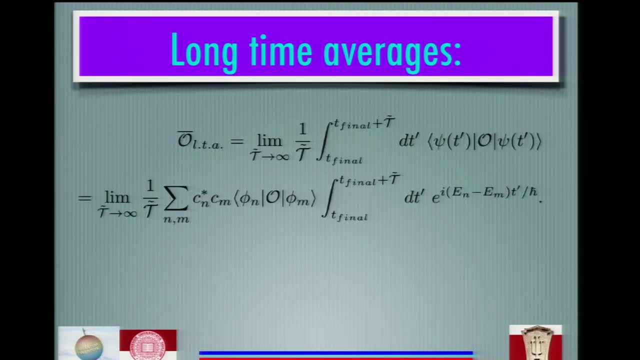 numbers and so on. They're all, in the end, classical. So even though I put in the h-bar, in the end h-bar disappears. So I had an h-bar here, But because this enforced a delta function, this becomes a delta function in the end. 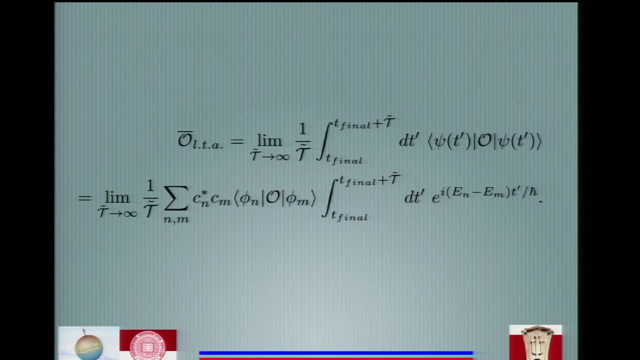 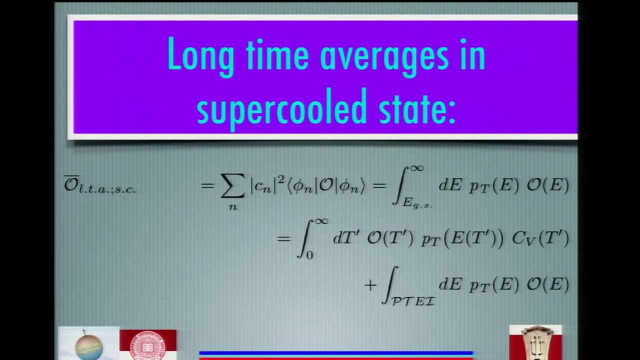 the final answer I had here had absolutely no reminiscence of h-bar. There's no h-bar that appears in the final answer Here. there's no h-bar. It's basically like a classical average. So a long-time average is that of what? 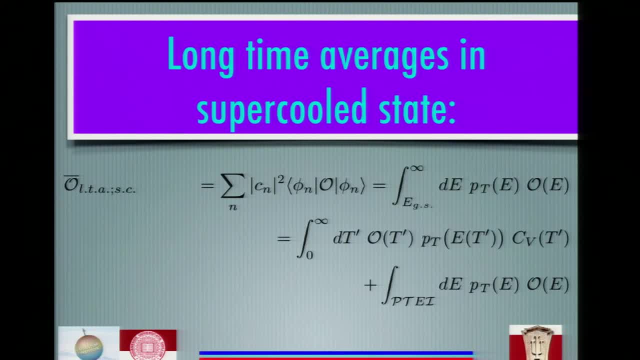 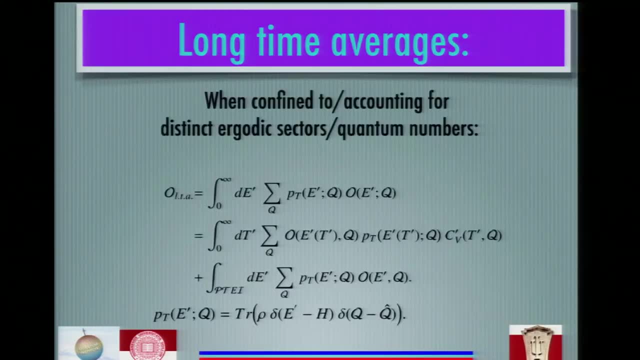 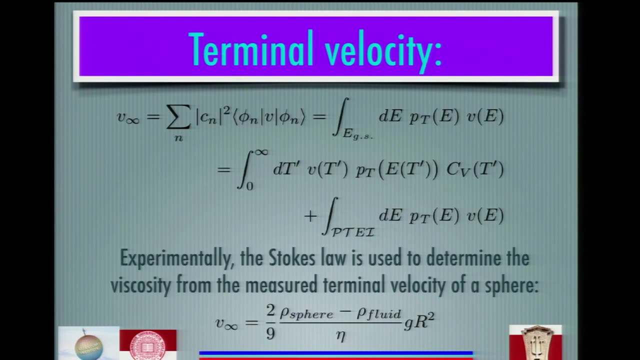 I have in the equilibrium multiplied by weights, And there's no h-bar. So it's quite intuitive. of course It's not terribly surprising. So now let's calculate the viscosity, And let's not do this usually in a conventional way. 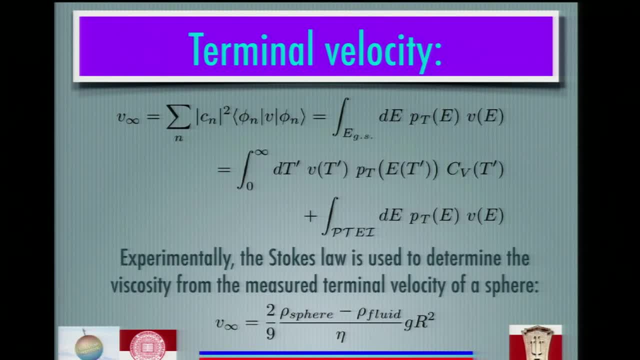 using a group, of formalism and so on. Let's just do it in a much simpler way. So let's imagine how we actually measure it When you measure viscosity. there are many ways of measuring viscosity, But one of the oldest ways of measuring viscosity- 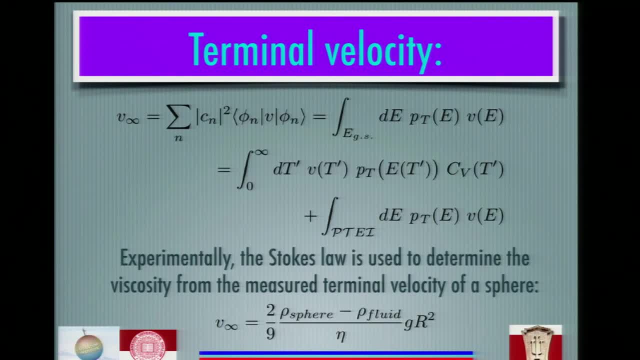 is taking a bucket or whatever you actually have with a fluid that you want to measure its viscosity. Take a sphere of radius r, plunge it into this bucket and measure its terminal velocity. Terminal velocity by Stokes' law is equal to some constants. 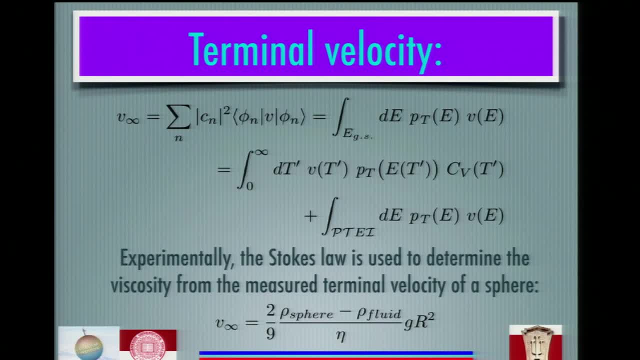 This is just radius that you have of your sphere and so on. It's acceleration of free fall, the difference of densities and so on Divide crucially by viscosity itself. So if you know the terminal velocity, if you know the long-term average of velocity, 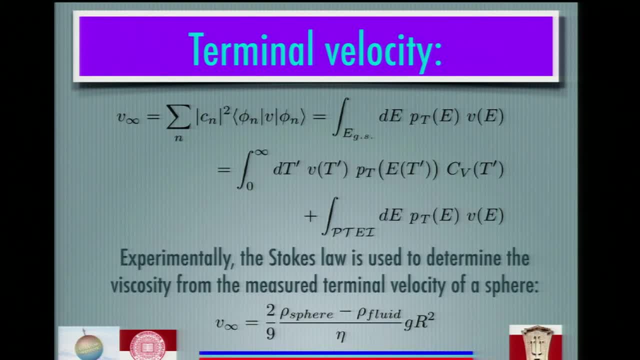 you can infer from that viscosity. That's the oldest way of actually measuring it, One of the oldest ways of measuring viscosity itself. So what we'll do right now is we'll actually calculate what this long-term average is And from that infer what the viscosity. 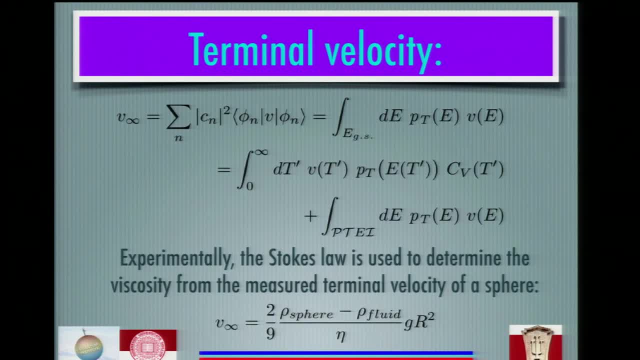 is again a prediction, And we'll calculate this average by just using the equation I just derived for you earlier, the stripple equation I derived for you, in which I wrote down the long-term average of the velocity or any quantity as what I have- velocity. 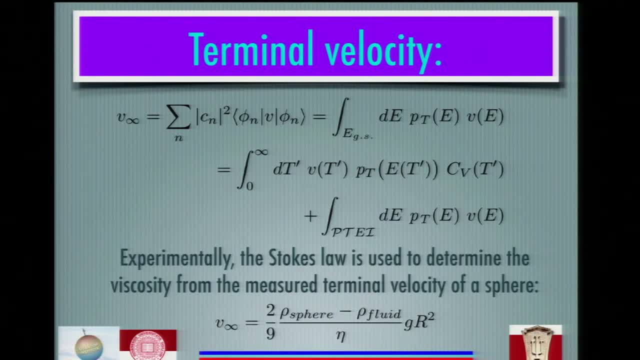 in equilibrium at energy, meaning at temperature T corresponding to a particular energy density, E itself, and multiply with this probability distribution. So this I know from measurements. I can measure it in equilibrium with the terminal velocities of a sphere falling down in a bucket at a temperature T. 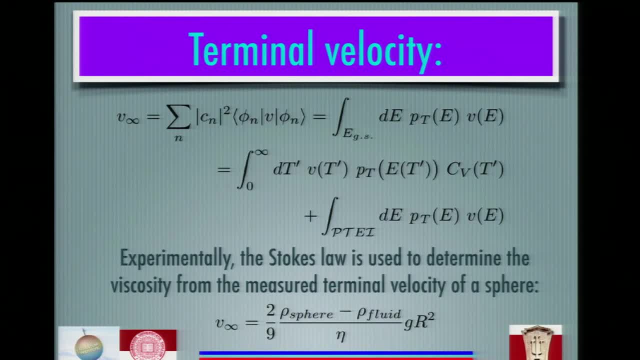 or energy E, And I can multiply that with this probability distribution, do an integral and get the answer. Once I have this, I can plug that in here and calculate the viscosity. So everything is known, so to speak, The only thing that's unknown here so far. I'm not cheating. 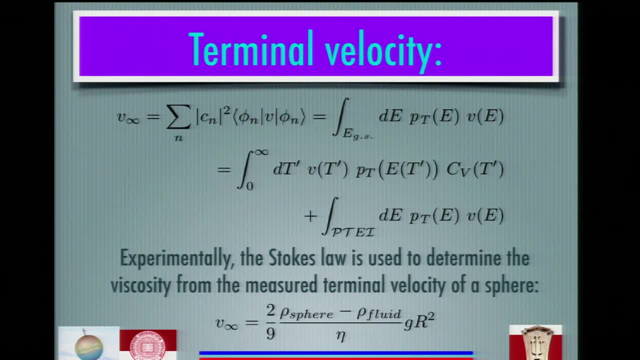 This is a general expression. The only thing that's not known here is, of course, is this distribution, this function, Pt of E. Of course, the function contains the infinite number parameter, of course, So you might say you can always fit any quantity, you. 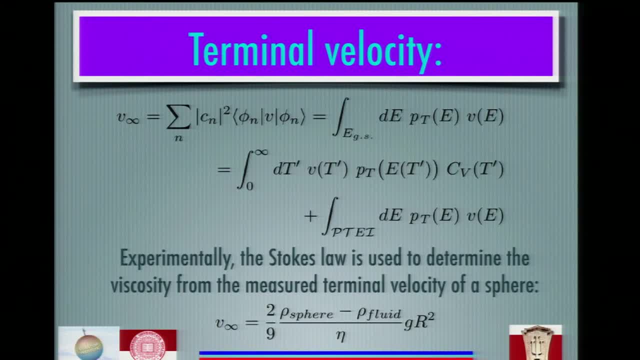 want to fit to this form because, of course, you can always design a function Pt of E that will do the job. That's not terribly surprising. So what we'll try to do is actually try to find out what's the most natural functional form. 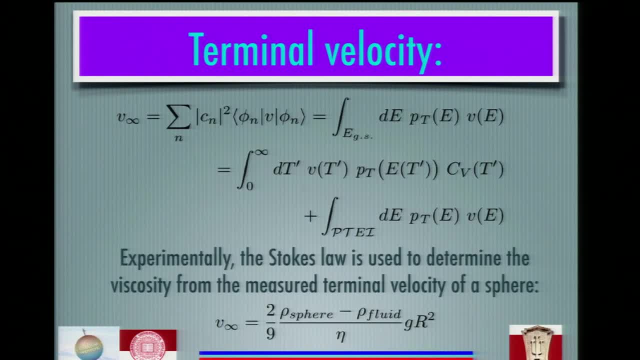 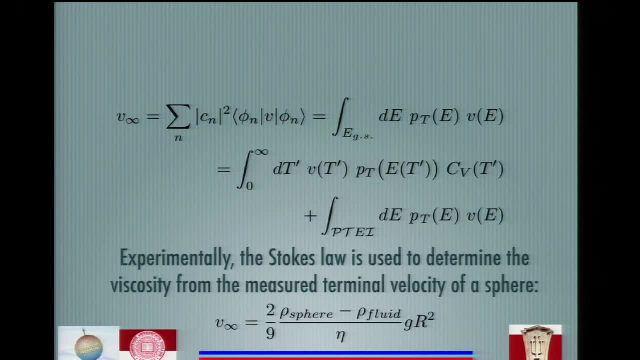 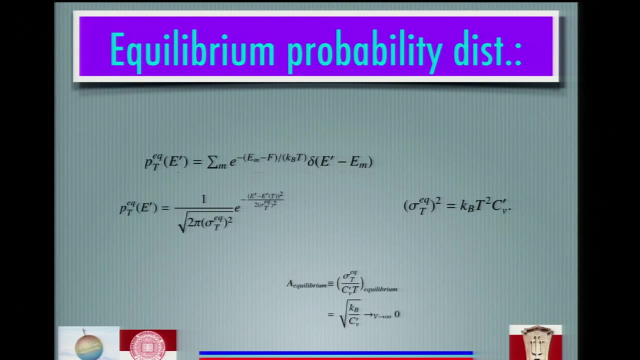 The form that we'll have for this distribution. What should I plug in here for this distribution? I have Pt of E, So to that end we'll just use simple principles. So, as you know, in equilibrium, if I write down the probability of attaining a particular energy density, E, 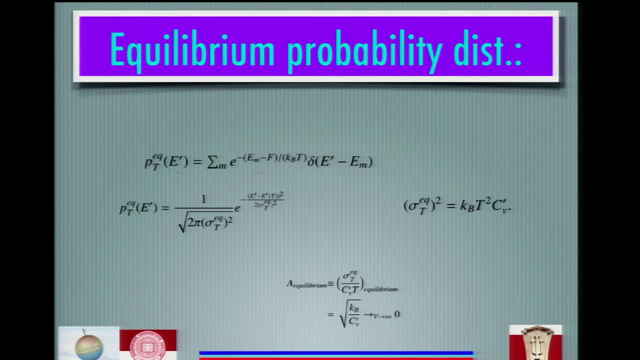 prime. it corresponds to a Gaussian whose width is set by heat capacity itself. heat capacity, constant volume times temperature squared, So it's basically proportional. The standard deviation is proportional to the temperature times, the square root of n? n being system size. 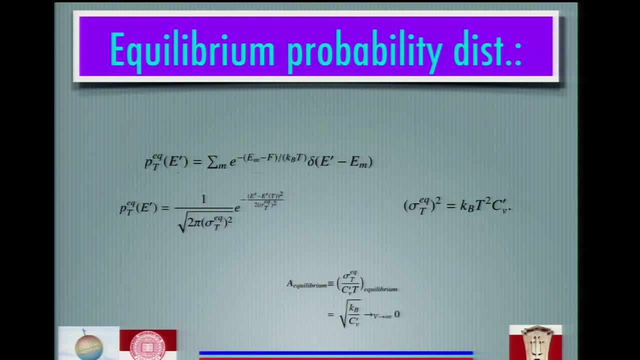 because of course, heat capacity, of course, is extensive quantity. So here, in the conventional case, I think about the width for my distribution, That width, the standard deviation divided by energy scale, that goes to zero in the 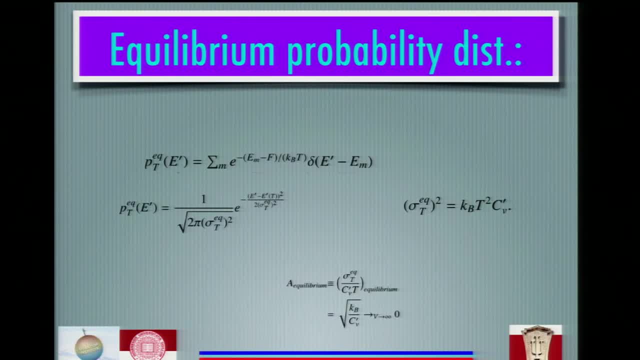 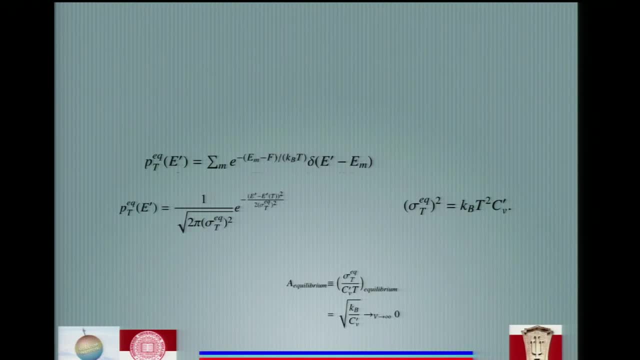 I have 1 over square root of n fluctuations. The energy density is a very well-defined quantity. Now, in our case, that obviously is not going to happen, Because if it would happen, we would just regain the usual results of equilibrium-specific mechanics. 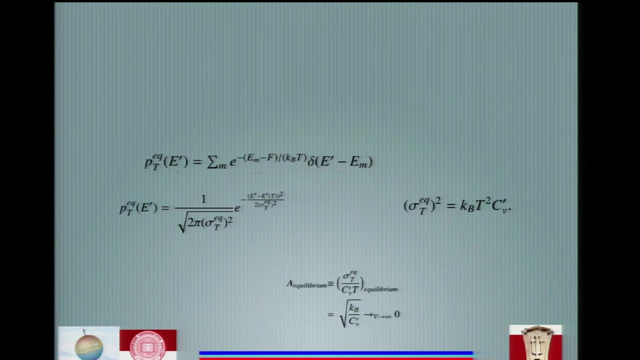 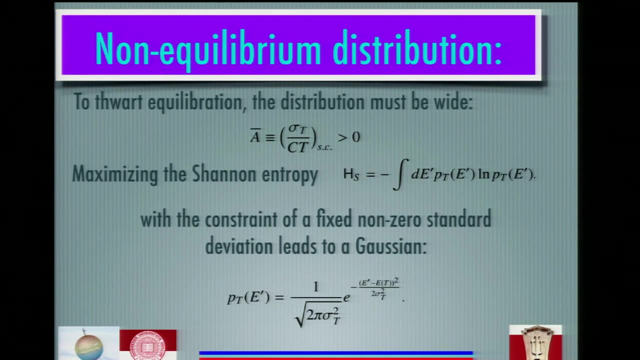 And we don't. What you actually measure in the superglue fluid is not what you actually get in equilibrium. So obviously this distribution cannot hold anymore. So what we should do is we actually should try to maximize the Shannon entropy written here for a probability distribution and ask ourselves: 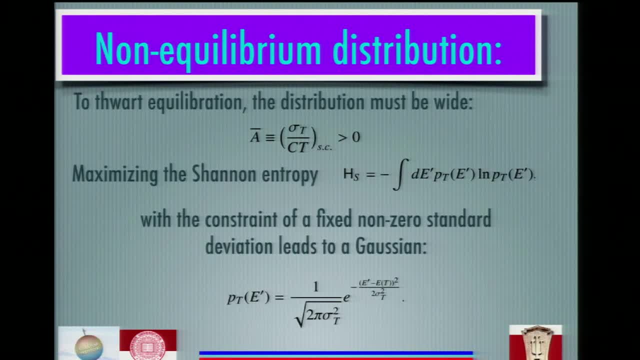 what's the most likely probability distribution that we'll have here? Pt of E prime that maximizes the entropy, with a condition that has a fixed variance. The variance cannot be 0, because if the variance were 0, I would just get as I just mentioned now. 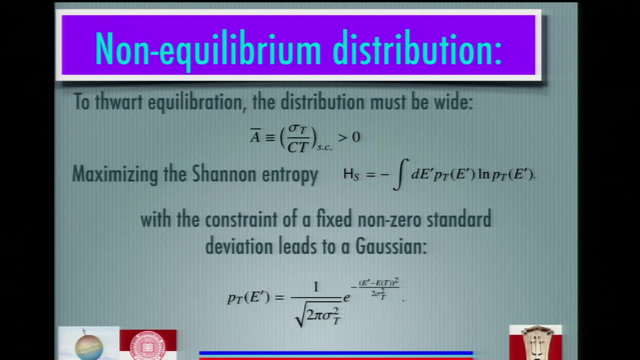 I would just re-derive what I had in equilibrium and obviously the results I get should be different from equilibrium. So I should have a finite width sigma and I should just maximize this entropy And, of course, as you know, or you? 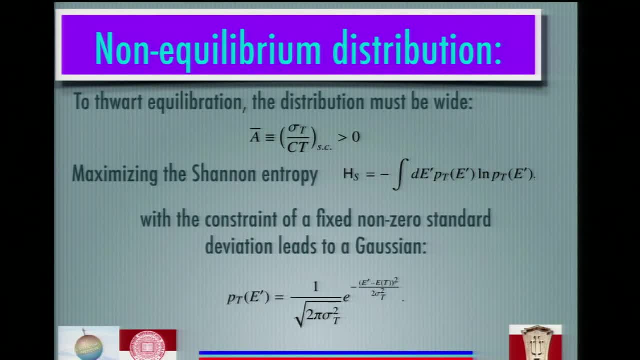 can just do some calculation with the Gauntlet multipliers if you want to maximize the entropy with a constraint of fixed variance. So if you have a fixed variance, what you get is a Gaussian. So we'll have some Gaussian who's centered about what you have at temperature T itself. 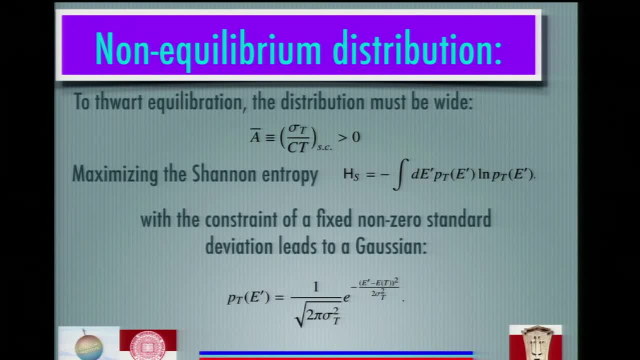 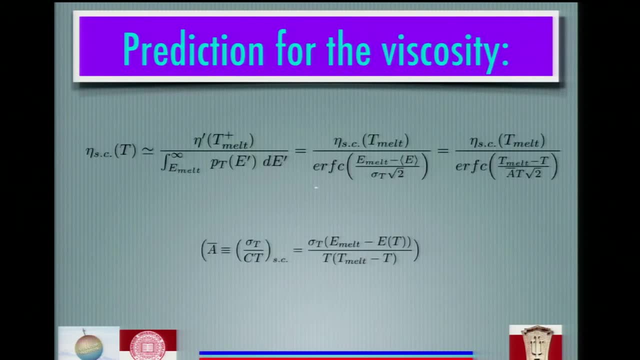 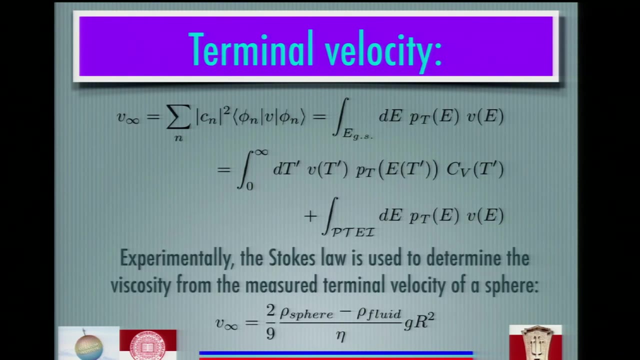 temperature T itself with some fine distribution. Now we can take this functional form of the Gaussian and we can plug it in back into this form I just told you about earlier. We can plug it in this equation here, here, with the top line that you can see here is integral. 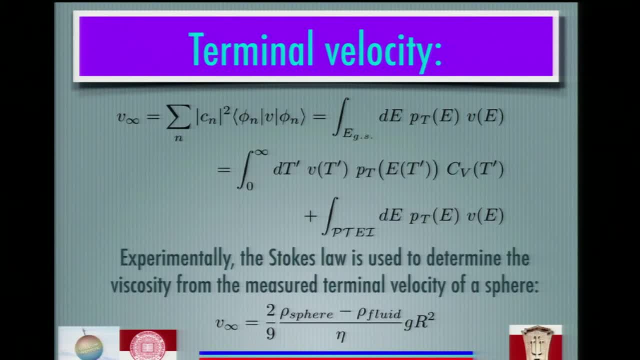 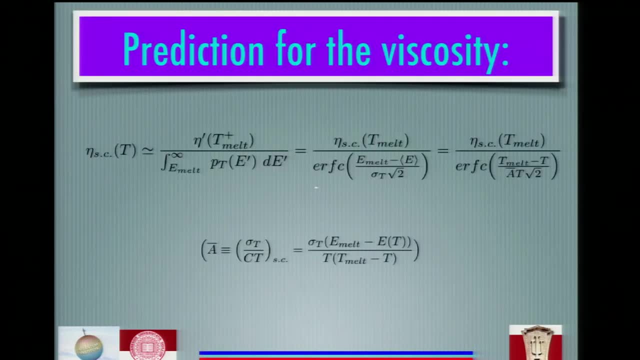 We can do the integral and find out the result, And that's what's schematically sketched here. So we can just plug that in And the integral. of course, this integral for a Gaussian is trivial. It's an error function, a couple of error function. 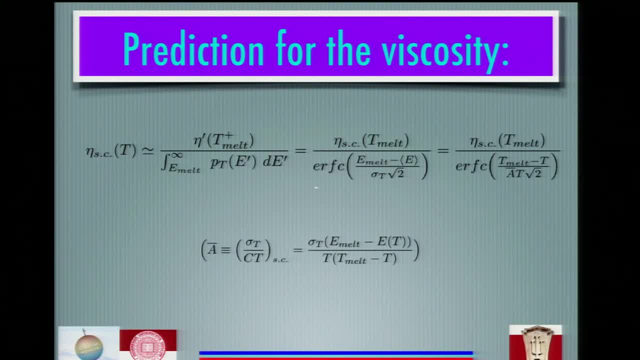 So the prediction would be, using these considerations, that the viscosity at temperature T for a supercooled fluid behaves as what I have at melting, divided by this couple of error function of how far away I am from melting the difference, And then we can divide by temperature itself. 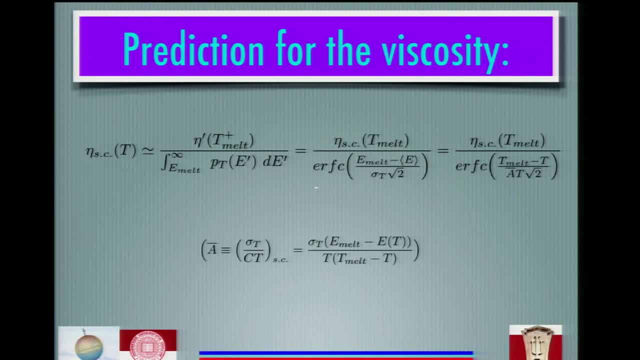 And I converted the standard deviations, still divided by temperature scale. I've just dominated the quantity. So basically the only one dimensional scale. The width of the Gaussian is proportional to energy itself. OK, So that's a prediction itself. That's how we derive it in the first. 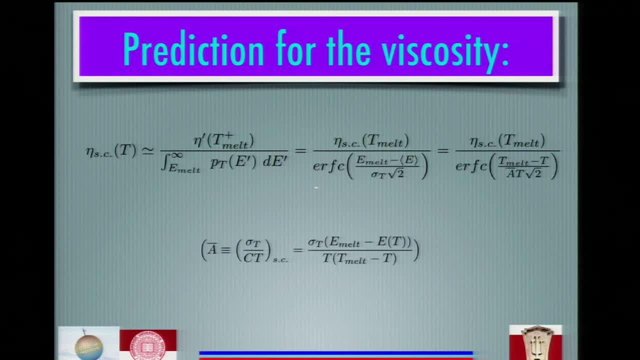 I can, of course, check to see how this thing works, And that actually works pretty well. That's what I showed in the beginning of the lecture. So now we can actually go and see how it works. So this is ultra-fennel, one of these fluids. 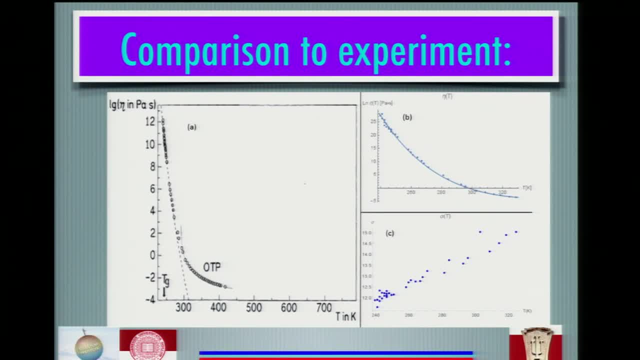 that has deviates the most from we need to begin with. so that's the idea, Uh-huh behavior. okay, this is raw data themselves, and you can fit quite well to this form with only one parameter, but of course, one fluid by itself is only one system. not terribly surprising you. 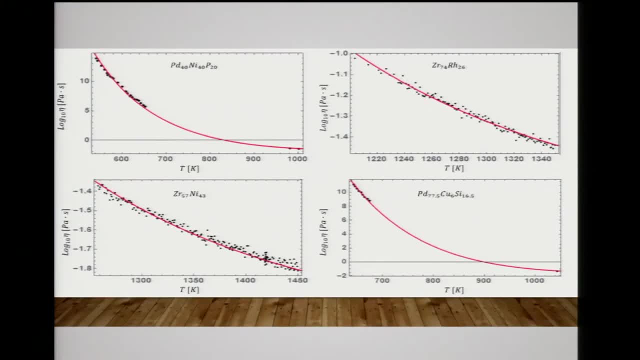 might say. so you can do this for all fluids where we look that which have literature into open data, some data which actually not published because of proprietary, but over there published. we can, we try to fit them and we got the same results. so basically, here are some metallic fluids and 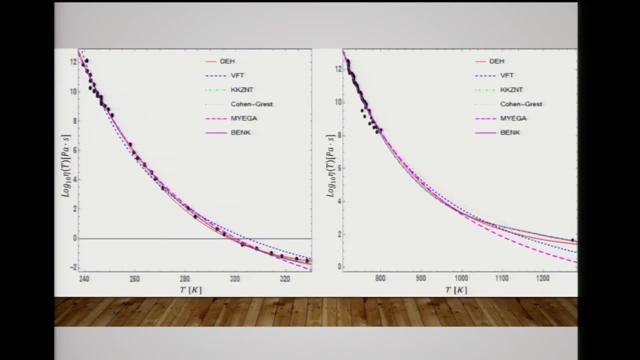 so on other fluids, water, okay, so all of them. basically they all collapse into this. they all work pretty well and in fact this works much better than this mobile folder form. so this mobile folder is this dashed curve here. the second one is VFT. it doesn't work, very, very. 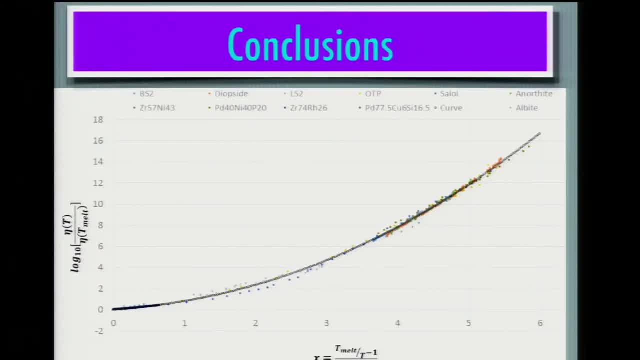 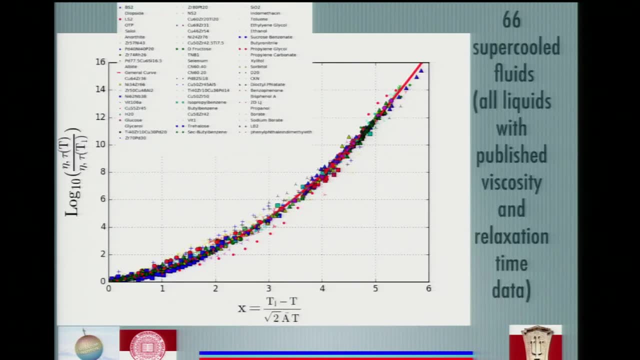 well, and you can do this, for here's a small sample of fluids. you can do it for more fluids. okay, there were six, six, six six of those are short at the beginning. so basically seems to work pretty well, this curve. here. the red line is this integral- I showed you this error function, one of its complementary area function and all. 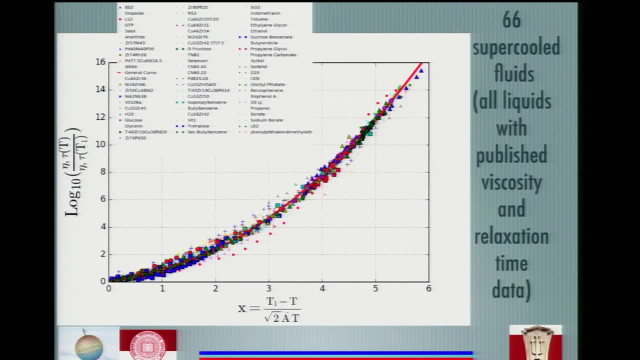 the other day. all other points are just raw data. okay, and the only parameter in this problem is a bar, and it doesn't change that much. as I told you, it varies from about 0.06 to 0.12 and it really doesn't change that much- on average of fluid to fluid and in fact, this quantity right here is a. 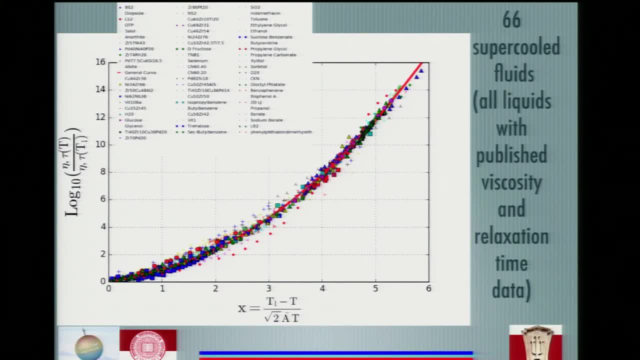 bar actually has physical meaning because, as you can sort of see from the my earlier sketches, I assume they have some probably distribution and a bar was the width for this distribution. so the more the larger the value of a bar is, the larger the more influences of low energy states- you will feel them already- at kind of higher energies because their distribution 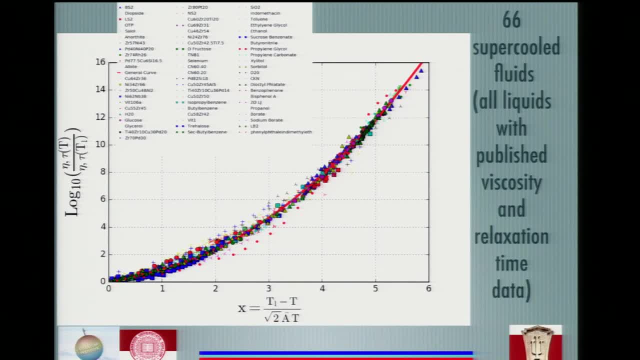 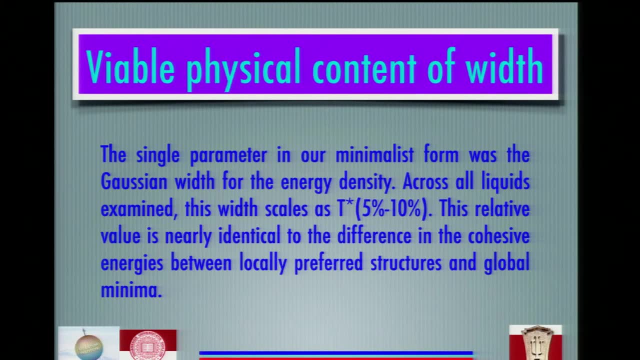 is wider, so it deviates from Arrhenius already at high temperatures. so basically, and I just alluded to now the width that would he have, basically scales at five or ten degrees, and then the percent that I have was of his Gaussian and if I actually look at what I have for various, if I do, 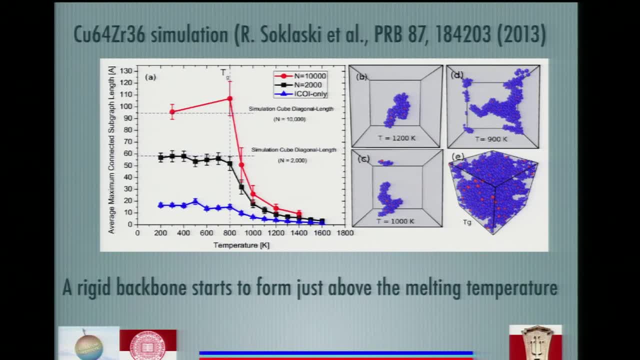 simulations, for instance- and I try to see what happens- various temperatures. we see what we did here. you can sort of see that something starts to happen just above melting and just above actually with this. it seems to coincide with this parameter, emissions parameter that I have now they're. 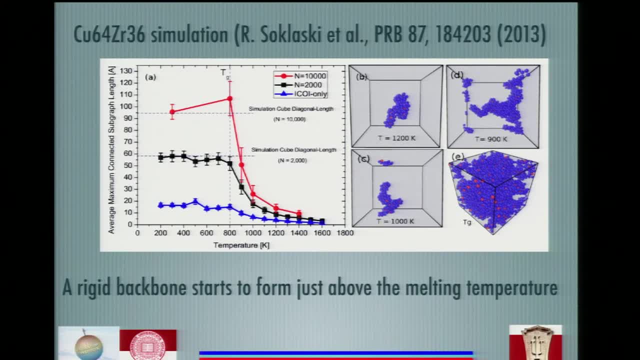 basically this parameter determining the width of that, of this, of this Gaussian. so if you just go a little bit above melting for the system, this here are the spanning clusters. we actually find these stable clusters. they start to appear exactly above melting and the system starts to become. 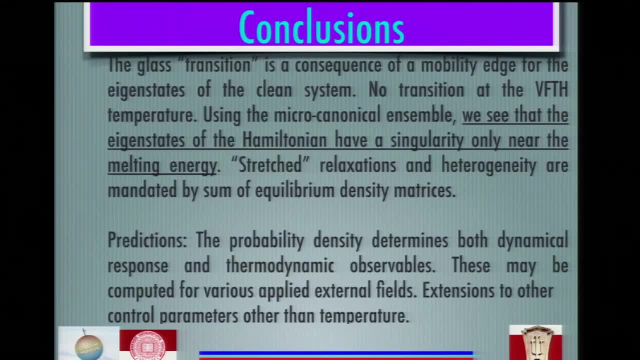 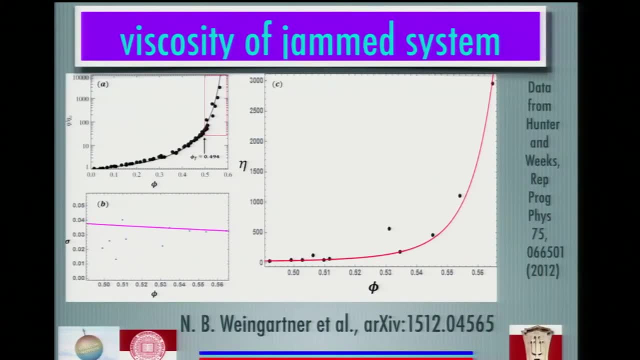 rigid and so on, above melting. so I guess I probably should stop here. about a baby, I just say one more thing. I just alluded to it, so just as a, we just jump to the very end of something I wanted to say earlier. I apologize for this. 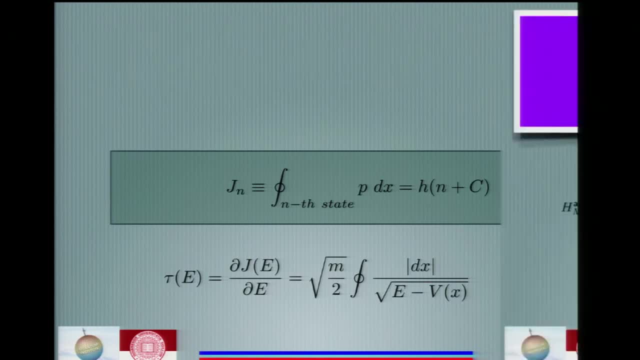 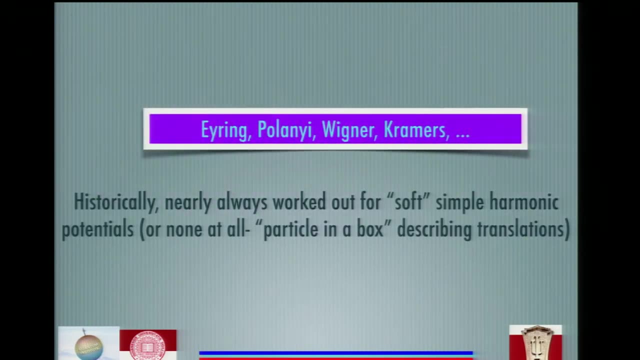 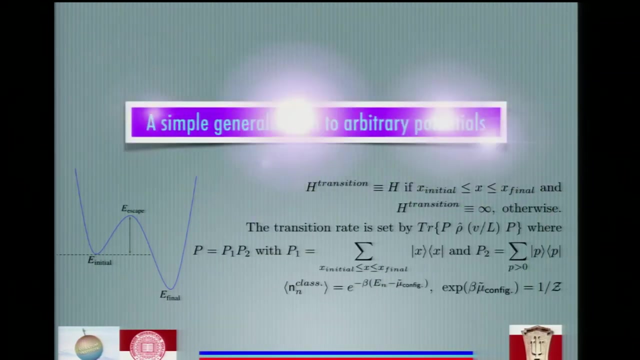 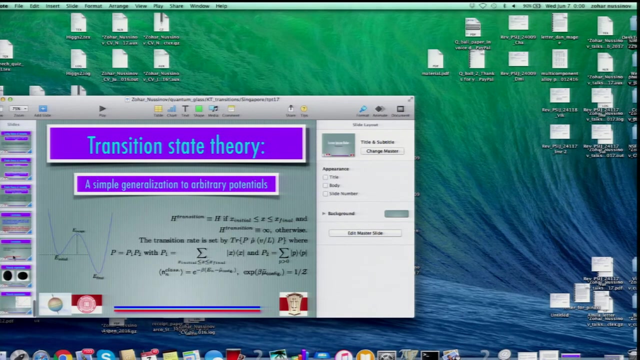 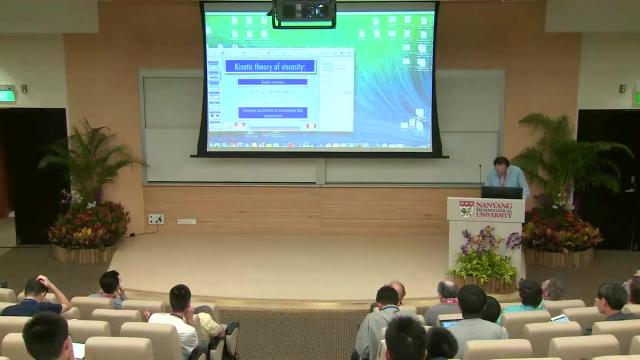 doing this so you can actually go to the other extreme and ask what happens at very high temperatures, and there, of course, typically became they have an activated behavior. what you find is that- I apologize- what you find is that the pre factor that you have seems to be. 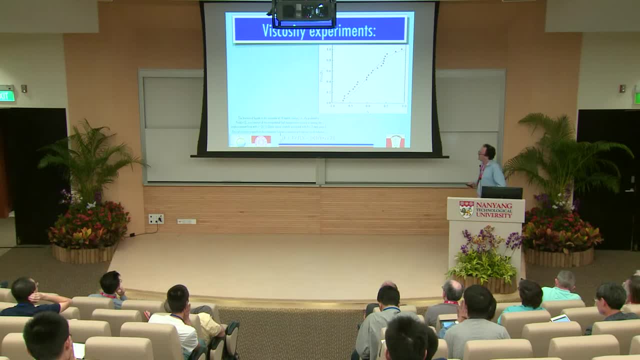 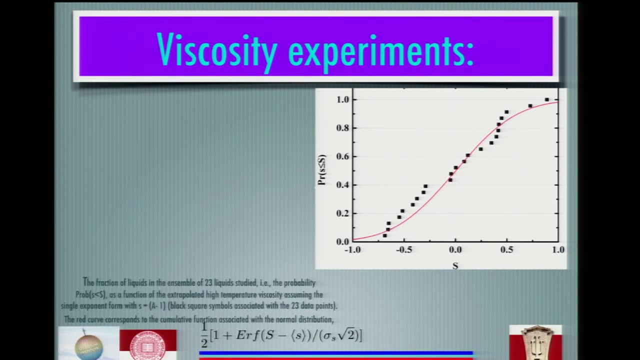 nothing else but the number, density of how many items you have for your volume times Planck's constant. so units of viscosity, as is well known, are equal to Planck's constant times Planck's constant. so units of viscosity, as is well known, are equal to Planck's constant times Planck's constant. 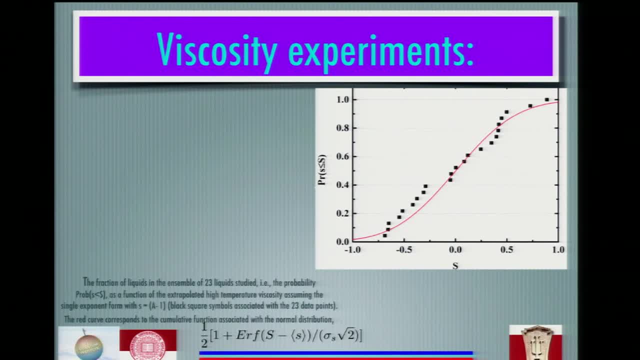 times the number, density, one of her volume, and it seems to be that if you try to fit the viscosity to the ring, this form, the pre factor is nothing but just as this average, this product of n times H, remember it. and if you try to look at that, but rather than themselves and ask how much do you? 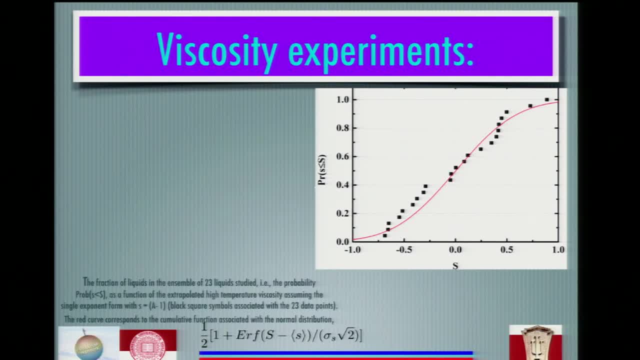 deviate from that. for deviations and this is the reserve deviations from this raw value we might expect by an average. it seems to cancel. so an average. this pre factor is pretty close to one. so this is basically about zero point six percent systems that we looked at. 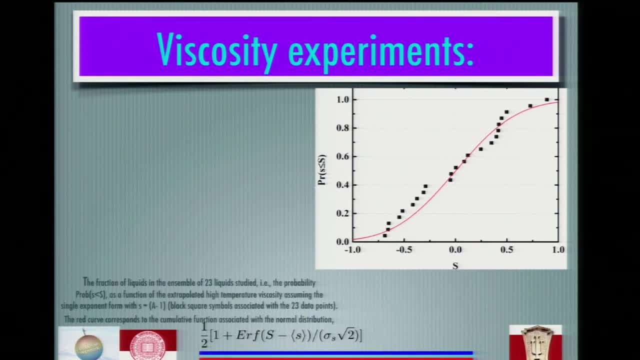 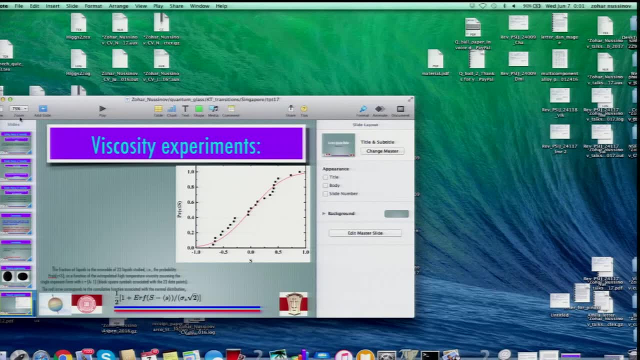 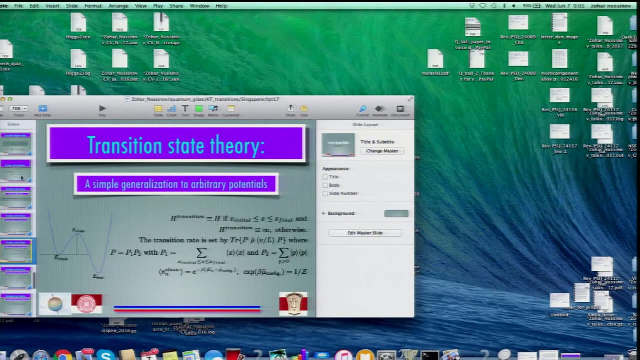 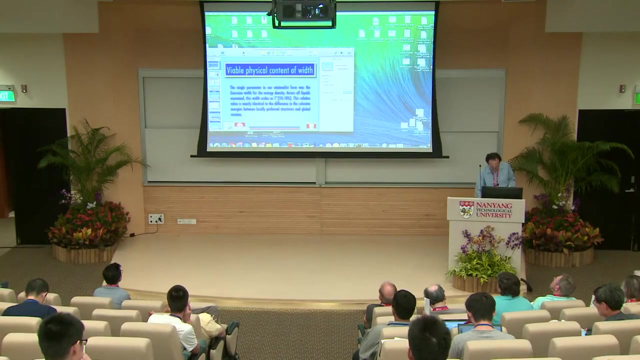 and the reasons for that might be reasons for this, but I don't have time to go over that. so, anyway, let me just tell you back, let me just go. I thought it was talking. I am NOT getting it in a good way. I was a serious for this. but let me just go back to what the conclusion like, my conclusions. 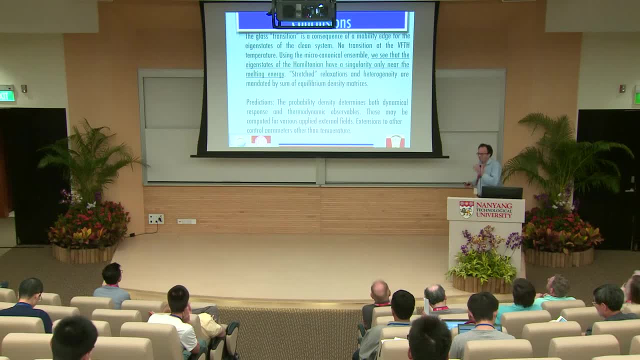 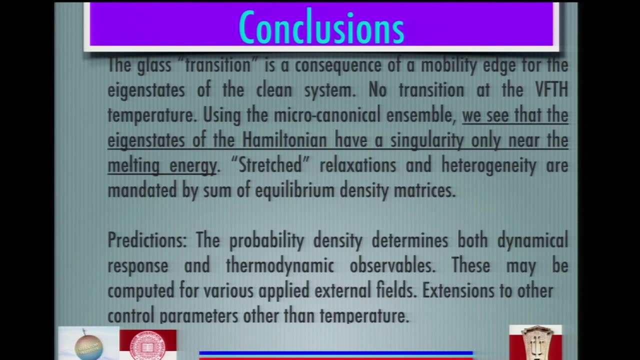 so the basic punch line I wanted to tell you is that this transition, even though it seems to be very, very different, might actually be a conventional transition in disguise. okay, just because you just smear it out of her distribution, that's it. so it's a minimal change for what we usually know. 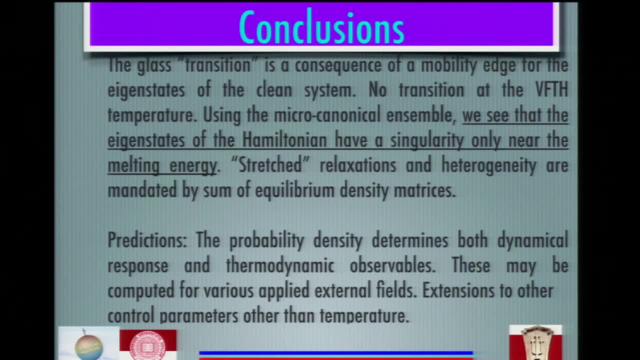 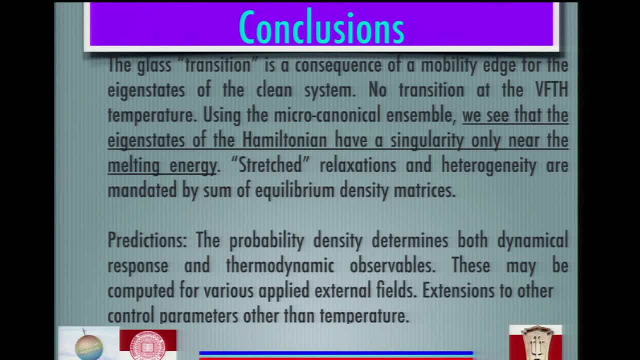 above melting to below melting. that's manifest. anything you actually would expand in terms of eigenstates, including what you have for glossy system and how you can actually test this. so here I just showed you what happens for the viscosity and that could grace the fixation data. but you can of course out ask yourself: or the same distribution of scouts distribution. 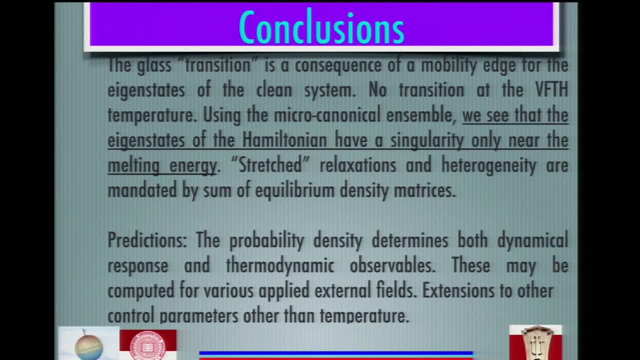 actually can describe everything. so there's only one parameter, this, which was Gaussian. can you predict all data using only one parameter? what you have for all fluids that we haven't done partially, because it's very difficult to predict all the data that you have for all fluids that we haven't. 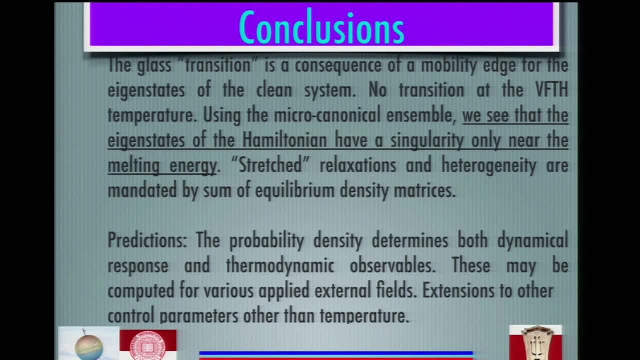 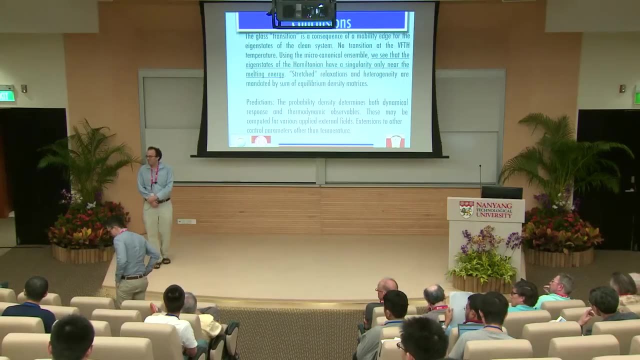 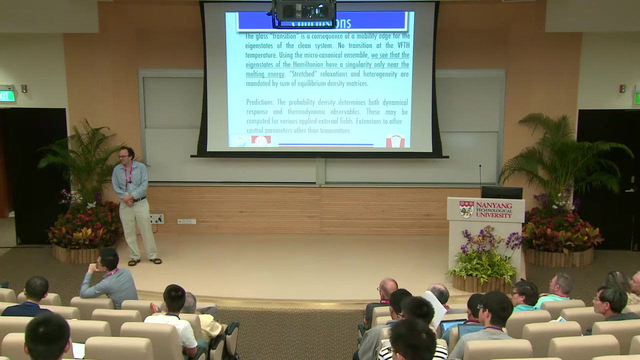 done so it's pretty hard to compare it to various things, but that's the best. basically, but upstairs, okay, two quick questions. the first one is what, if you can sort of velocity, if you calculate something like an order parameter, then the states we, dominated by the states that have- lower energy than your, than your market that privileges were looking for. when you have an order, and when you as well, that could mean that we could have an order parameter, then the states will be dominated by the states that have lower energy than your. that your market emissaries, you're trying to. 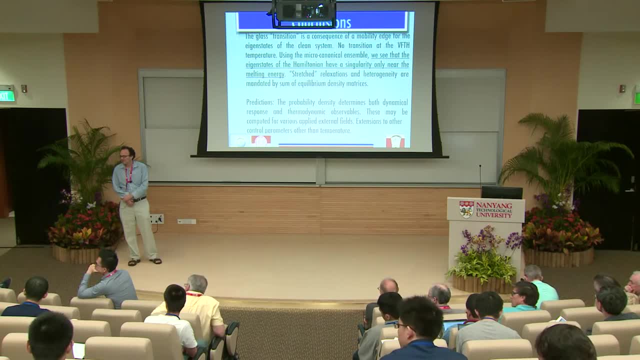 make. so how are things better than normal energy? and that's very interesting, the property of my cosmetics melting temperature, and then you might get some kind of order parameter in your calculation. that's not present in the in the glass, so can you comment on that? the second one is sorry, I forgot my second question, if I think about it, okay. 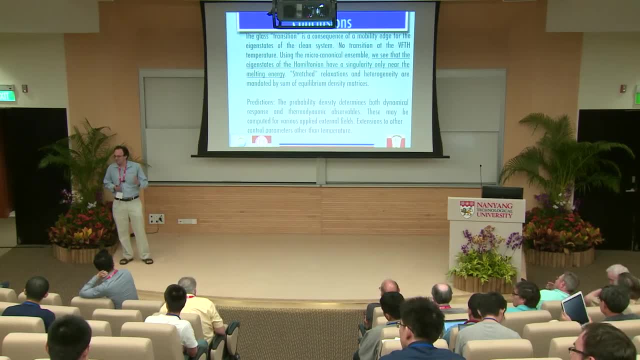 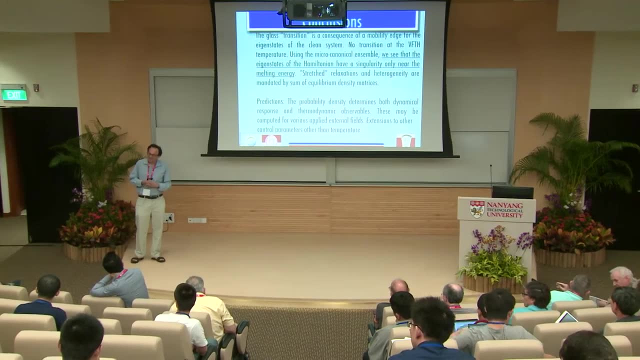 so you're asking: why is it not a crystal? so yeah, you're asking, basically, if I have a distribution which actually has crystalline states, why is it not a crystal? which might seem like a paradox? so it's not a paradox. and in the following way: so suppose I look at any, any system like any state I want to. 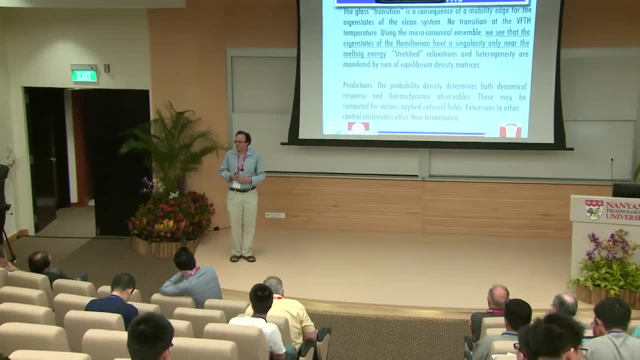 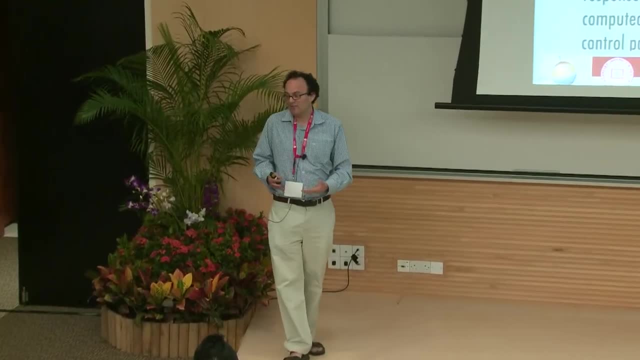 think about, I can always expand that state in a complete set of eigenstates. so, whatever it's a morpher state, but it's a low energy, I can always expand. it could be eigenbasis. and if only states are around, if low energies are, votes of a. 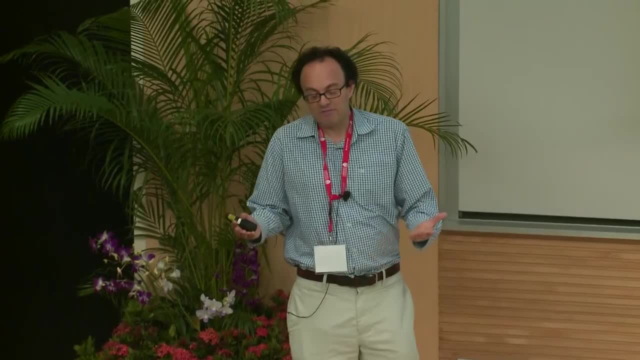 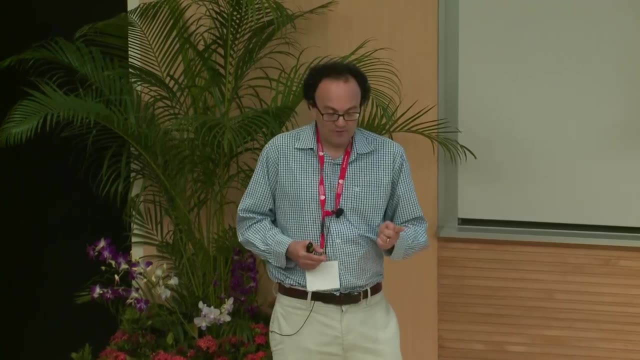 crystal. there's not. there's no way around it. they never. alternative differences suppose I have. I have different crystals with different wave numbers, Q, so I have different black peaks that I have associated. but now suppose you superpose many, many states having it, Q is at different angles. the result: this thing will not be. 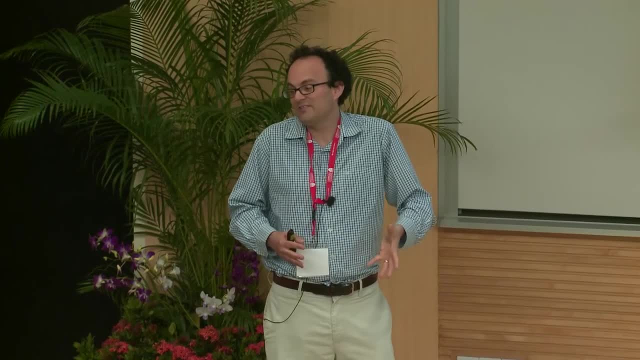 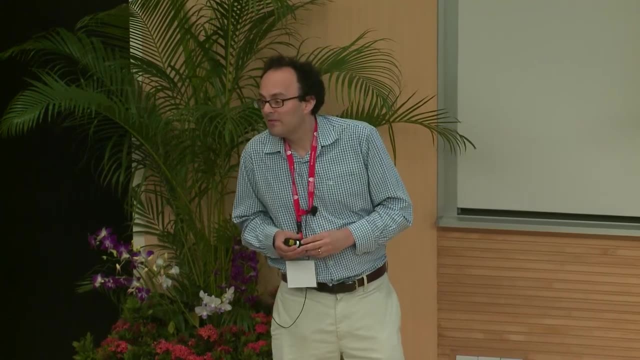 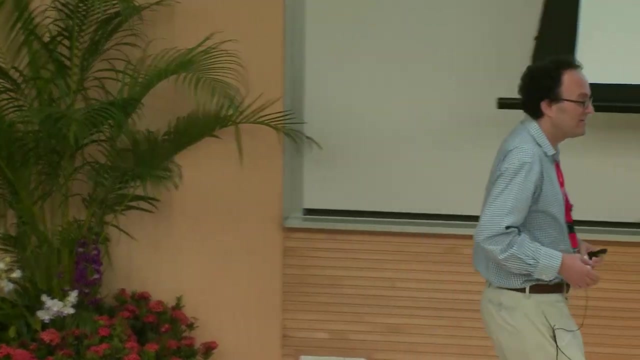 necessarily ordered because you just superposed it. the very aptitude actually just get mixed. you see what I'm trying to say, okay, okay, the rare events are here. the rare events are just if I go to this cartoon I showed you earlier. so it's a very good question. I thought I didn't say what you asked at the beginning, so 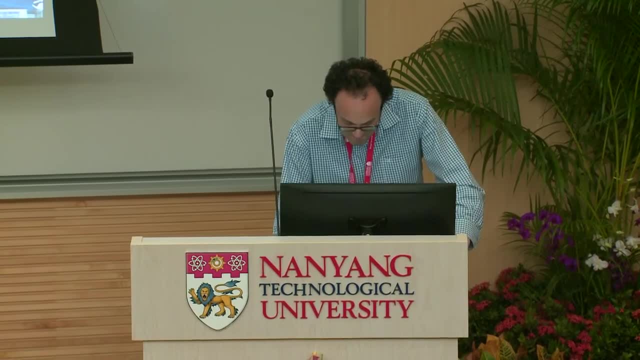 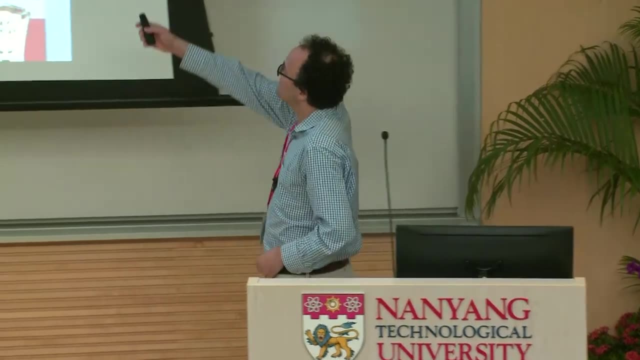 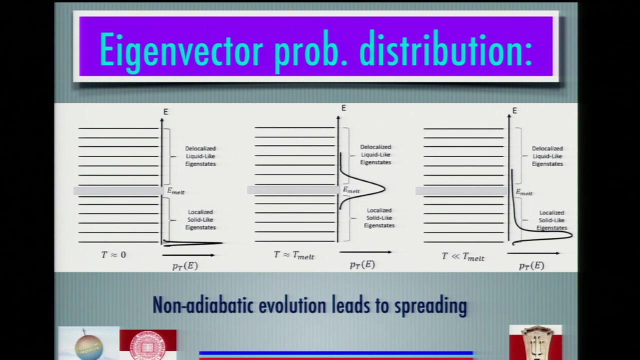 if I go here, sorry, not here here, so let me bring it to the table now. so here's a contribution of low energies. so here's my distribution of low energies temperatures. so now you can see most of this weight corresponds to a solid type eigenstates. but you see it. 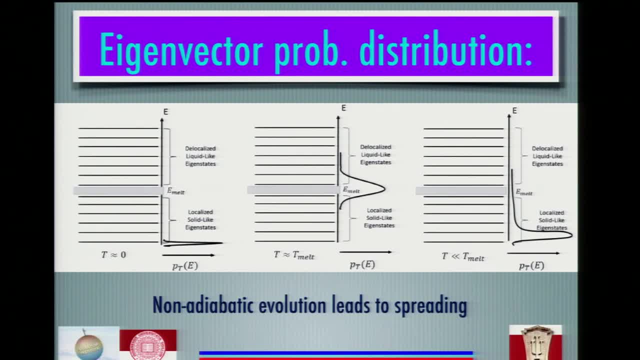 has a tail above melting and that tail is a narrow, but it's not zero because it's overall. this tail is very, very narrow. the probability of being here is very low, so these are rare events, so it's very unlikely that you actually have energy above melting, but once in awhile does happen that it does happen. 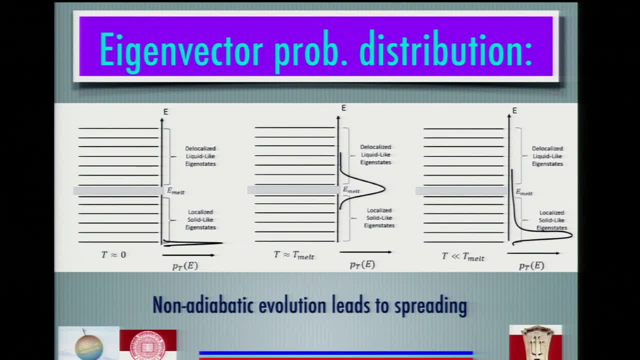 And that was an enables flow. So in the fluid type states we have flow. In the solid type states we have no flow. It's very rarely we actually have this, but we do have it and that's why we have flow. 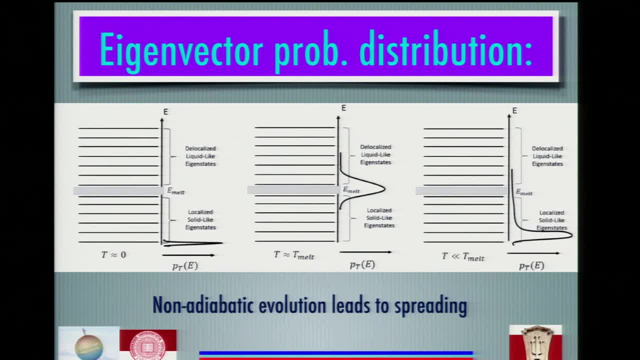 So the picture really is: as I go down in temperature or energy density, this thing goes down. this weight goes down. As a result, it becomes more static because the probability of motion, it just goes down. There's no singularity. 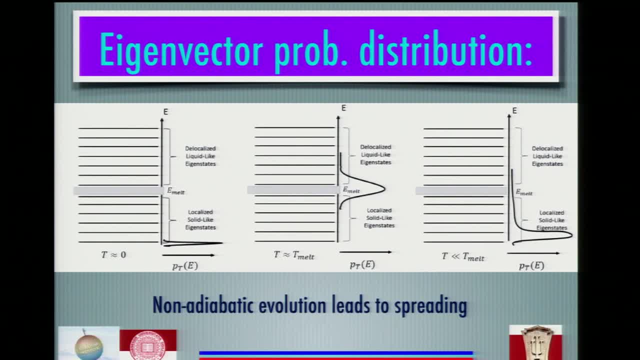 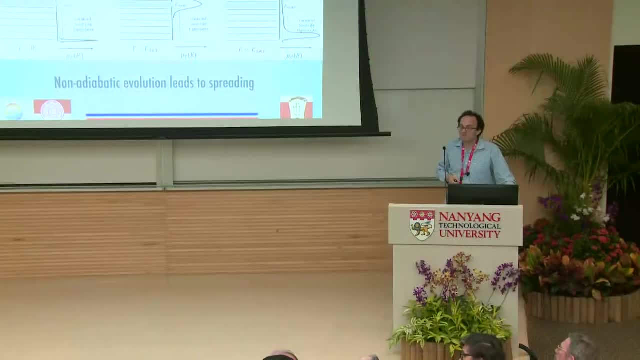 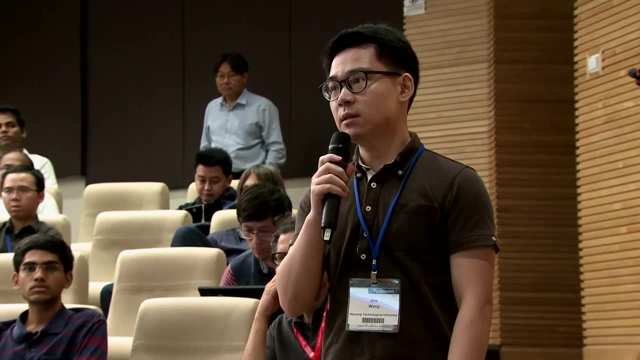 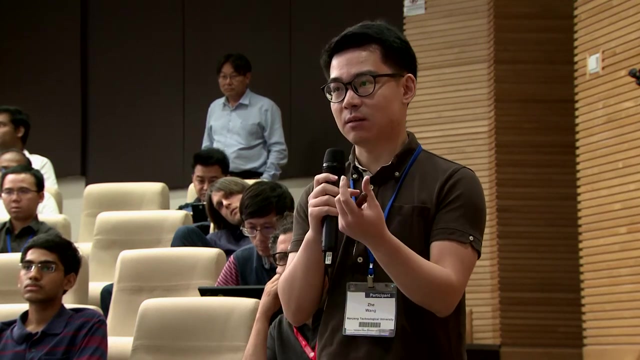 This whole thing is continuous, but it just drifts downwards and this tail becomes more and more narrow. Thanks, There's one slide called the viscosity experiments, that there is a white picture with a black dot and a red curve fitting. Would you be able to find that slide? 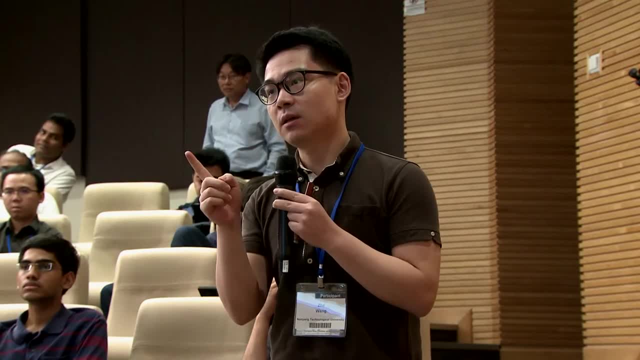 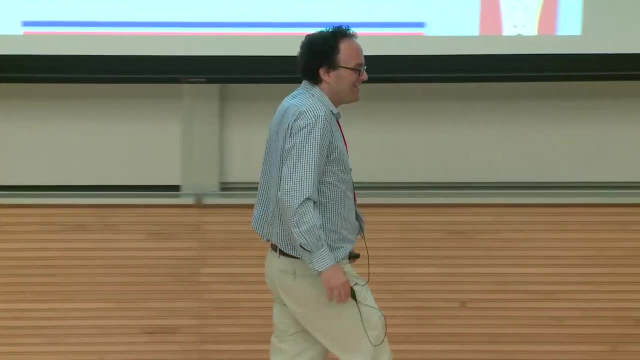 There's one slide titled viscosity experiment That shows one figure, Oh, but I didn't show one. Yes, yes, Yeah, okay, that's how we measure it. I'm not doing it, but my colleagues measure it, Yeah, so actually, the conventional way, as I told you, is to measure it with a sphere, using Stokes' law. 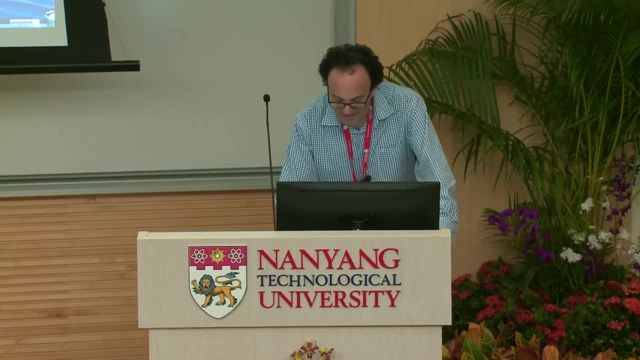 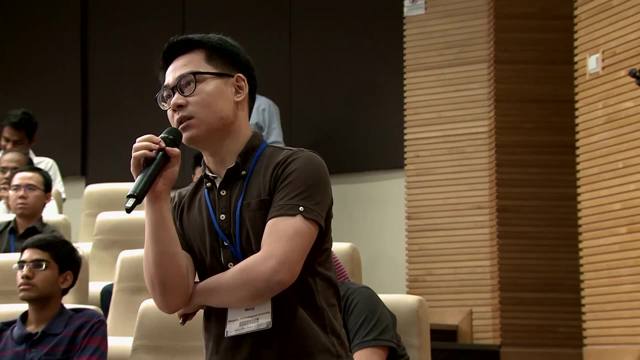 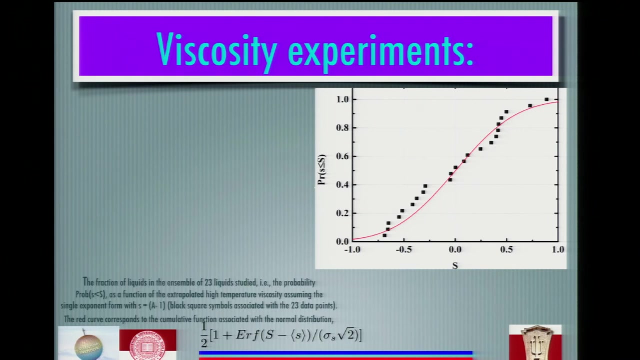 But of course this has been around for decades. Another way of measuring. it is actually like this. So what you do? This one, The next slide, The next slide With the red curve fitting This one. Oh yes, If you rotate the picture 90 degrees clockwise and if you have more data points, maybe you'll see the plateaus. 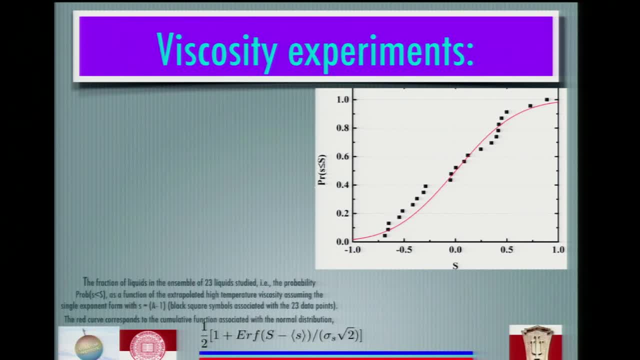 Maybe I'll see what: The plateaus, the steps, The plateaus. If you rotate the pictures 90 degrees, clockwise, Yes, And then if you have more data points, the most probably you'll see the plateaus, And these plateaus increase. follow the Farrow tree. 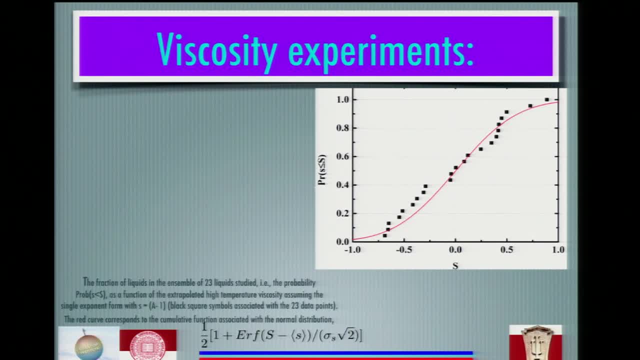 And this is called a devil's staircase. It's called what? Devil's staircase, Devil's staircase. Yeah, yeah, yeah, Oh, okay, Is this a? Oh okay, I'm sorry. Yeah, this is probably not devil's staircase. 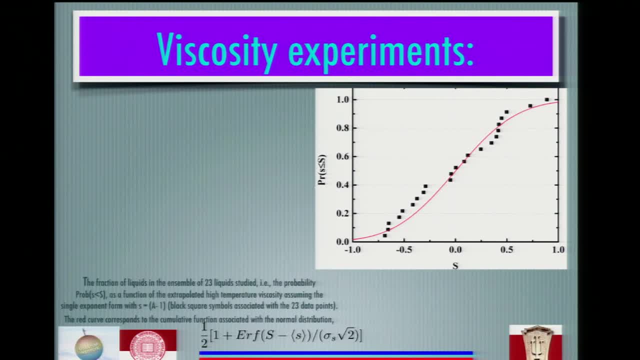 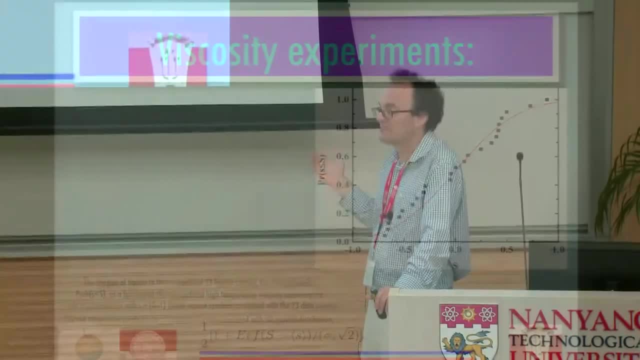 So, but it's a very good question. So of course you would like to know. these are all values that we have from my colleagues, have from their measurements, And we tried to fit the viscosity measurements to this simple expression from the theory to see how it works. 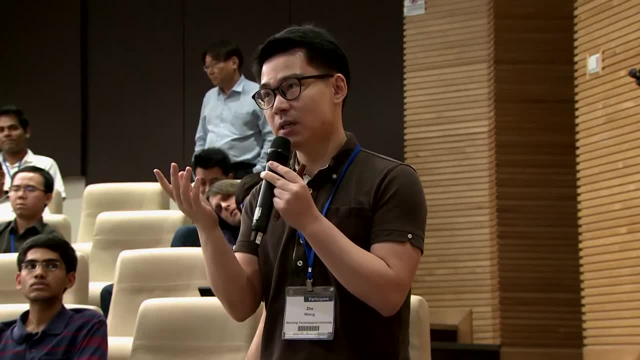 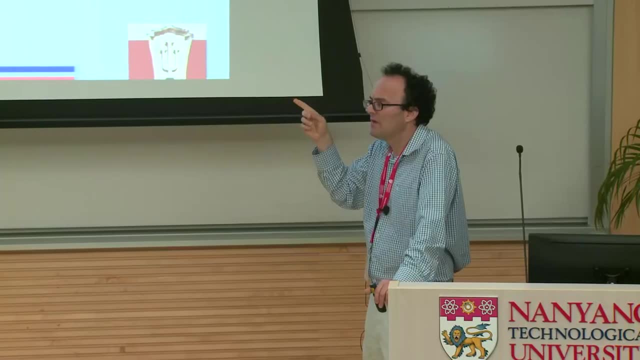 So I'm curious, I was just curious why this kind of a plateaus just come into presence in this kind of things, Why they present like this: Yes, and also they seem to me a fraction number, and then it's follow the devil's staircase. 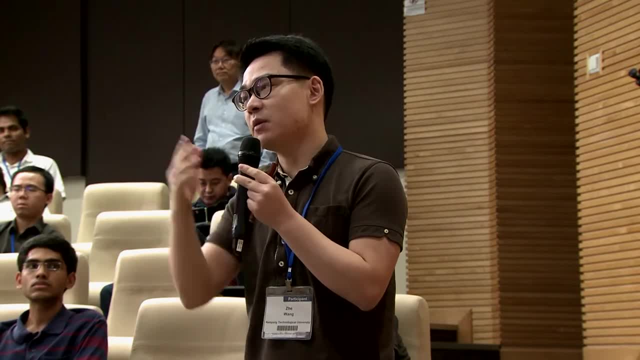 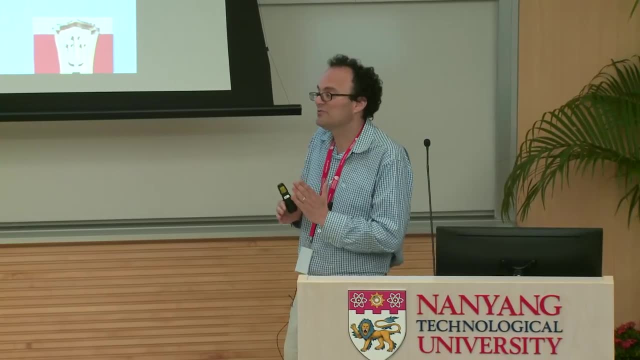 So if you measure the values Of this kind of things, then you'll find the fraction numbers Right, of course. So the problem really is, I mean, so you want to see if the number is close to one. The problem is the data set that you have is not very large. 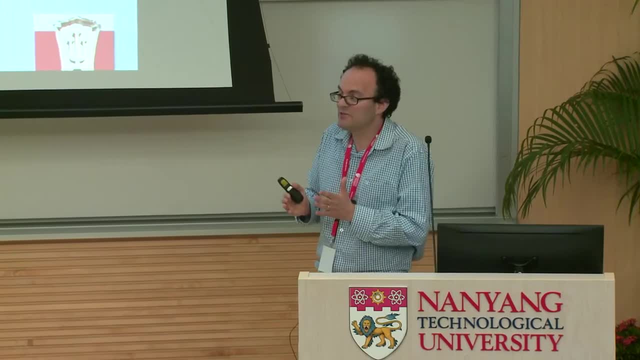 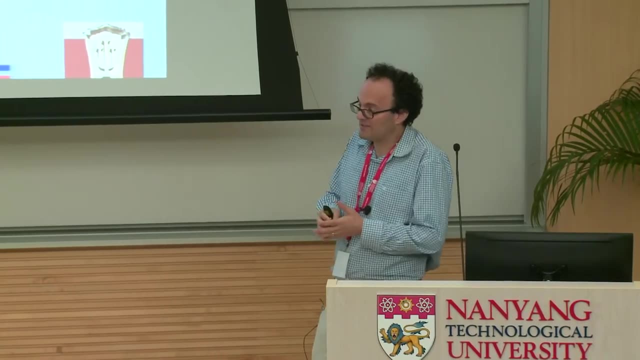 And here we have 23 different fluids. So if you do a histogram, it will be useless because you just have bars which are one or zero and it's hard to say. So what we do here is we wrote down the integral that you have of a probability- some of the probabilities- of being smaller than something. 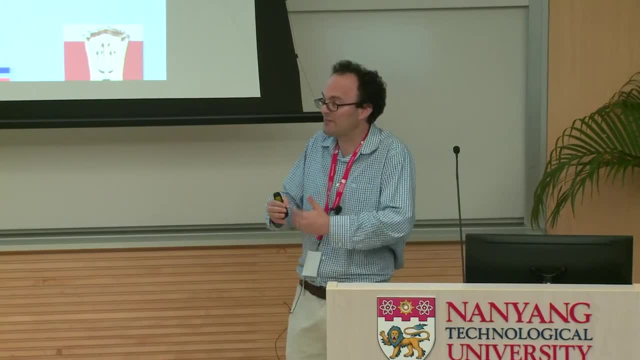 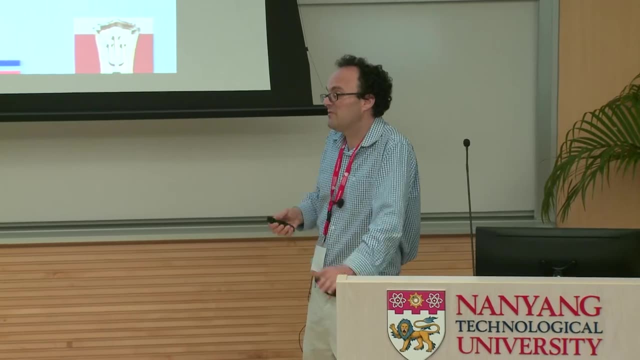 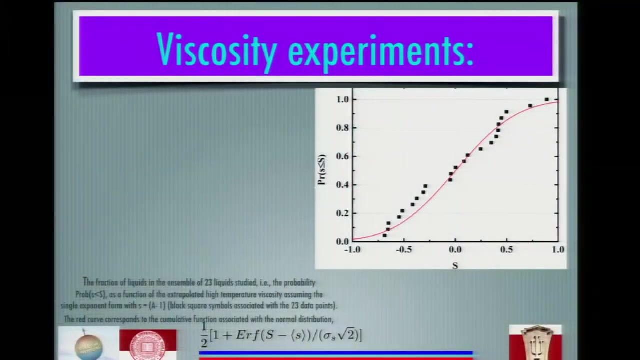 Okay, So now it becomes continuous. So instead of a histogram now you just spin some histogram So it becomes more continuous. And now you see, if you have a Gaussian distribution, what it would actually be. So if you have a Gaussian distribution of overall average value, where you have a zero relative to what you expect, what you actually get, 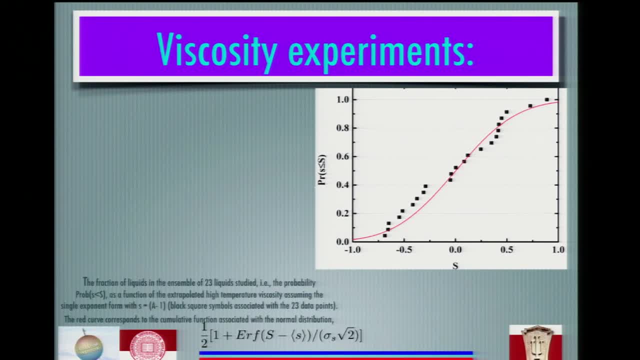 So this red curve is what you have if you just use the variance that you actually measure from the raw data And you see right down with the corresponding normal distribution and you integrate to find the error function And compare it to actually the probability from the different data points that you actually have. 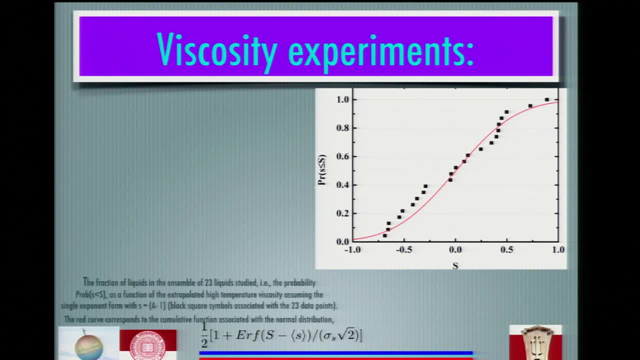 But overall the value of S is smaller than something. Okay, Ken, thanks, I'm not sure you've answered the question. Yeah, so the problem is there's not enough data to actually do. If you just do a histogram, it would be useless because you just have a bunch of steps. 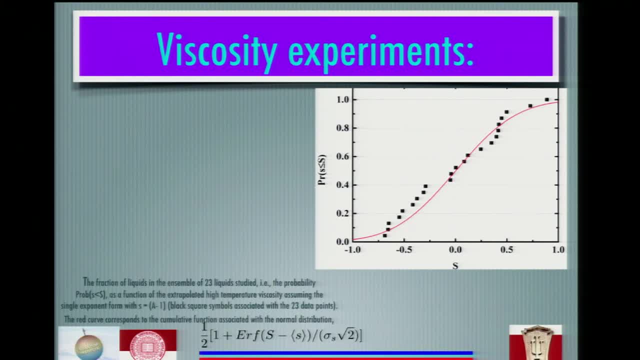 So you just sum it up, Okay. So you ask: in what fraction of instances is a pre-factor smaller than something? And that's what we've done here, Okay, thanks?